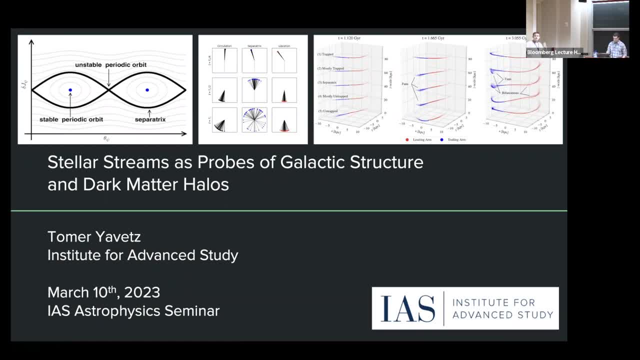 John McGoran at Oxford and I was introduced to the Lidov-Kozai mechanism via a paper that Scott wrote with Toma back at Princeton on why do Earth's satellites stay off. He realized that that was his real purpose in life. So he came back to Columbia and he did half of his PhD on. 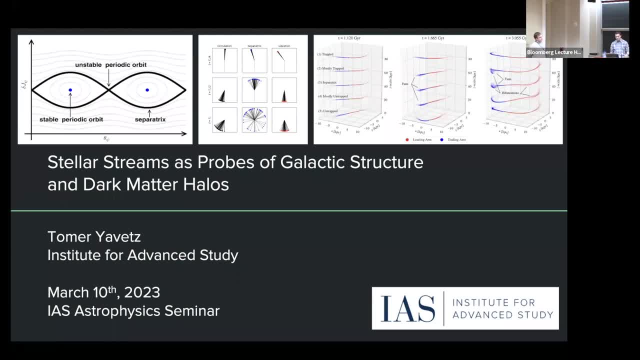 quasi-dark matter with Lambui and the other half, which is a half, I think we're going to hear about today on stellar streams and probes over the dark matter potential in our own galaxy. So take it away. Thank you very much. I hope my ghost doesn't haunt you too much. 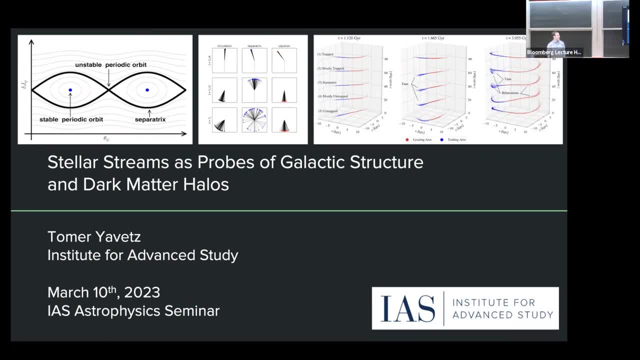 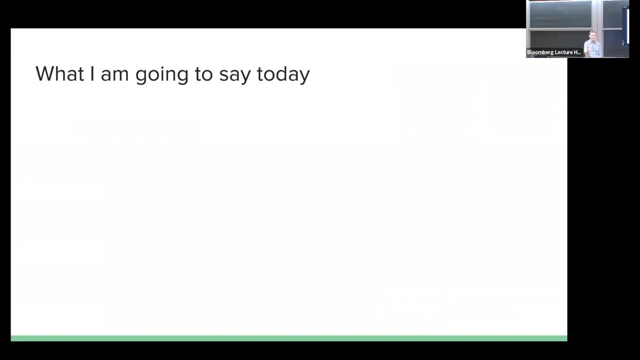 Thank you, Chris. Thank you all for coming. I'm excited to talk today about stellar streams as probes of galactic structure and dark matter halos. I'll just dive right into it, Okay, so what I'm going to tell you today? I'm told that it's good to tell people in advance what 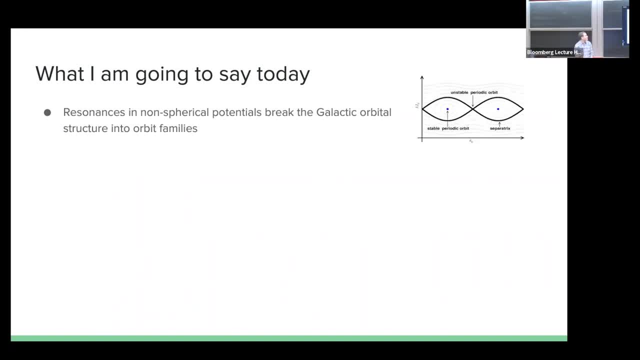 to expect, so that if you don't like this slide, you can leave. right now I will try to explain that resonances in non-spherical halos break up the galactic orbital structure into orbit families- kind of a brief, theoretical, initial part of this talk. I'll then explain that stellar streams 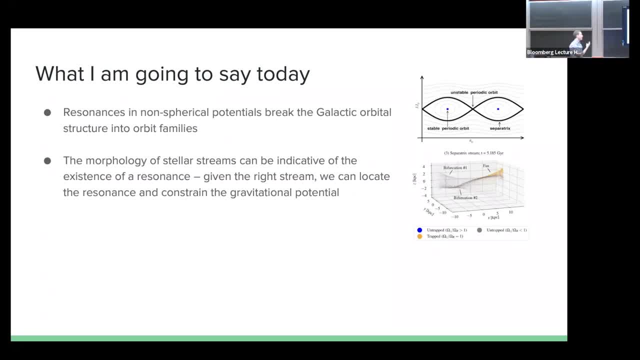 if you look at their morphology, you can in theory detect the location of the existence and the location of these resonances And then, using that, you can constrain the shape and the characteristics of the galactic potential. And then, finally, if I have enough time, at the end, 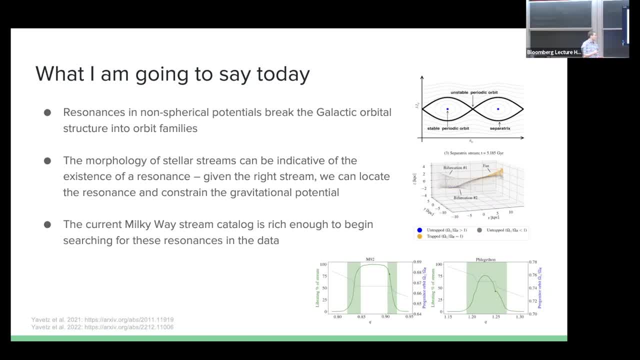 I might use the last few minutes to talk about how you can see the galactic potential of the galactic potential. Today's Milky Way stellar stream catalog is beginning to be rich enough to actually probe these things. I might even mention streams in other galaxies if I get there, but that is the 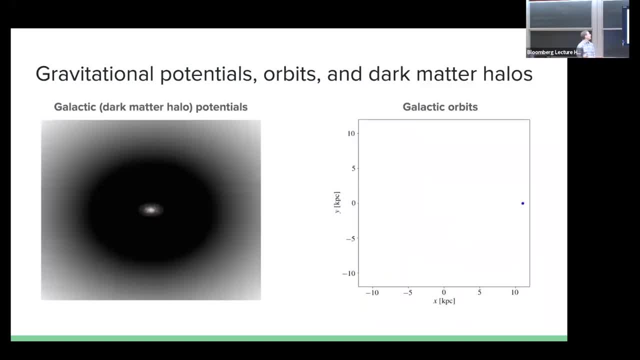 general overview of what I'd like to talk to you today. To start things out, I think it's always good to anchor this in what I think my job is as a galactic dynamicist, And one of the main elements of my job is connecting between gravitational potentials and orbit families. 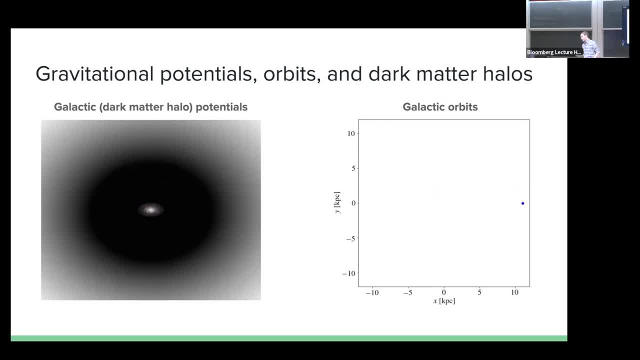 So here's the galaxy. it's surrounded by a big dark matter halo thing. If you were to know what that dark matter halo is, or if you had some other way of figuring out exactly what is the potential, you can integrate an orbit in this galaxy and you can figure out exactly what any star should do. 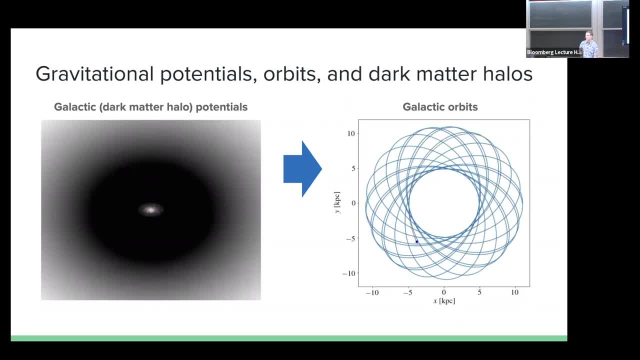 And this is a typical galactic orbit and what we think is a typical galactic potential, And so this is nice. You can also go the other way. If you know what the orbit is, if you see the orbit kind of evolving in the sky, you can then integrate it into the galaxy, And so that's what I'm going to. 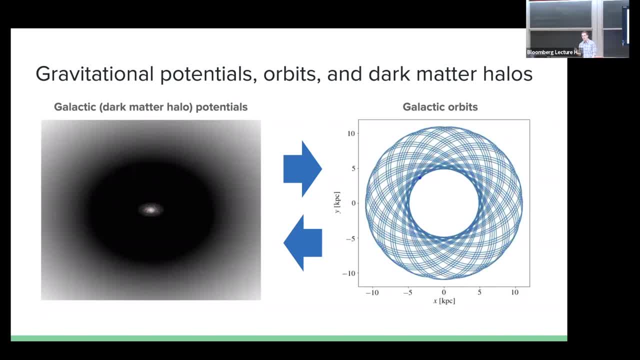 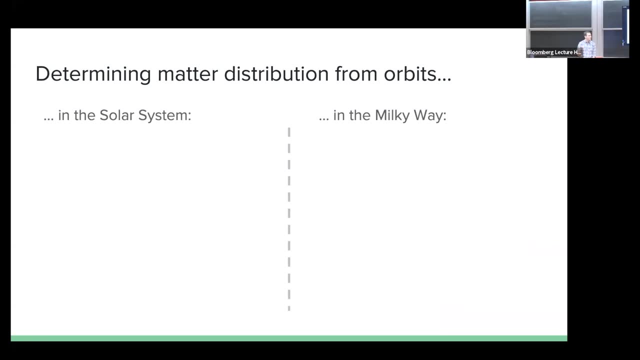 talk about today. You can then infer what must the potential be in order to host or to support such an orbit. You can't, maybe you can't get it exactly, but you can certainly constrain the shape of the potential based on what you see the orbit doing. This is not a new thing. People have been 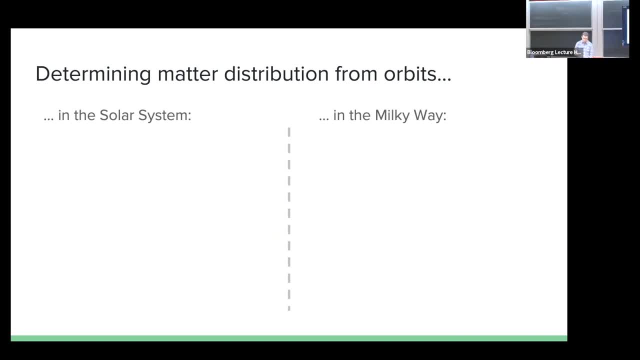 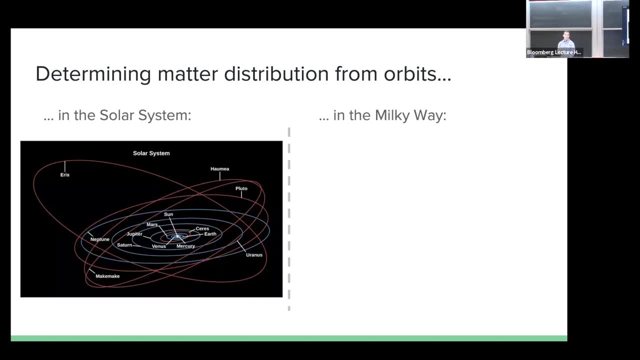 doing this. astronomers have been using this to study the solar system for centuries. This talk almost worked out perfect in terms of timing. In three days, it will be the 247th anniversary of the discovery of Uranus, or the discovery of Uranus as a planet that is orbiting. 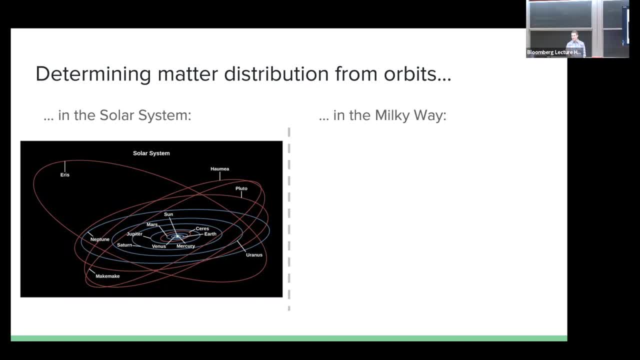 the sun. Interestingly, about 65 years later the next planet, Neptune, was discovered. And the reason it was discovered 65 years after the discovery of Uranus? because it took astronomers about 65 years to observe almost a complete orbit of Uranus. to see that that orbit isn't in line. 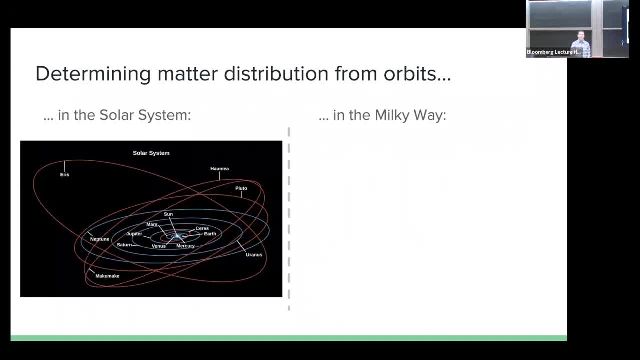 with the existing mass distribution that was known at the time. They figured out there must be something else tugging at Uranus to perturb it from that expected orbit. They figured out where they thought it should be, They turned their telescopes there. 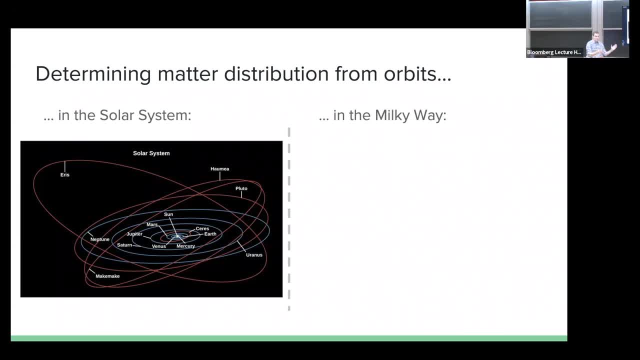 and lo and behold, there was Neptune. So, bottom line, you see orbits, you can infer the mass distribution, in this case mass distribution of planets in the solar system. And so we want to play a similar game in the Milky Way. The problem, or one of the problems, that we face with the Milky 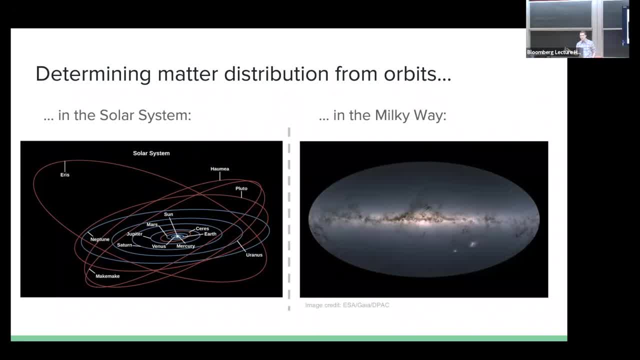 Way is that, unlike the solar system, where we can sit and observe over many nights and see these orbits in the Milky Way, the longer you sit, the more you'll just see the same picture: The middle. you know the timescales involved. here are millions of years, A typical star. 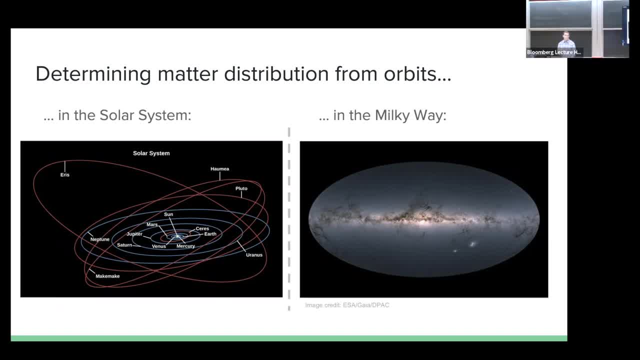 the solar radius of the sun, for example, will orbit the Milky Way once every 200,, 250 or so million years. So it's not like you can actually sit and watch and expect to see Uranus orbit once around and figure out what is the potential that is inducing that orbit. So we have a snapshot. 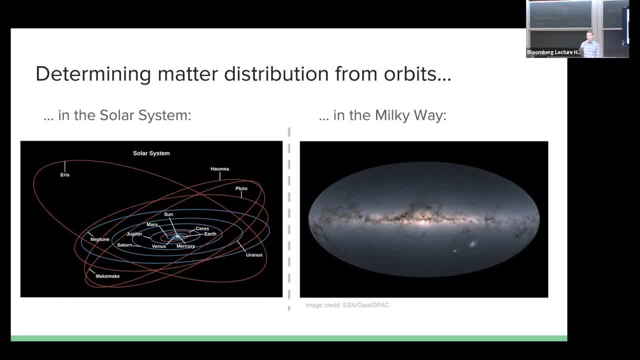 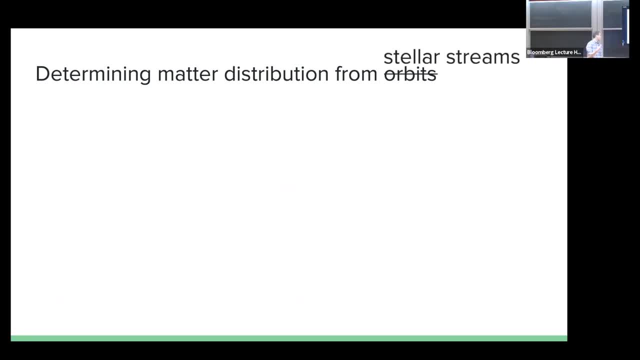 What can we do with a snapshot? How can we use a snapshot To infer or determine the mass distribution? how do we see an orbit in a snapshot? And so one of the tools that we have come to use over the past few decades is this thing called. 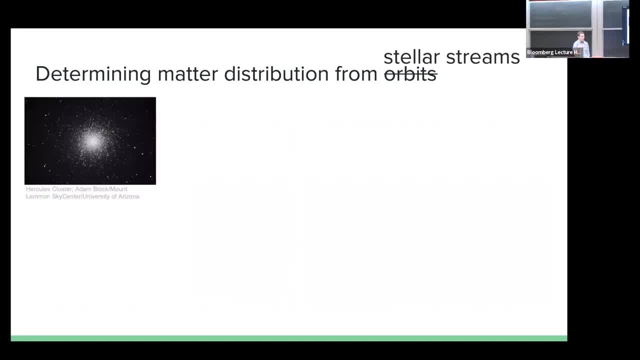 stellar streams. Stellar streams are the product of when a small object like a globular cluster or dwarf galaxy, falls into a bigger object, like a galaxy, like the Milky Way, and gets tidally destroyed, tidally stripped as it is falling in. or maybe it's formed in the Milky Way and is 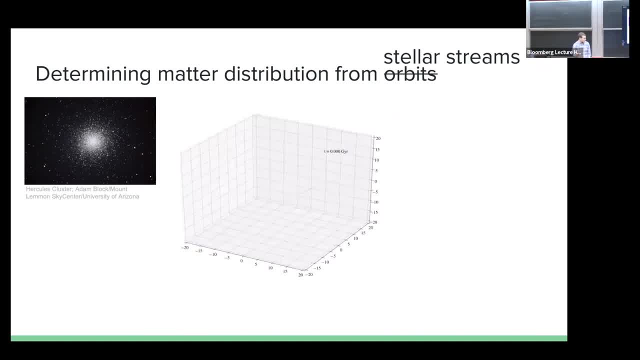 tidally stripped as it evolves, And you can actually model this, simulate this very easily with just test particles. That turns out to be a pretty accurate depiction of what's going on. What you're seeing here you can make out the little gray line That's the orbit of the 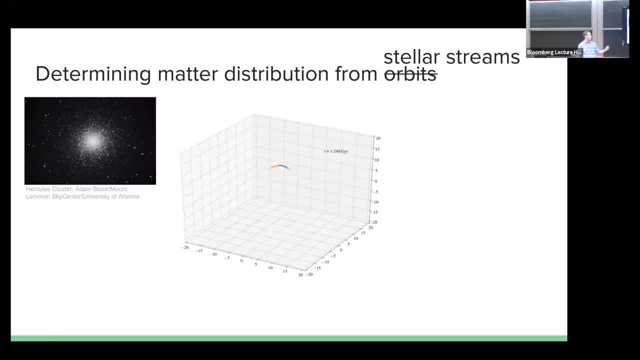 progenitor, And you can see that along that orbit you have a bunch of stars that are slowly spreading out as this thing evolves over time. Newer stars are really closer, but the stars that are initially stripped kind of spread out further. So that's a pretty accurate depiction of what's going on. 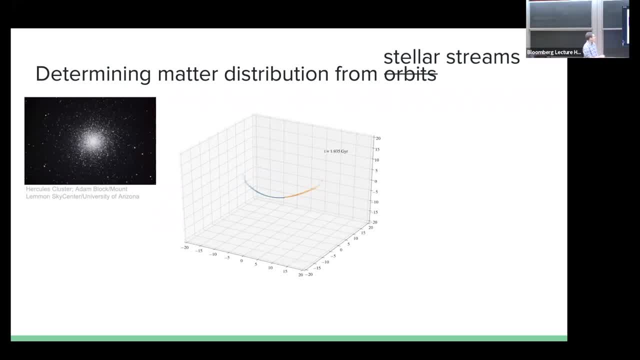 So you can see that there, along this progenitor orbit. I don't know if anybody can see the laser. You certainly can't see them. So anyway, so the bottom line at the end of this picture, you've got your orbit. that's more or less traced by the stars that have been stripped from the stream. So here, 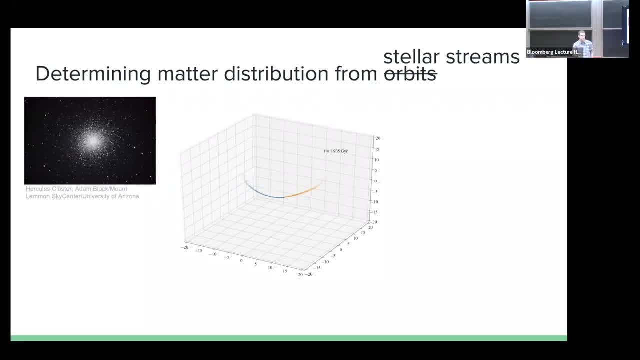 we have a snapshot and we've essentially found an orbit, which is pretty cool. It's not exactly an orbit- I can talk about that, but it's pretty close and you can do a pretty good job of figuring out what the orbit of the progenitor was. to have formed a stream. 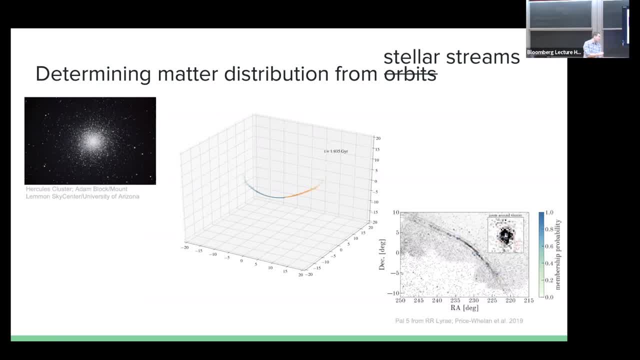 Along this track And we see these things. This is a picture of the Pallet 5 in actual data And our Lyrae stars again forming that long, thin filamentary structure. What Pallet 5 is one of the streams that we've known to exist for a while around the Milky Way. 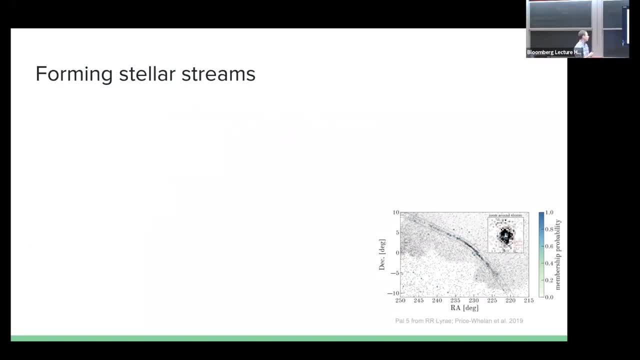 A little bit more of how you get the structure. One way that's, I think, very, very easy to understand kind of why you get a thin filamentary structure that you can see and observe, is if you convert to from phase space, from X and V position of velocity, to what we call action angle coordinates. 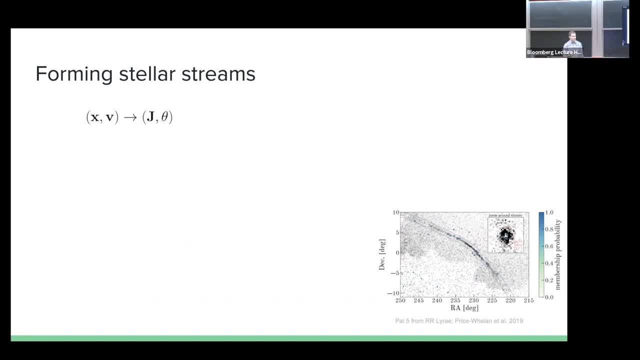 Generally, a lot of dynamics becomes a lot easier when you convert to actions and angles, because your actions are constant and your angles evolve linearly over time, And the frequency that governs the evolution of the angles is just the partial gradient you have with respect to the 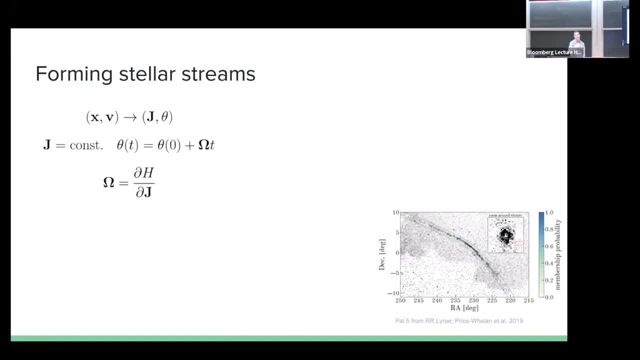 actions. So if you find these convenient coordinates, evolution in a potential becomes very easy To calculate because again you've got a set of coordinates that are constants and a set of coordinates that evolve linearly over time, And then you could project that back and figure out. 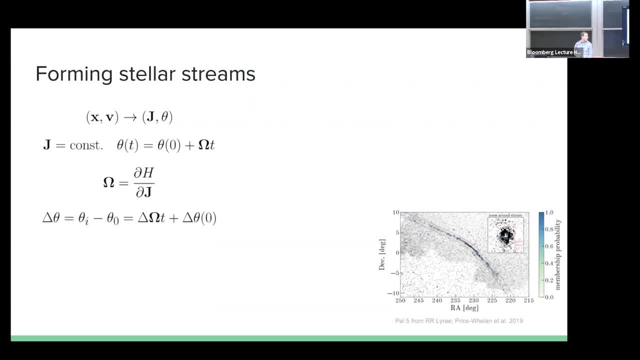 where your star is at any given moment. We can take this a step further and say, okay, we believe that our progenitor, our globular cluster, for this case, is leaking out stars and those stars are spreading out And the reason we see kind of this long filamentary structure or any kind of 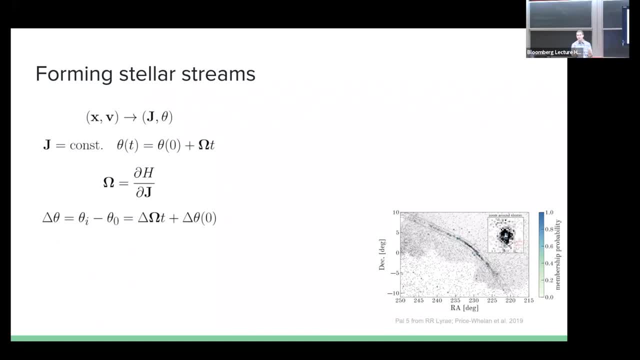 structure that we see must involve some delta angle, basically a change in where you are along the orbit to spread you out the way we saw these streams spreading out. So this delta theta is theta of the i-th particle that was leaked from the progenitor, minus the theta of the location of the progenitor, currently theta naught And that. 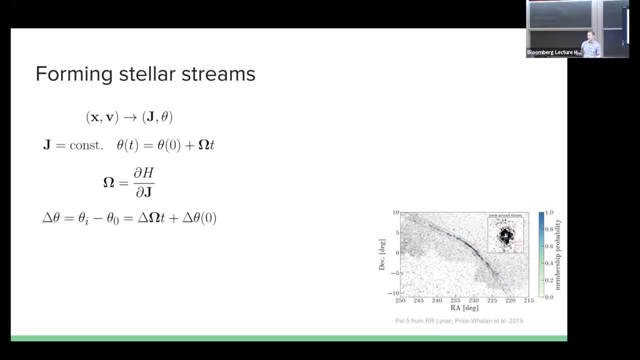 is just delta omega t plus whatever initial spread between angles you had. Now we had a long enough time. The initial spread in your angles you have when you leak the particles is insignificant compared to this delta omega t term, because that just goes with time And you can also well. 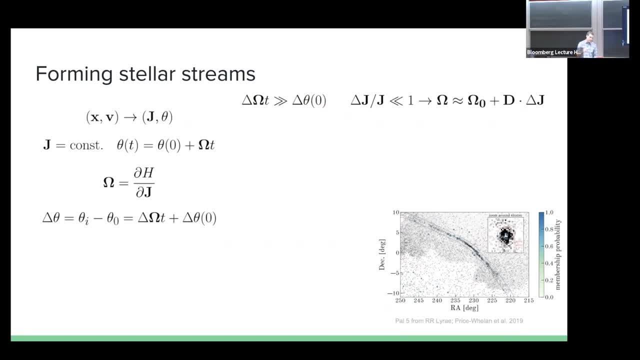 the assumption we typically make here is that your initial spread of actions, basically the spread of leaked particles from this progenitor object, is much smaller than the size of your galaxy or the scale of actions in this galaxy. And so you can, you, can, you end up being able to approximate. 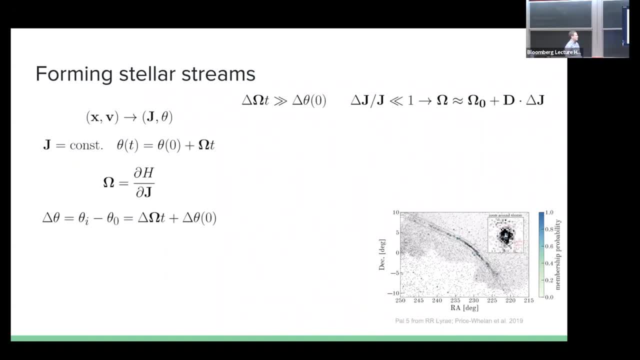 the frequency of any particle, any star that's been stripped from this using a basic Taylor expansion of the frequencies. This is the Hessian object, which gives you basically the second order term that lets you expand the frequencies And then you can write out your delta theta Again. 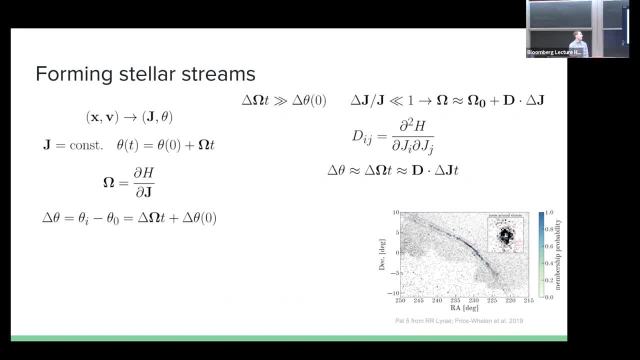 this is delta. theta is how spread out the stream is, as a function of this Hessian which then relates things back to the spread in action space to begin with. So if you know, do you have any way of prescribing or figuring out what is your spread of action? 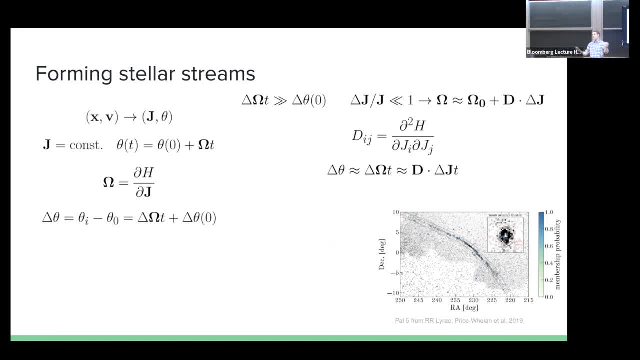 that delta J and you know what the Hamiltonian is, you can figure out what this stream or what any kind of configuration should look like. assuming these assumptions I made on top, It turns out- and you know this has to be the case- if you get long filamentary structures. 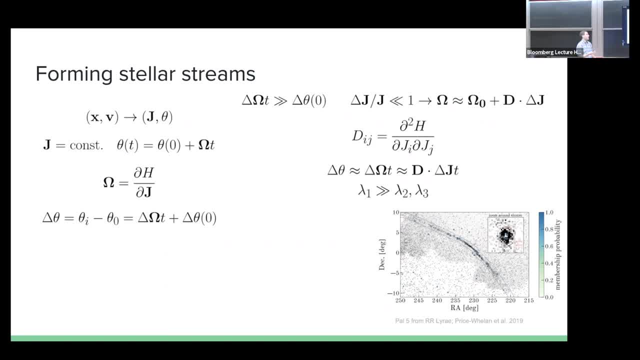 that are one dimensional, that this Hessian matrix has to have one dominant eigenvalue. If it wasn't one dominant eigenvalue, you wouldn't get a one dimensional structure, And so you can. then again, you can relate your spread in angles to this one. 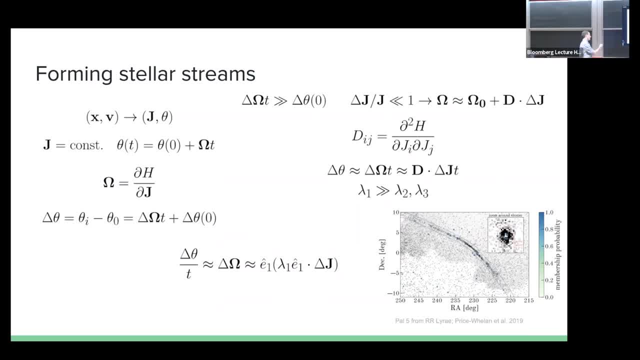 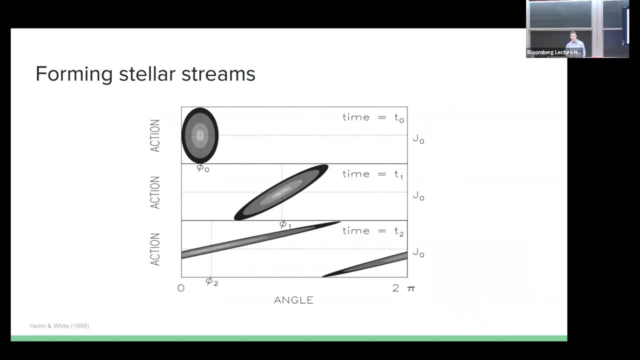 direction that's governed by the Hessian, related again to the spread in actions. To draw a picture of what is going on here and just go back to the paper from now, 20, 25 years ago- almost this is Helmian White, one of the more important papers on started this Russian. 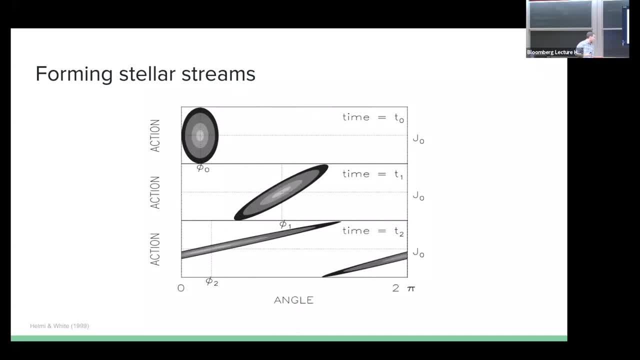 streams. There's a few others, One by my PhD advisor, Catherine, one by Scott, all kind of touching on similar aspects of this idea of forming the stream from a disrupting cluster in a galaxy. What are you seeing here? you're seeing this initial blob in action space up here, an action angle space, And, as you let, 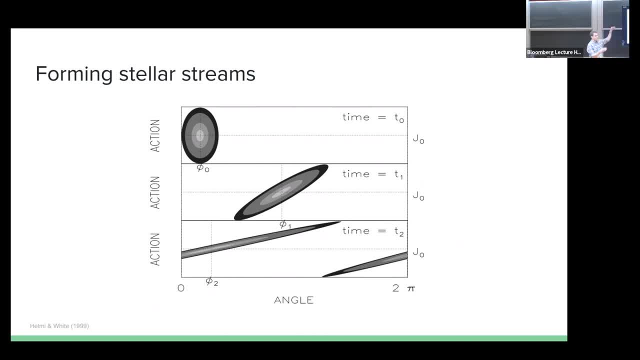 this thing evolve over time. your actions remain constant, So you're not changing anything vertically, but your angles are spreading out and they're spreading out at different frequencies. Again, this is your delta omega, And so over time you shear in an action angle space like this very kind of easy thing to 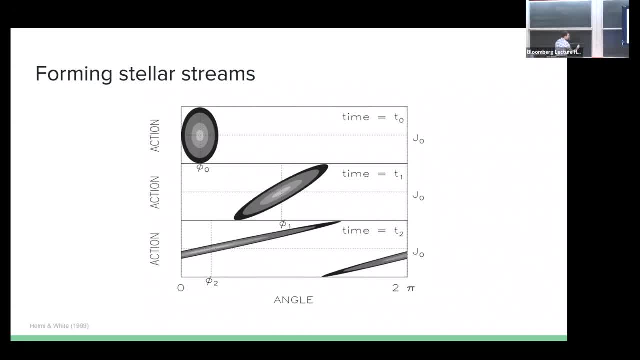 visualize The main thing I want to just draw here, because we want to come to this later. So you've got actions, you've got angles, your actions are constant, you're not changing actions, And Hamiltonian is small behavior, integral, integral and every particle just moving along. 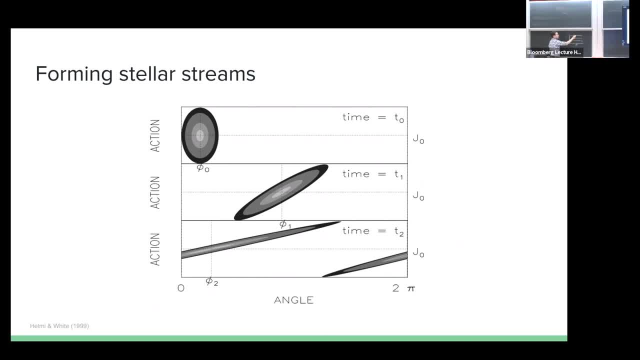 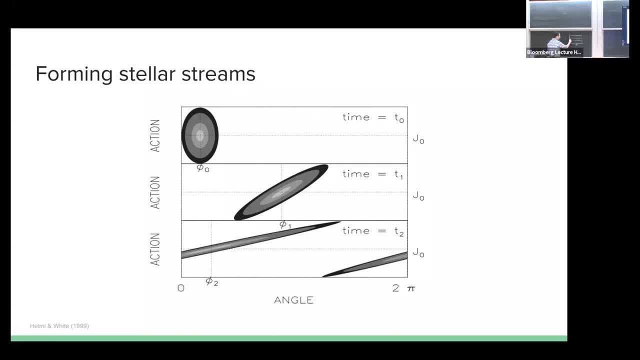 you're moving, but whatever is governed by these differences in frequencies. So if you start out with a line that lines slowly shears, that would choose either Very, very simple. That's how you get this nice, clean, one dimensional structure in the galaxy. 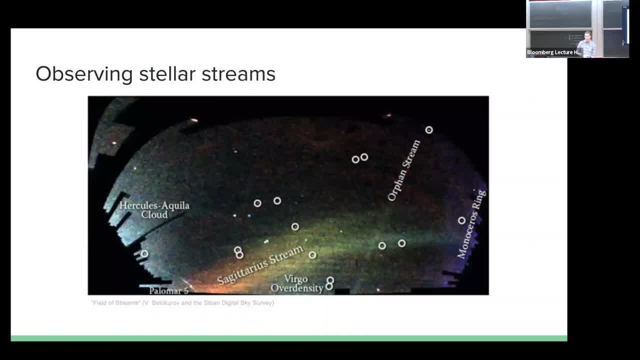 And we see these things, And we've seen these things for a while. This is a famous picture called The Field of Dreams. We've gotten much further since this. This is early 2000s, I think, or mid 2000s, And here all they've done is they've colored stars based on their distances. 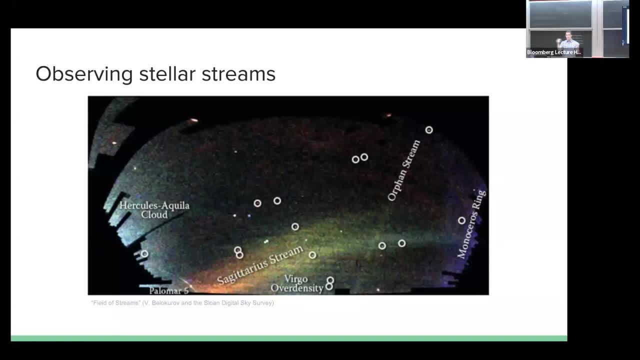 from us. you can see kind of as the gradient changes. you see these filamentary structures. So you see, this big kind of somewhat one-dimensional object is the Sagittarius stream. that's in the Boreth galaxy. You can see PAL-5, which I showed earlier, right down here. 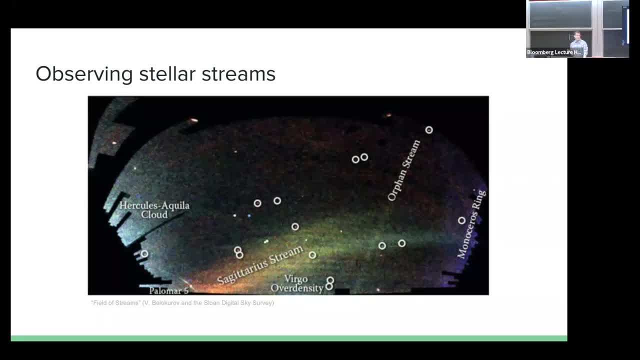 It's a cluster stream, So we see these objects in the Milky Way in actual data, which implies that these theories are in some way working and that these are our general assumption of progenitors spreading across orbits. There's at least something behind that that we can use to study the Milky Way and its potential. 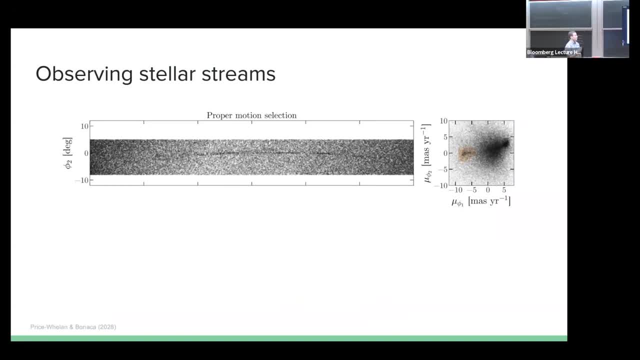 We can do better than the field of streams. You can certainly select for proper motion. So if you look at the plot all the way in the right you've just selected for co-moving stars. Stars are all moving in the same direction because, again, the stream is all moving along more or less. 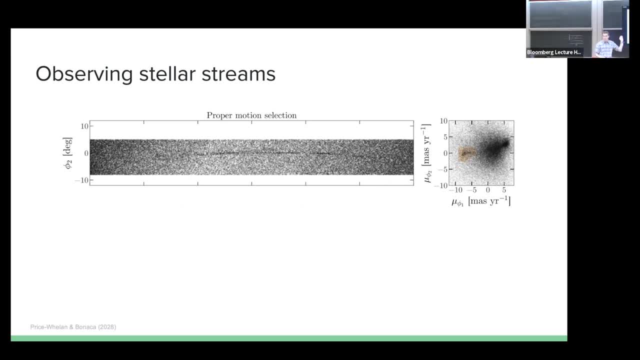 the same orbit. So if you select for that, you see cleaner pictures of streams. So here this is a stream called GD1. You see a nice long kind of thin filament. You can do even better than this if you go to photometry. 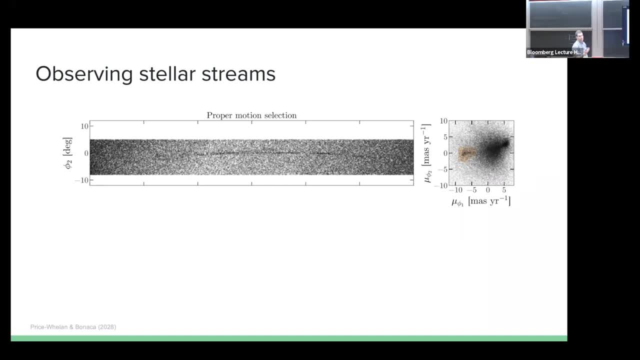 because, again, these streams are formed from an object, usually a globular cluster, in this case a globular cluster, Globular clusters. I won't say they have one population of stars, because that's an area of active debate, but they 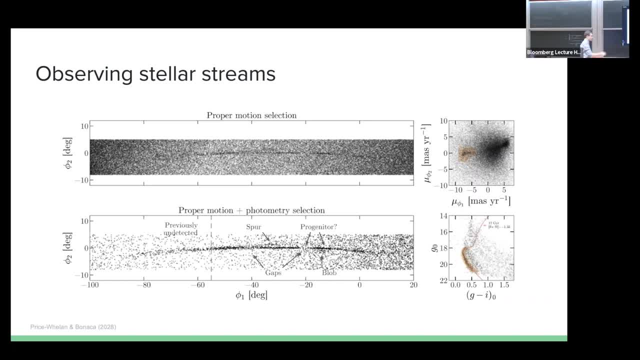 have a very cohesive population of stars. So you can pick out your track in an HR diagram or a color magnitude diagram and filter just for those stars and you get an even sharper picture of the stream than you did from just proper motion. So generally this is kind of the game. 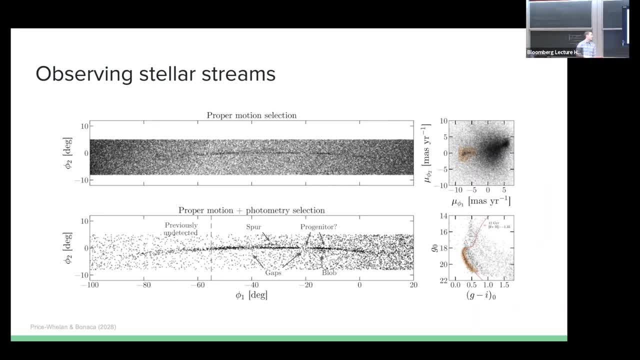 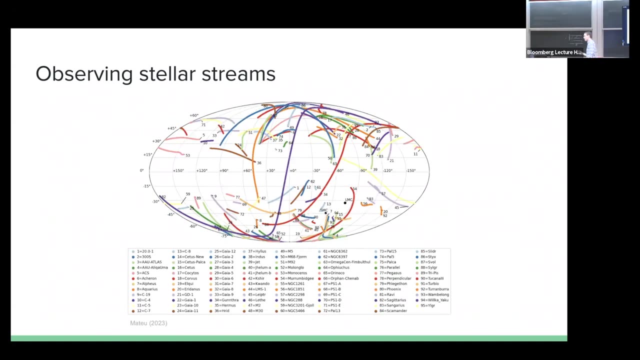 that observers nowadays play to find these streams in the data, And we see more and more of them with new surveys: Dark Energy Survey, Gaia, further iterations of SDSS. We now have a catalog of closing in on 100 stellar streams from dwarf galaxies and globular clusters in the Milky Way. 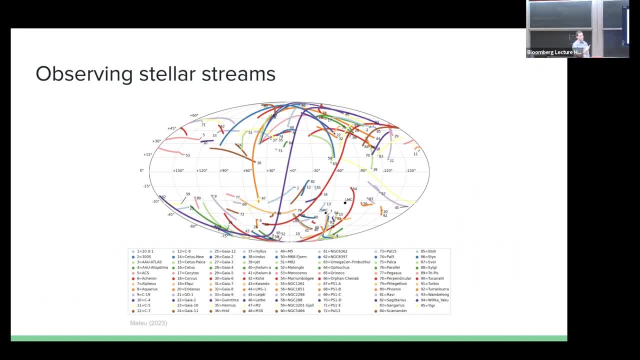 And so you all should be saying: all right, Tomer, this is the end of the talk. You've got a lot of orbits. You can figure out the potential. What's why are we still here? This should be it, and this should be it. 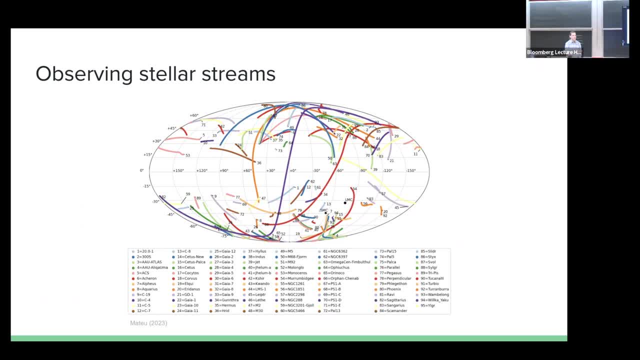 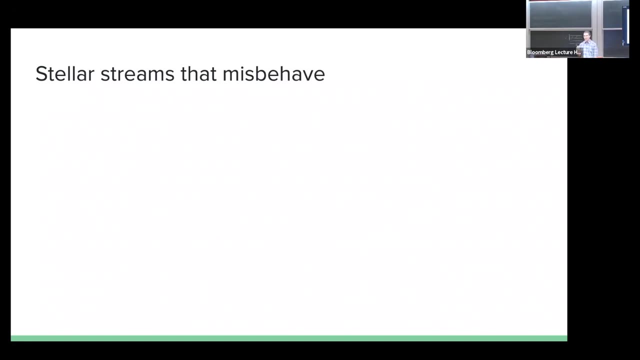 It turns out, we've discovered more streams. We've also discovered a whole lot more complications into modeling these streams and figuring out- inferring based on the streams and what we think their orbits are- what is the actual shape of the potential, And so I like to label this part of the talk. 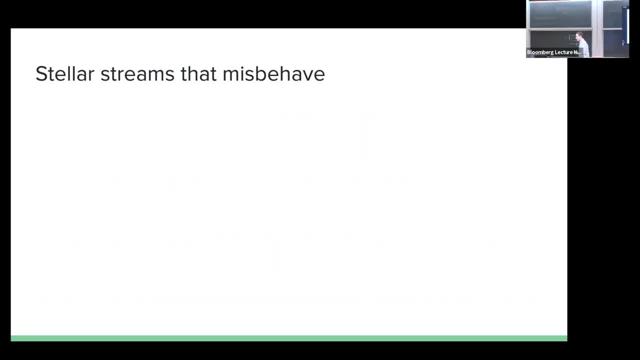 that stellar streams misbehave in our data. So, unlike this picture that we would have liked to believe, where each stream responds nicely to an orbit and then we can look at all these orbits in one simple potential that isn't evolving, is not changing and is just as defined by a smooth form, 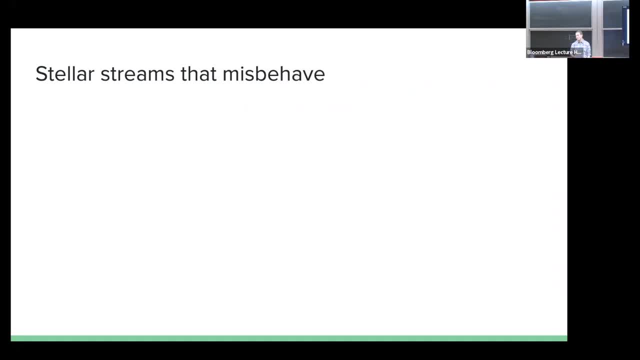 turns out that's not the case. We know the Milky Way is evolving. It doesn't even come as a surprise. We know there are other things that contribute to change the way these streams evolve. There is smaller scale structure in the Milky Way. 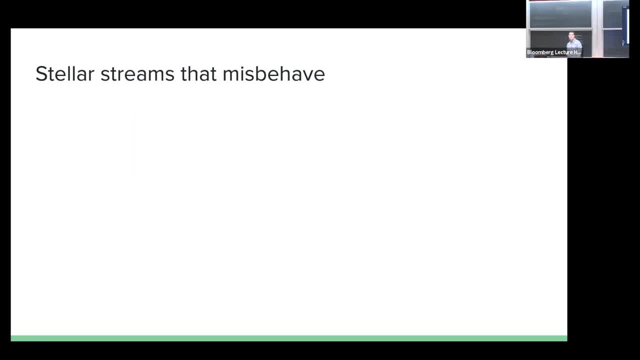 There is potentially smaller scale dark matter structure. There's certainly smaller scale baryonic structure, bars, spiral arms, GMCs. But Milky Way, The potential is evolving. So the Milky Way's potential five years ago, when perhaps one of these streams started evolving. 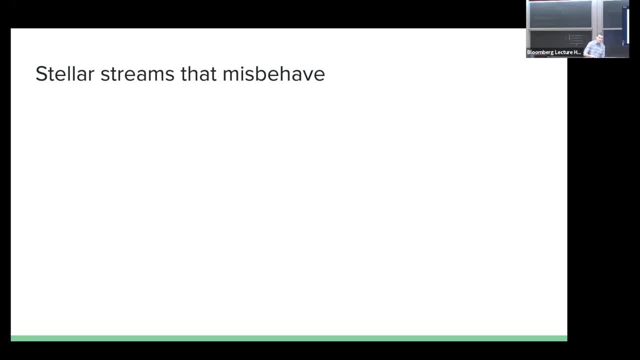 is not the same potential in which it's evolving now. The LMC has fallen in. It's tugged things away from where they should be, And so trying to model these things cohesively has actually turned out to be much more complicated. 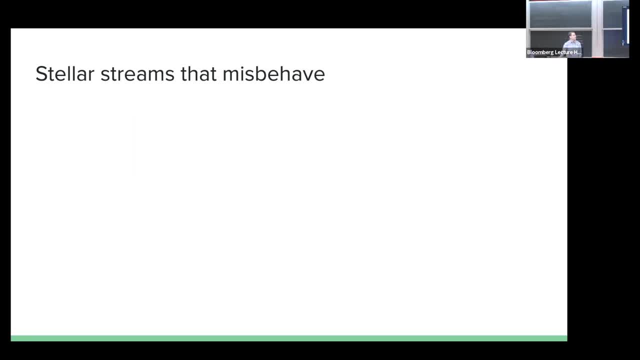 because it turns out, when you try to make these simplifying assumptions, you've got one stream that tells you: well, the potential should be x, And then you've got a second stream that just rules x out entirely, And the answer is: oh, we needed it. 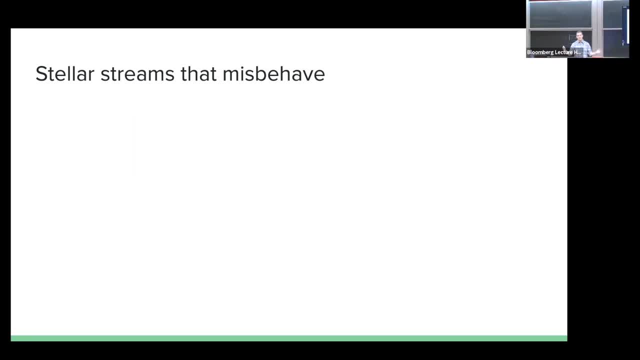 to take into account something like the LMC, which tugged at one of these streams but not the other one, for example. So you've got all sorts of these little examples that have popped up in literature. I'll just flash a few of these kind of a newsreel highlight. 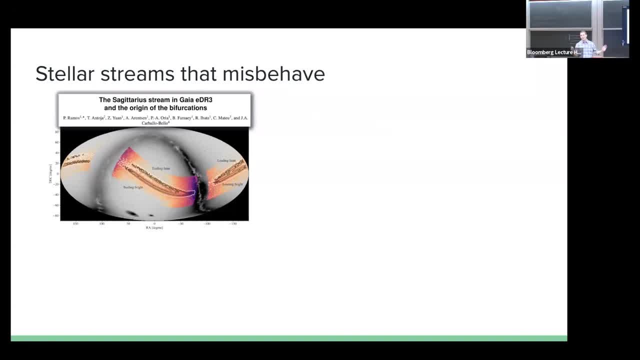 Sagittarius. that stream that I showed in this big blog has a bifurcation. We've known about this bifurcation for a while. How do you model a bifurcation? How do you get two different tracks And what is the orbit if there are two different tracks? 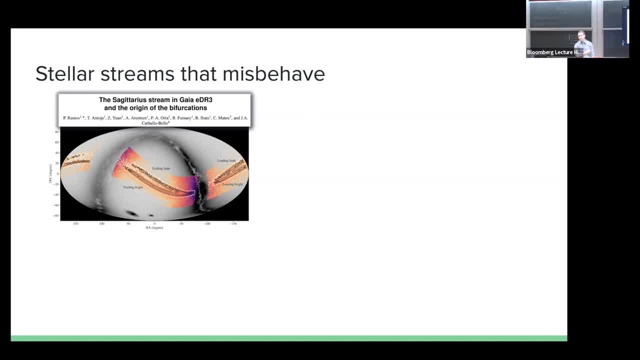 that you think these stars are spread on. One theory here is that this teaches us about the progenitor, actually Sagittarius itself. dwarf galaxy had rotation, had something else: flung stars out in different ways. So you've got a bifurcation, maybe. 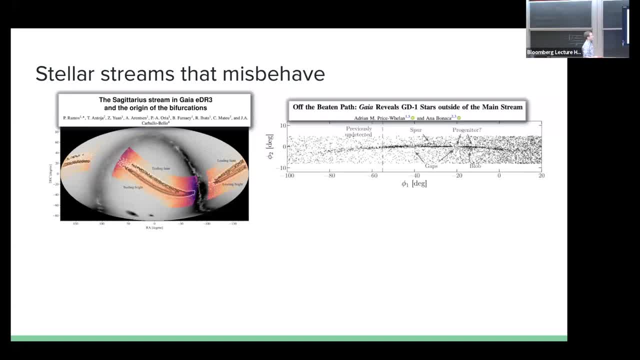 Not necessarily the answer, but certainly an answer. GD1, the stream I showed earlier- now I can talk about the little labels here- has all these gaps and a spur. How do you explain these gaps and how do you model the spur? 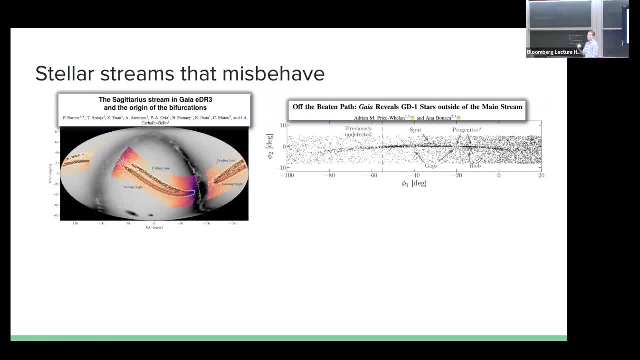 How do you get a stream that has these kinds of features? Maybe this is substructure In the potential, maybe these are dark matter halos that are punching through the stream and creating these under densities over where those two arrows point and pulling off the spur of stars. 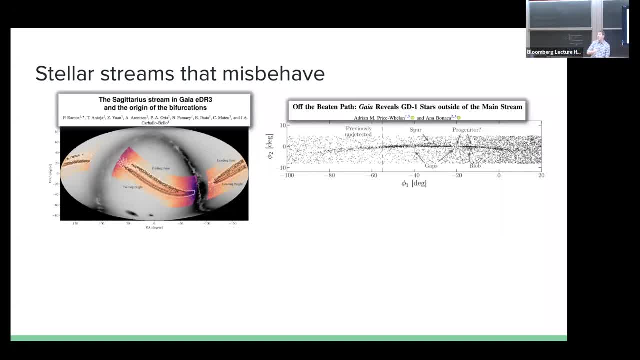 Maybe. Maybe it's an intermediate mass black hole that's punching through it. Maybe it happened to fly by a GMC. We don't think it's a GMC, But who knows Why not a GMC? Just the orbit doesn't, Doesn't bring it anywhere close enough, I think. 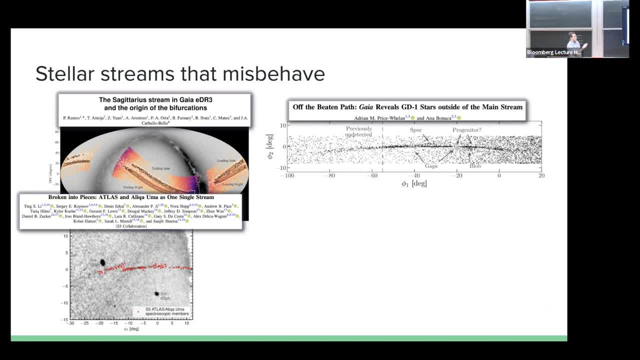 to known populations of them. Streams that appear to be broken up, or rather two streams that we thought were two separate streams, have actually turned out to be very similar in terms of their chemistries. How do you explain that? Do you try to model these as two separate orbits? 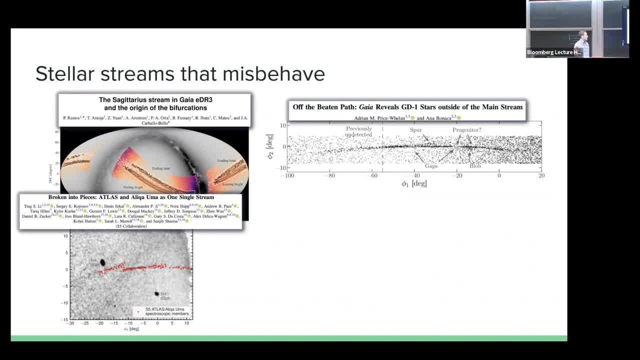 or do you try to explain them as one orbit that maybe, in this case, Sagittarius plowed through and pulled off an entire arm to a slightly different, different inclination along this orbit? So there's a nice YouTube video which, if I have time, 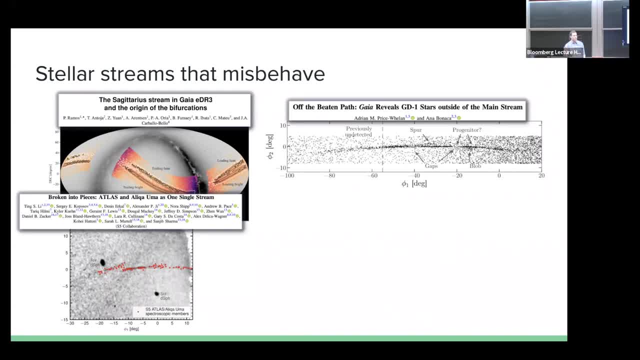 I'll show at the end, which shows one simulation in which, if you include Sagittarius in this, you kind of Sagittarius plows right through here and pulls off this secondary arm. And now, as many people thought to allow these two streams, 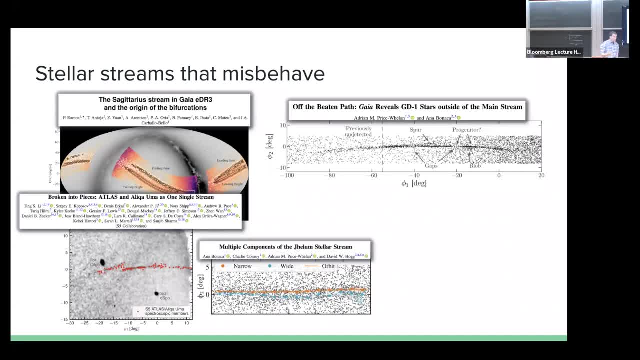 actually they're just one stream, Multiple components, though similar to the previous one, the stream that has a thin track and then a wider track, which is a little hard to see here. Below the thin track there's kind of a wider over-density. 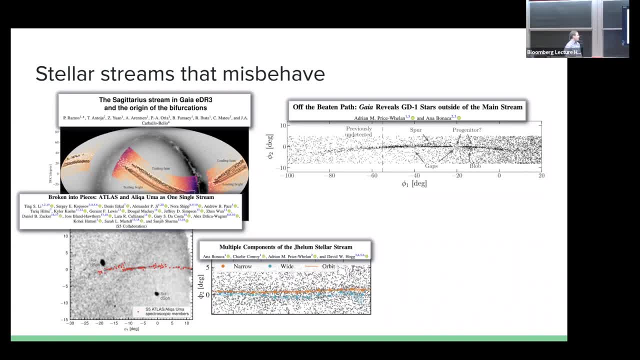 compared to the background. This one, as far as I'm aware, doesn't even have a good explanation yet, besides there being well two kind of parallel stream tracks that I can't really explain well in terms of formation mechanism or something in the potential that has induced them. 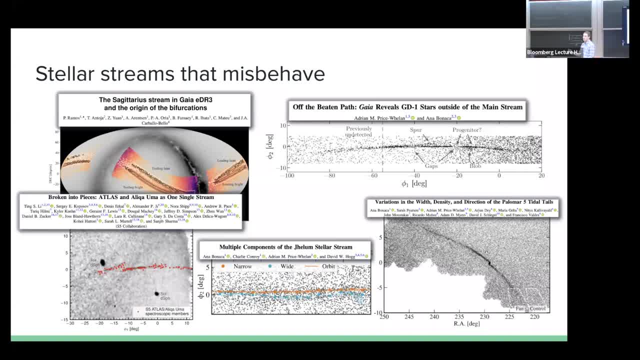 Pal 5, the stream I showed in the beginning has a very stark asymmetry between its leading and its trailing arm. One of the arms is quite long and thin. The other one has a fan that appears quite soon after the progenitor that's shown right here. 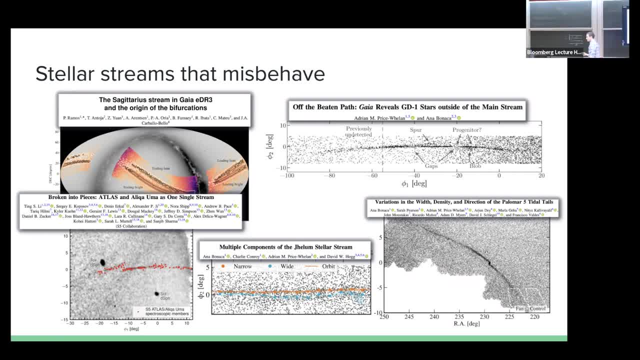 where the stars stand out. How do you get that? Well, the leading explanation now is that there is an interaction with the galactic bar that sweeps by and torques some of the stars in one of the arms, away from their orbit. Other things that have been invoked to create this. 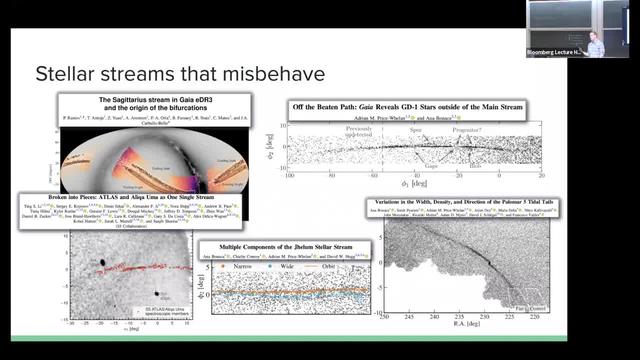 are flattening the potential, and chaos in certain regions specifically affect one of the arms here. I'll address that later in the talk. Bottom line is There's a lot going on in the streams that move away from this very simple picture of a smooth potential. 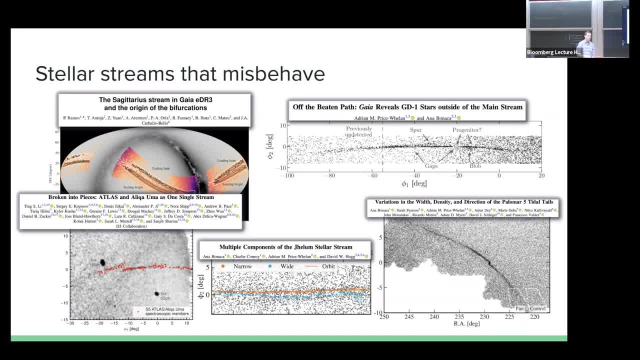 in which a stream is evolving. If you're a glass half empty type of person, you might say, OK, this is hopeless, We're never going to get back to this original picture. A glass half full person might say: well, this is all very interesting. 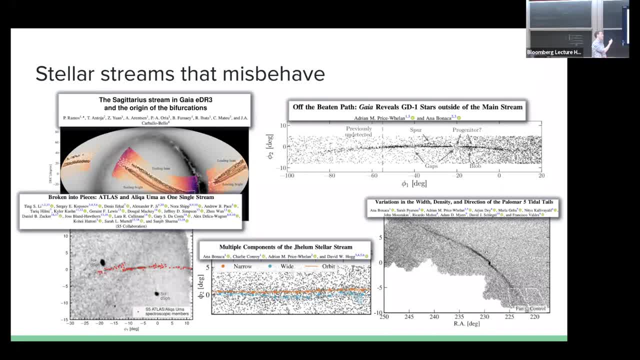 because we're learning other things about the potential in the process. We're learning about the properties of progenitors, We're learning about dark matter substructure, We're learning about baryonic substructure, bars and so on and so forth. in the potential, 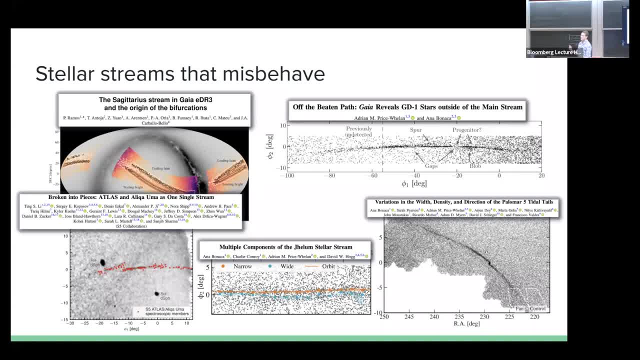 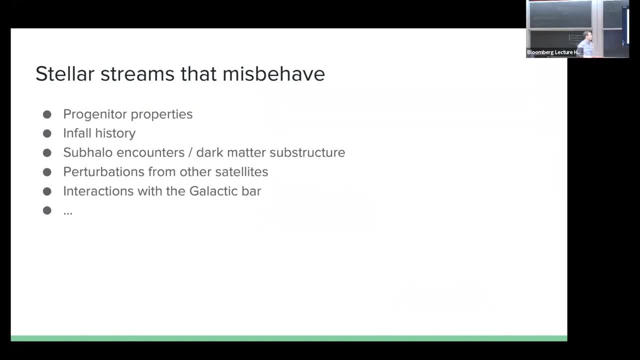 So there's a lot of Yeah Information in these perturbations and these deviations from the typical stream, like picture, But what I want to do is I want to bring it back to our original question, which is: so we've got all these possible things that we can learn. 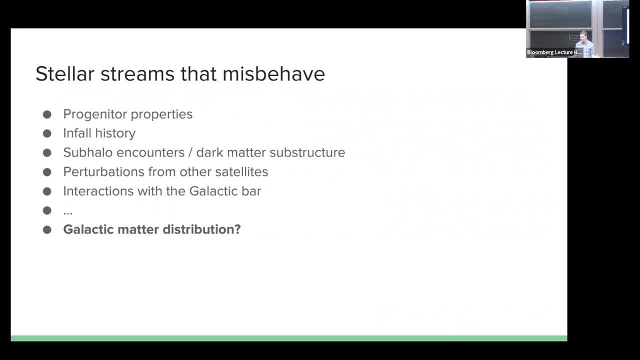 from this in stellar streams. But I want to go back to what is the overall galactic matter distribution? Can we still, given all these deviations and the fact that it's actually very hard to model multiple streams with one potential, can we still figure out something about? 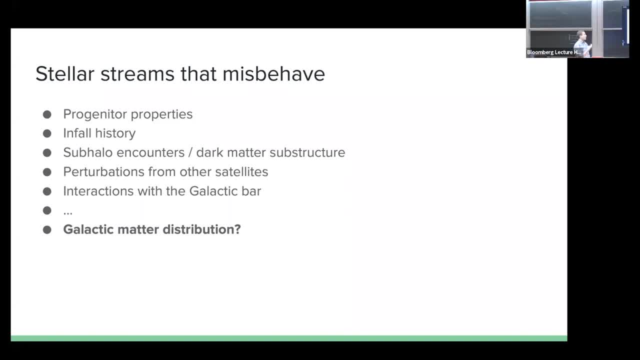 again the overall shape and structure of our halos from these streams. And so I want to come back to my solar system, to Milky Way analogy, and talk about a different game that we play in the solar system, which is- well, I call it seeing orbital structure and seeing. 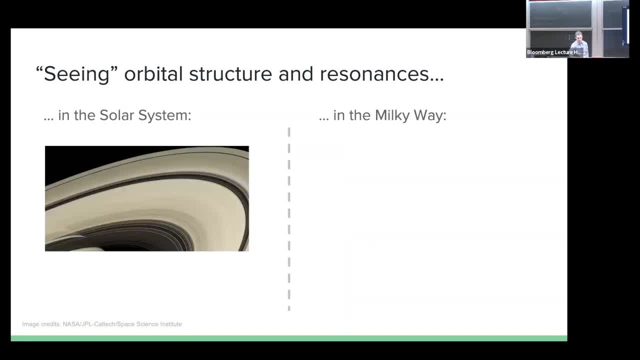 resonances in the solar system. Here is a picture of Saturn and its rings. You learn a lot about the matter- distribution in and around Saturn- from just a snapshot. again that we didn't see these rings at all. All you need is a snapshot of these rings. 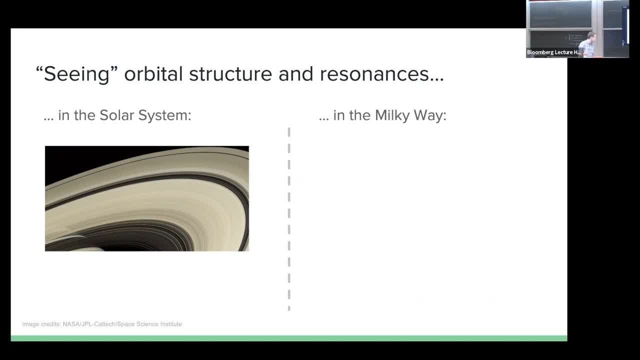 These over and under densities are indicative of various resonances with local moons of Saturn. Even I learned the other day, talking to you both, that you can even do seismology with these rings. You can learn about modes that are excited within Saturn that induce a resonant response within the rings. 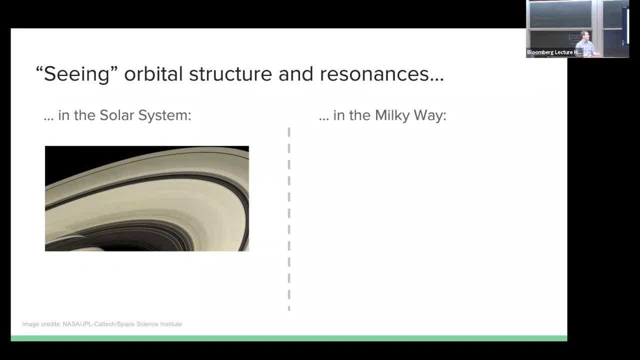 You can actually learn about the matter- distribution inside Saturn- kind of to a very detailed level from looking at this very fine ring-like structure, And so one of the main questions I asked in my thesis was: can we do this in the Milky Way? Can we see orbital dynamics? 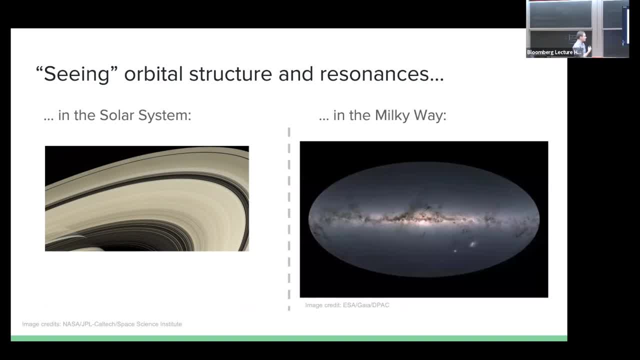 Can we see resonances in the Milky Way, And here we have a similar, although maybe reverse, problem. as I mentioned before, We have a snapshot but, more importantly, the Milky Way is very dynamically young compared to Saturn's rings. Saturn's rings have evolved and these secular resonances 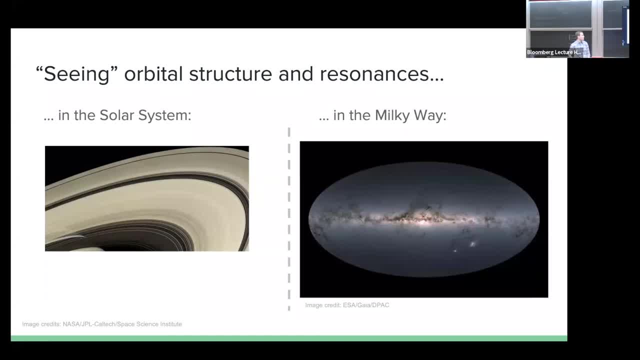 have taken their effect and created a very clean structure, whereas the Milky Way is between 10 and 100 dynamical times old, depending on how far in you go, And that's not necessarily enough time to actually see the effects of these long-term secular. 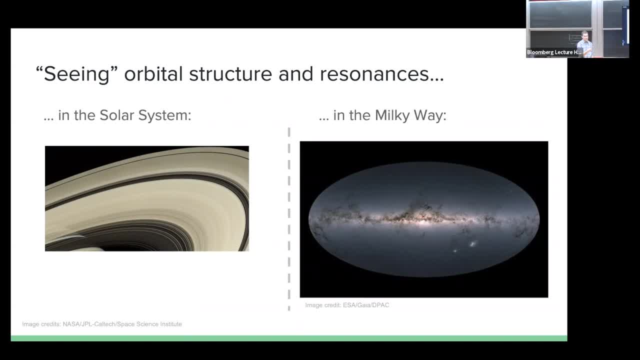 resonances, And so some people might say at this point: well, we shouldn't try to play the game of looking at long-term secular effects in the Milky Way. I'll try to convince you that, whether you want to call it secular or not, these effects actually matter. 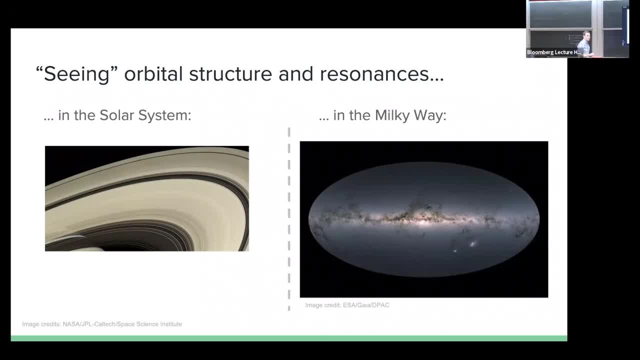 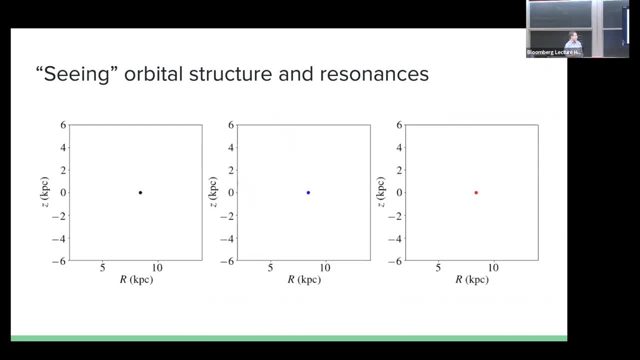 And studying resonances and resonance structure in stable and unstable balance points can teach us something very interesting about the potential of the Milky Way. To start out, I want to talk about what orbits look like in the vicinity or inside resonances, And so I'm showing here three orbits, now plotted. 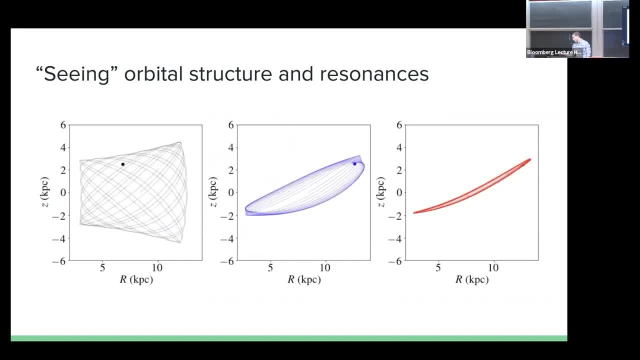 in their radius and their vertical excursion from the disk In a Milky Way-like potential. this potential has a disk, so a flat component which we know do exist, the baryons. It's got a halo. Overall it is axisymmetric. 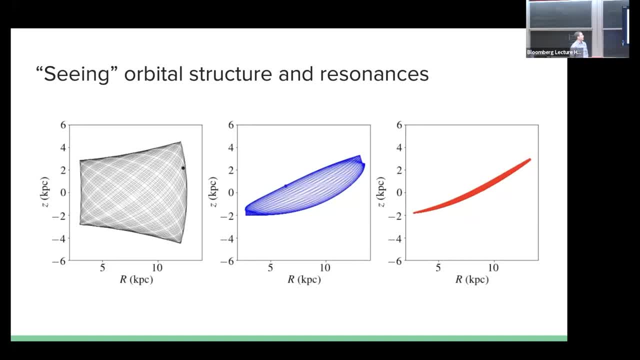 It's oblate because the disk is creating some deviation from sphericity. In fact, I think in this case my halo is also oblate. This is a very oblate case. This orbit on the left is a very typical orbit. 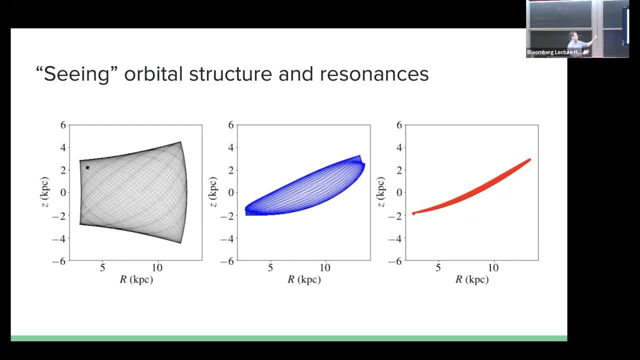 In a galactic case, it fills out its entire orbital torus. You see that in this RZ projection, as it's filling out the allowed space for this orbit, this symmetrical diagram in RZ, This is what a normal I would say. 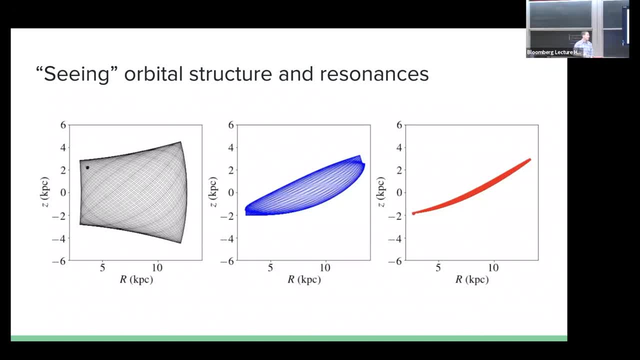 orbit, a regular orbit in potential, looks like. If you look all the way to the right, you see an orbit that is basically a completely commensurable, an orbit with commensurable frequencies. The reason that orbit on the right doesn't fill out the full space like the orbit on the left. 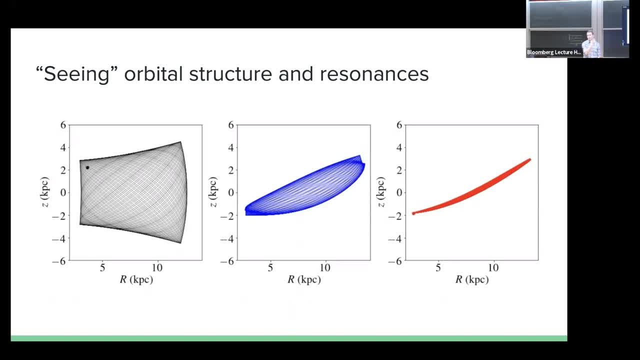 is because its radial frequency and its vertical frequency are exactly the same, are 1 to 1.. So every time it does a radial oscillation, it does a vertical oscillation and it just repeats the same figure in its R and Z plot. 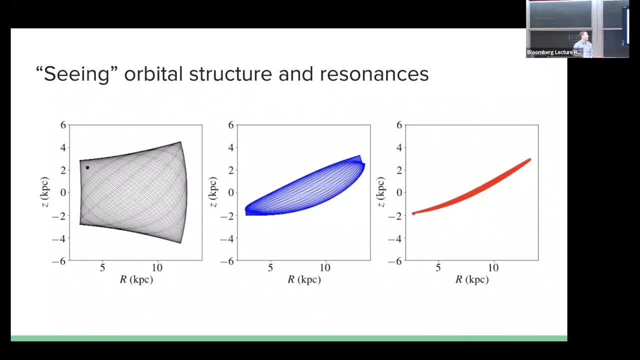 So it just kind of forms more or less than one. Yeah, This line, The orbit in the middle, is the one that I think is interesting. This is what we call a resonantly trapped orbit, So it's not exactly on the resonance. 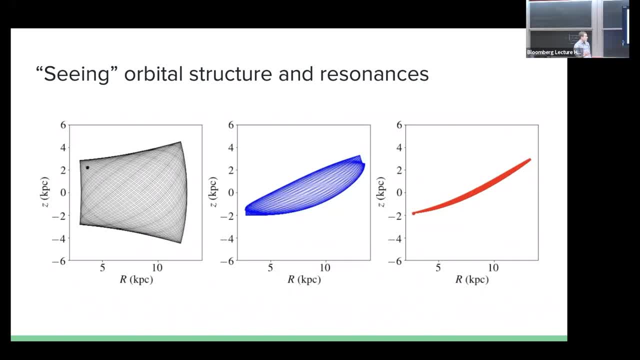 It is deviating around, away from the resonance, but it is close enough And because the Hamiltonian in this case depends on R and on Z, it's an oblate potential. it's getting tugged back to the resonance over many orbital periods. 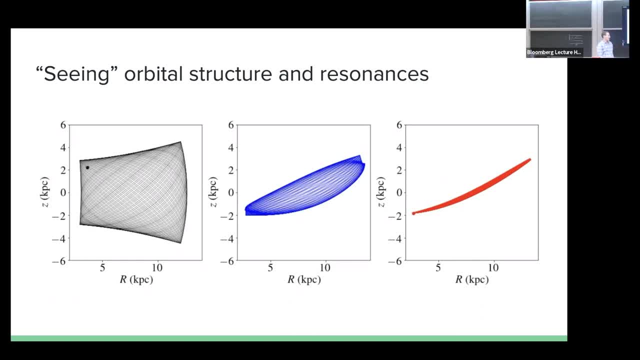 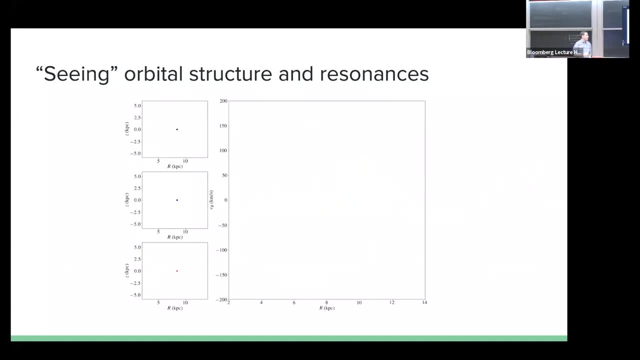 And it's never leaving to the opposite, the opposite shape. It never gets up here or down there in this diagram because it is trapped at the resonance, essentially oscillating or vibrating around the resonant orbit all the way on the right Good. 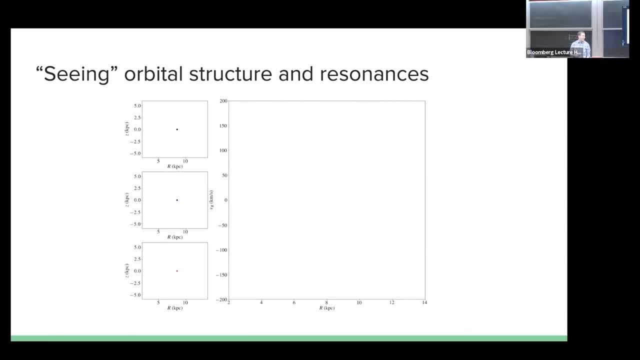 I'd like to visualize these in surfaces of section. This is one of the main projections that I think is useful to study these resonances. So now I'm plotting again the same three orbits you saw before on the left, And each time one of those orbits. 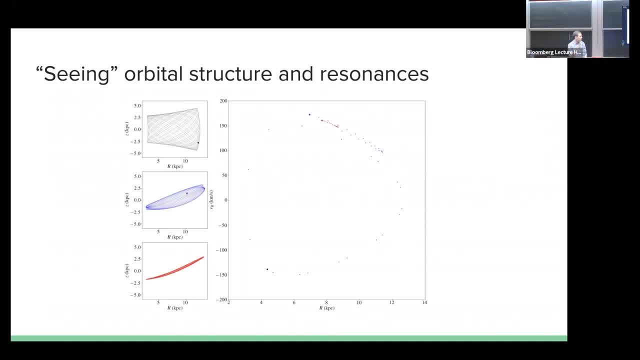 crosses the Z equals 0 line going upwards. I log It's radius, it's R and it's radial velocity on the plot on the right And it might be a little hard to see right now but hopefully eventually you'll see the contours forming. 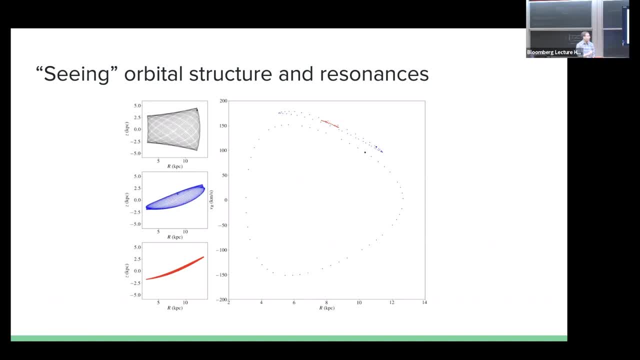 The black orbit, the regular orbit, is forming this big round, one little circle or almost circular-like shape here, whereas the two resonant orbits- the one that's exactly commensurable and the one that is trapped at the resonance- kind of get stuck. 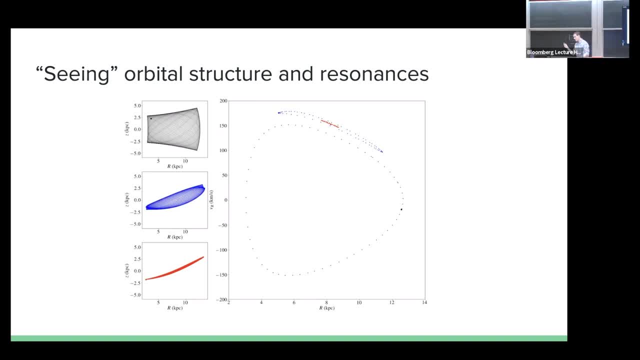 at the very top of this plot and just move around the very top. They never make it To the bottom. that's essentially the same statement as saying that this orbit will never get to here or to here, It just stays on the top of the section. 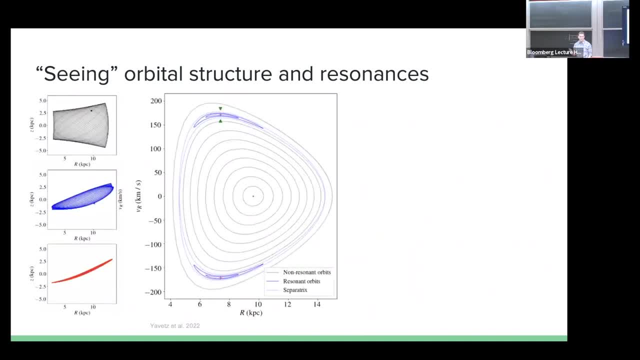 Here's that plot, shown with more orbits and filled out so it's easier to see. You can see most orbits in this choice of initial conditions will be regular orbits, though they are concentric around this point, So most of the orbits are like the black ones. 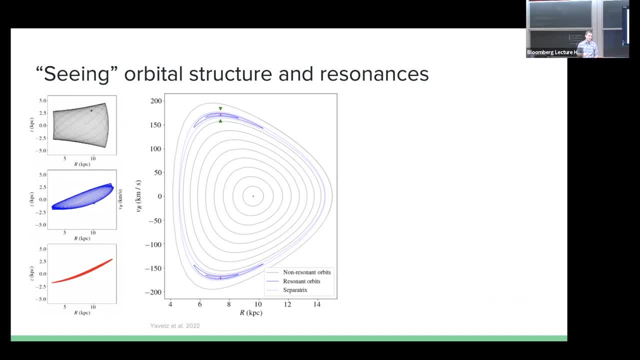 But you can see that there's this class of orbits at the top and the bottom that are resonantly trapped, that behave just qualitatively differently than the regular orbits. And again I want to stress, this is a smooth potential. There's no additional structure beyond the fact. 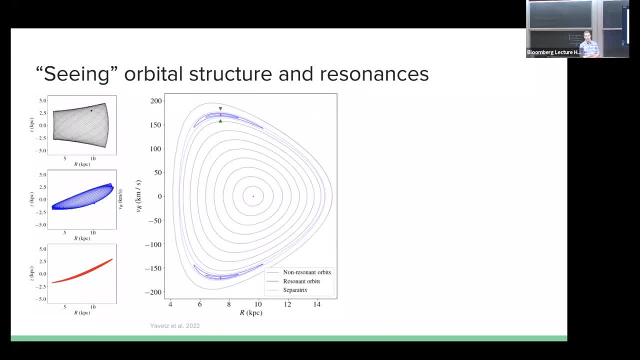 that we have an oblate configuration and not a spherical one. And yes, I said there's a disk. You would get this even if there weren't a disk, but you just had a smooth oblate halo Good, Why does this matter? 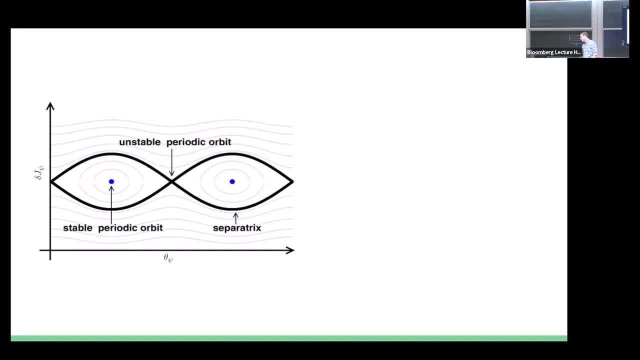 Why do I care? So here is you can study these resonances in action angle space again, And this is what we convert to slow action and slow angles. This diagram is equivalent to this diagram, which is basically, I said before, everything evolves very regularly here. 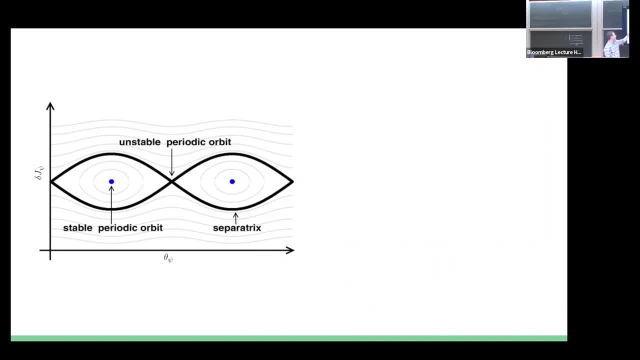 In fact, what you get in these resonantly trapped regions is a very different picture, where instead of this very clean linear evolution, you have your vibrating orbits trapped in this resonant region around the stable balance point, And then you've got orbits above and below that. 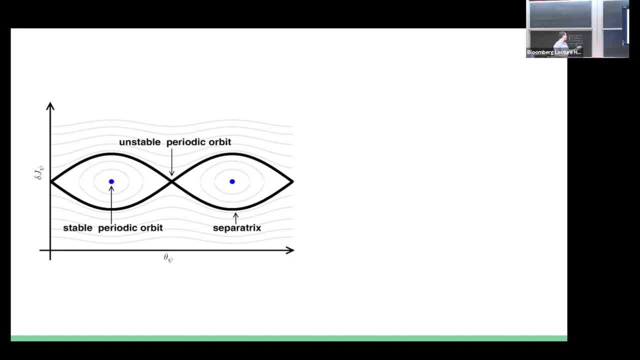 kind of circulate around it And you have to get far enough away to get back to this simple linear picture. I want to bring back that picture I showed earlier and say now: imagine, instead of that evolving here, you have that blob. start out here and let it evolve. 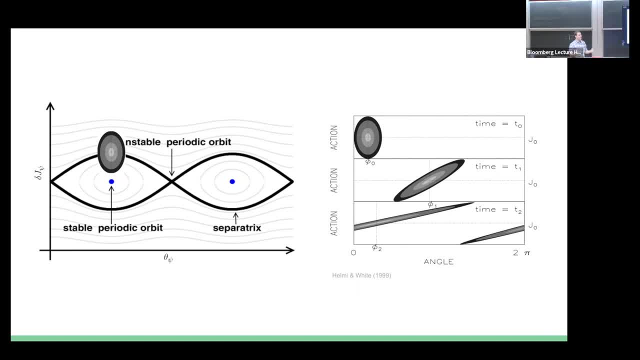 And now I'll just let you imagine. I didn't actually take the time to draw what this looks like, But just imagine if this thing is moving kind of relatively similar frequencies. That's not necessarily true either, But let's assume they're all moving with similar frequencies. 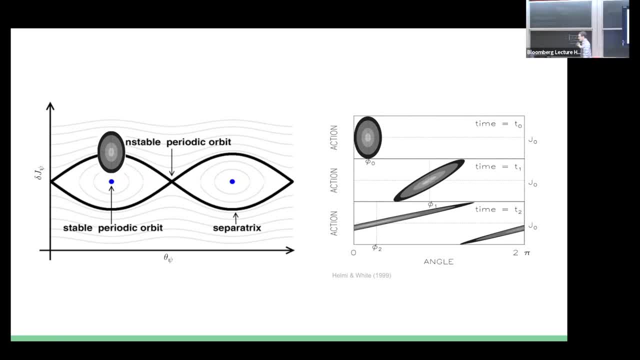 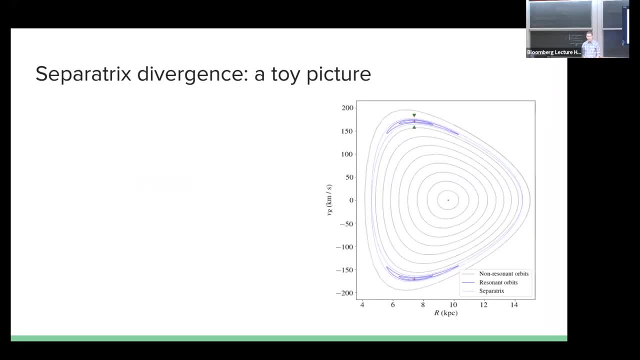 along these contours. What are you going to get? It's going to look very different. It's certainly not going to give you the simple linear shearing picture that you've got at the bottom of that figure on the right. Bringing it back to my surface of section, 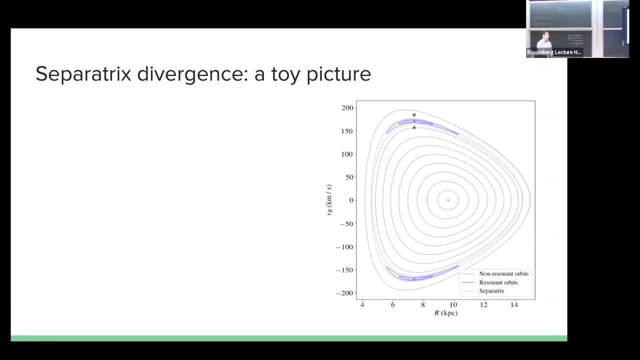 let's draw now a toy picture with actual kind of what is the behavior of a stream here? We certainly can detect it from seeing one orbit. If you see one orbit, that basically gives you a point on the surface of section. It tells you nothing. 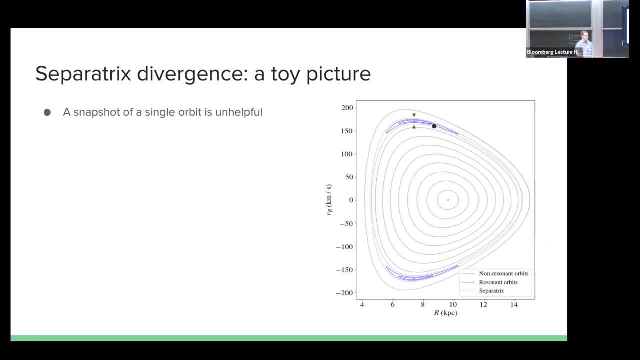 You could have a resonantly trapped region. You could also have a not resonantly trapped region. It would still appear as a point. So you wouldn't be able to know from just a single star in its current orbital parameters, is it resonantly trapped? 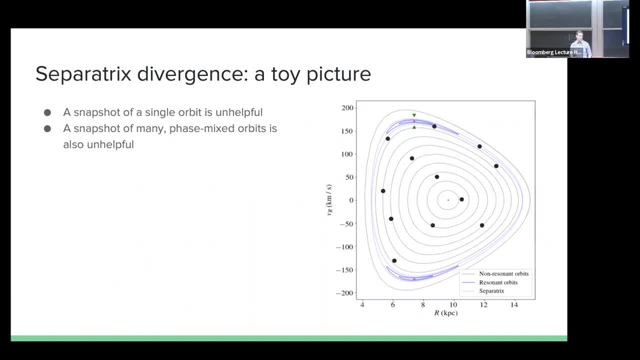 You can't even do that with a distribution of points. So a snapshot of the Milky Way: if you see a lot of stars and they're all orbiting, there's no way a priori to figure out if some of them are resonantly trapped or some of them. 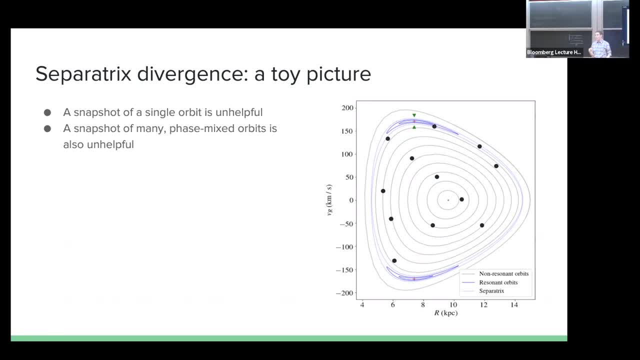 are not, because the thing of it, the contours of drawing them back, are potential dependent. So if you don't know what the potential is, you just know the 60 phase space information of each point. here you could equally draw a non-resonant. 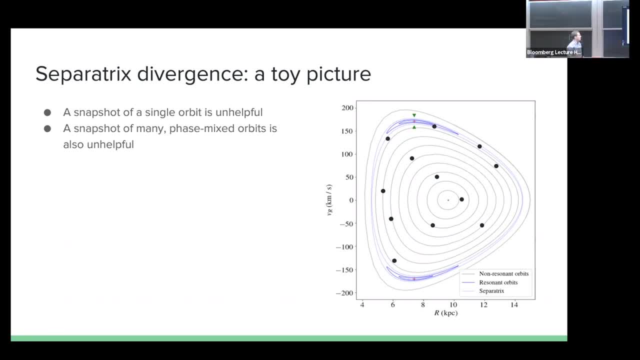 picture and have them fill that equally. There's no way over under densities that you can easily detect in the data. if you start out with a smooth distribution and you evolve that way, Maybe there are, but that's a story for another time. Bear with me for now. 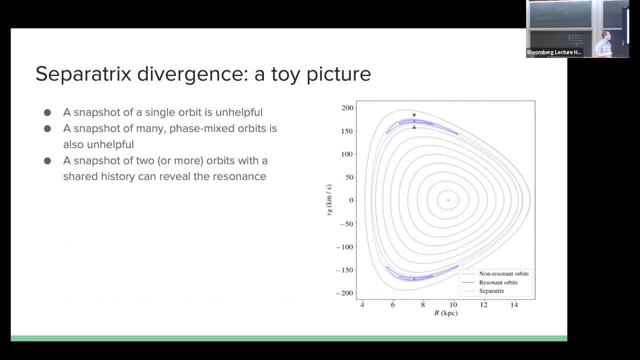 You can, however, very easily detect these resonances if you have two or more orbits that you know have some sort of a shared history. So if those two orbits both started on regular orbits, they will do the same picture that we saw here. 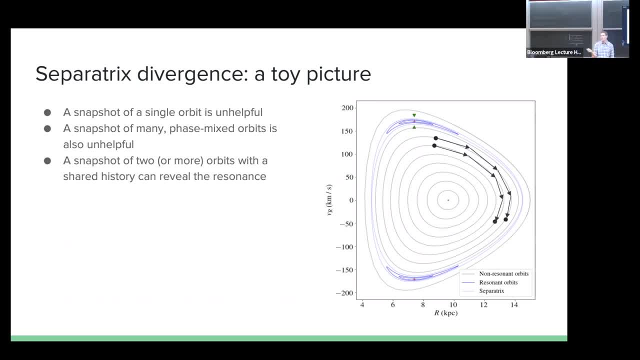 They'll move along the orbits and they'll shear slightly, because one of them has a slightly different frequency than the other, Whereas if those two orbits started straddling the boundary between the resonant and the non-resonant regions of the phratrix, 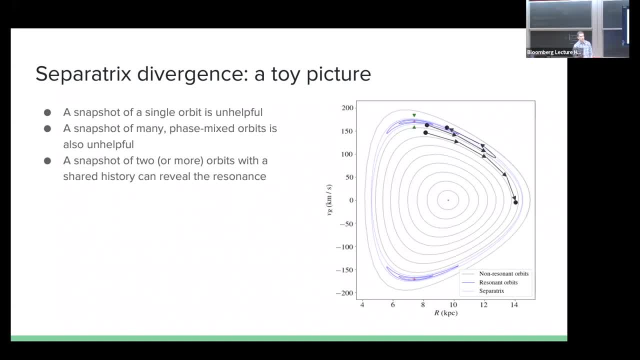 then those two orbits will initially evolve together, But then one of them will turn around and you will split apart, essentially appearing to have diverged a lot more in terms of your phases than one would expect from the typical picture. So if you know that these stars started out together, 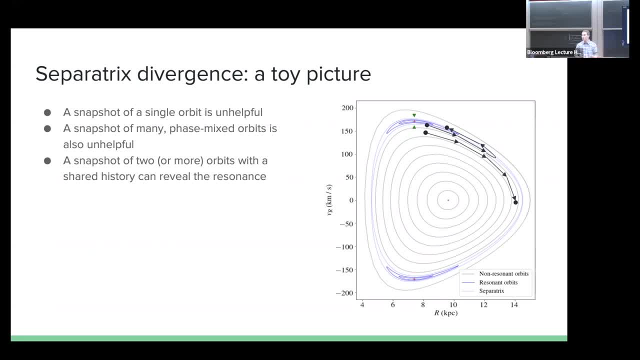 and yet they're so far apart from each other. one good explanation for that is: oh, there might be a resonance or really not. It doesn't even need to be a resonance, It needs to be an unstable balance point in the potential that has caused the flow. 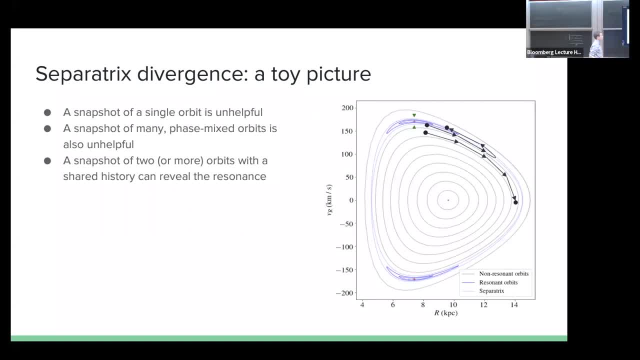 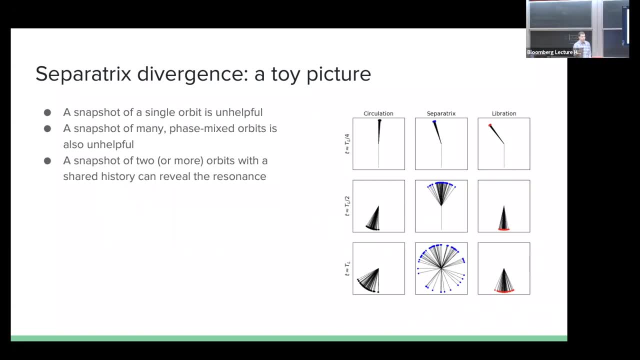 to diverge from the typical flow of two contours in the potential. Let's extend this to not two points, but an ensemble. Pendula are really good ways of modeling these kinds of resonances, So just imagine an ensemble of pendula that are evolving with similar energies. 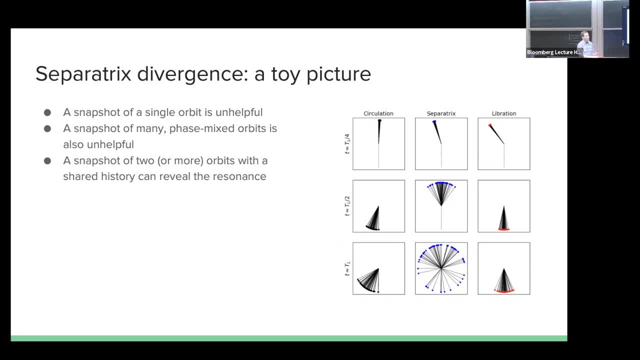 These are rigid pendula that are either circulating all the way around or they're vibrating back and forth. If all of the pendula are circulating and you start them all with slightly different circulating energies, they will all continue circulating And they'll start spreading out slowly. 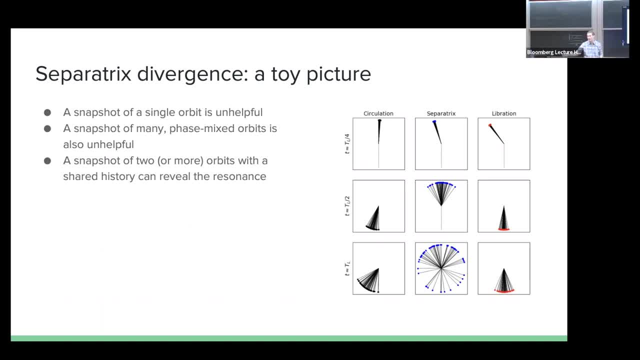 That's again your typical phase mixing. Same is true for the vibrating case, the oscillating back and forth case. If you happen to start them, though, such that some of them with the energy steps that some of them will circulate. 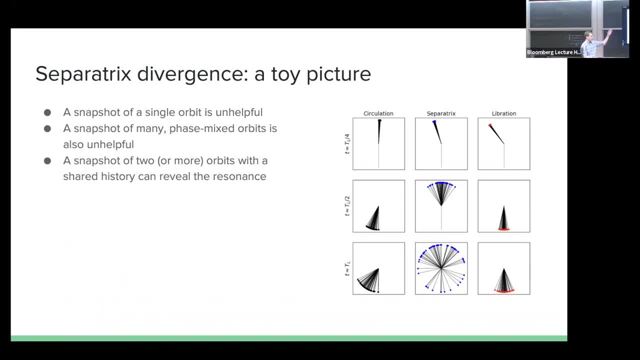 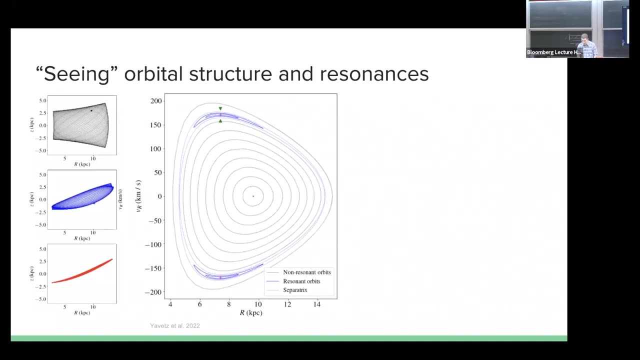 and some of them will not quite make it over the top and line, break that middle column. things will separate out very quickly, much faster than you would expect. from again, your prescription assumed no resonances in the potential. So now back to this picture. we've 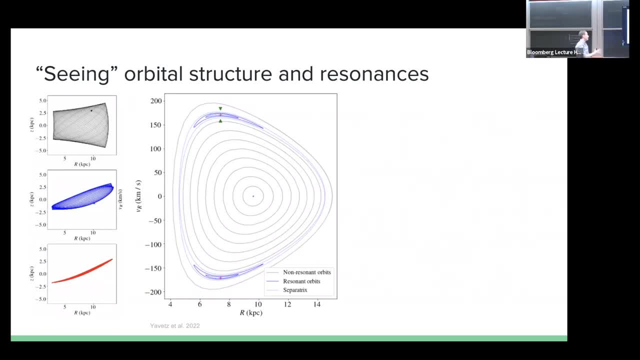 hopefully colored, this idea of resonances able and straddling the boundary between resonance and non-resonance: able to split you apart and face-to-face very fast. Now imagine that this picture, which now we can think of as initial conditions r and vr. 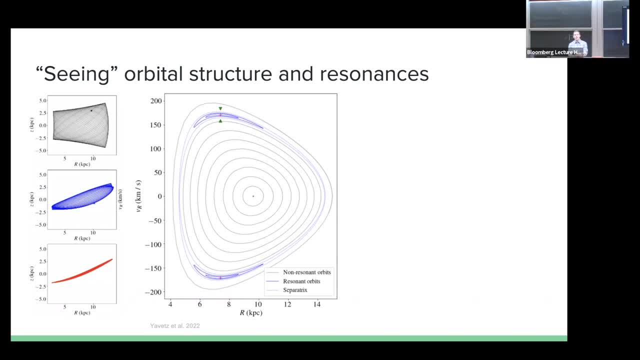 is covered with stellar streams or with globular clusters that will turn into stellar streams. You just try to populate this with lots of stellar streams, maybe many more than what we observe. I filled this diagram up with stellar streams, I would argue, and I think you all should, hopefully. 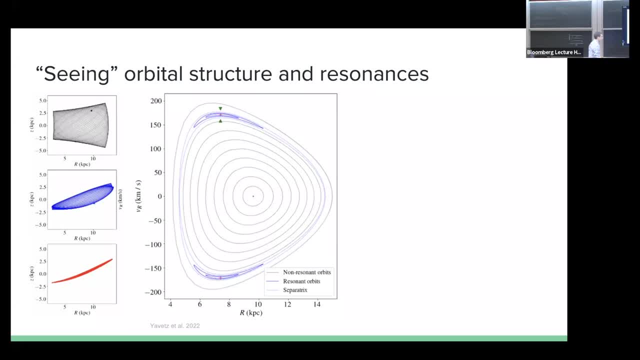 agree with me if I've done my job so far, that you would expect the density, the filamentary density, of streams that were born near this resonance to be much less than the density of the one dimensionality of streams that were born anywhere else. 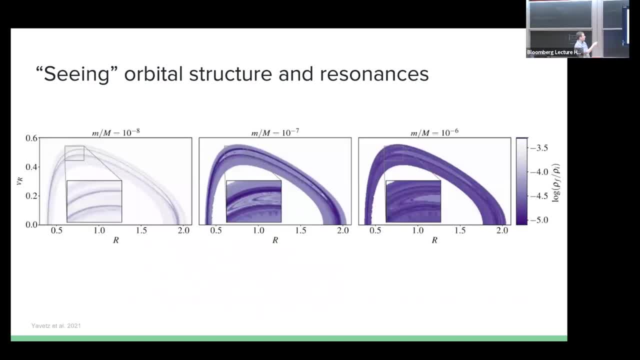 And so we've done that in simulation. This is the same axis here as the plot before, as this plot just half the top half of it, Except here. we know nothing about drawing these contours. All we've done is we've integrated globular clusters. 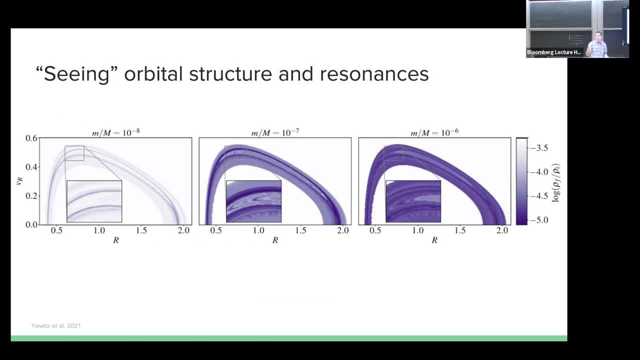 or ensembles. that model globular clusters in a galactic potential that is equivalent to that and measured their density after some several giga years And you can see that the density is darker here corresponds to less dense. The density clearly delineates where that separatrix is. 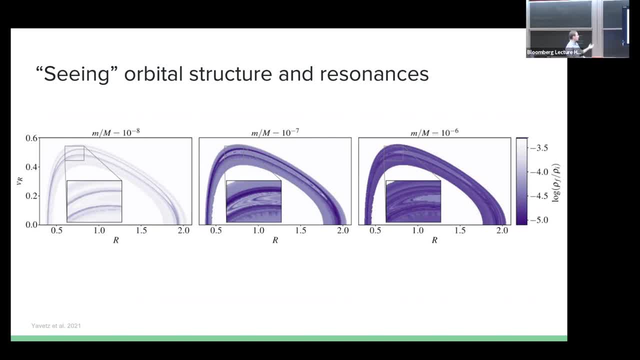 You actually see the contours of the surface of section I showed earlier in the density of streams- again assuming that your streams cover your entire phase space- to give you this very detailed probe of the potential. So if we had that kind of data, we would immediately 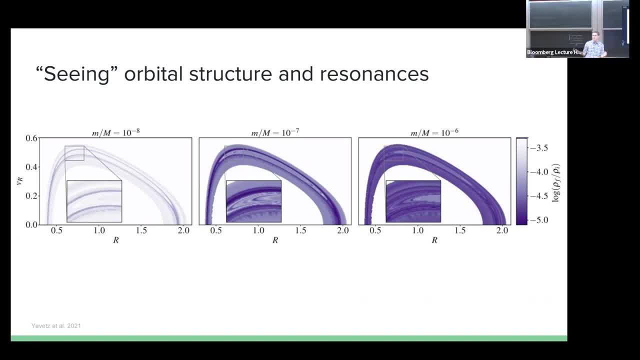 find these resonances because you would just look at the density of streams and say, oh, in a certain region in orbital space my streams are much less dense. They've kind of spread out a lot more than they should. Surely that means there must be some sort of a resonance there. 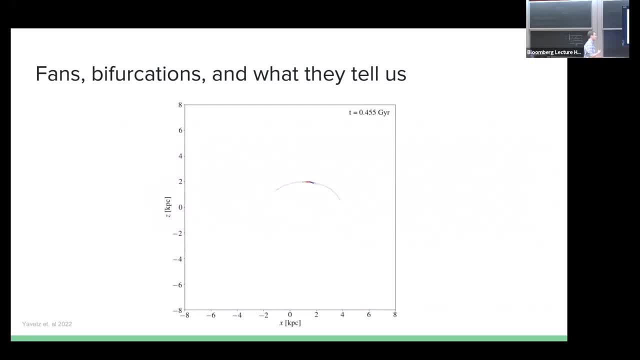 What does that actually look like? So here's actually a stream evolving near one of these separatrices. Some of the particles here will be trapped, Some will be untrapped. So far, everything looks good, nice and thin, more or less. 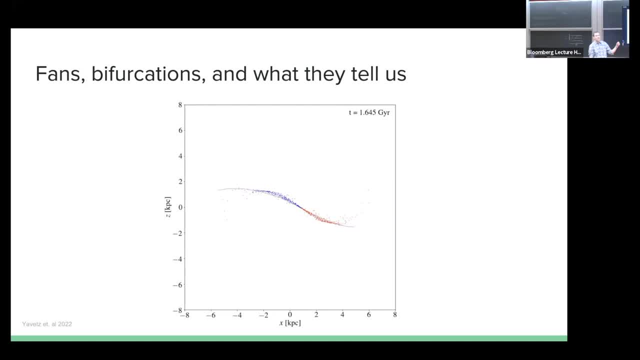 Stops in. There we go So far, so good. The gray line is the orbit. The leading and the trailing arm more or less delineate the orbit. So things are looking well-behaved right now. But wait, we're about to encounter. 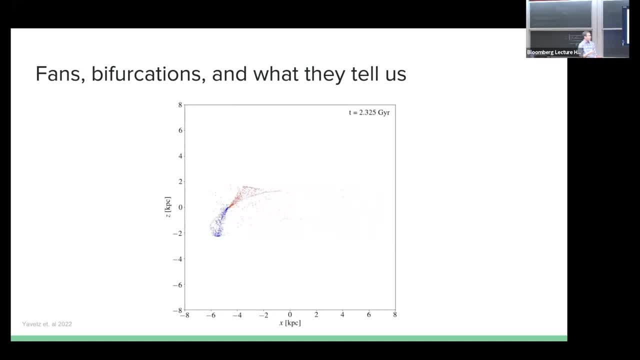 the unstable balance point. If you look at the red points, you're going to start seeing a red component that is just on the opposite side of where it should be. I'll highlight it: There it is. So look now. that's way, way away from where the orbit that we 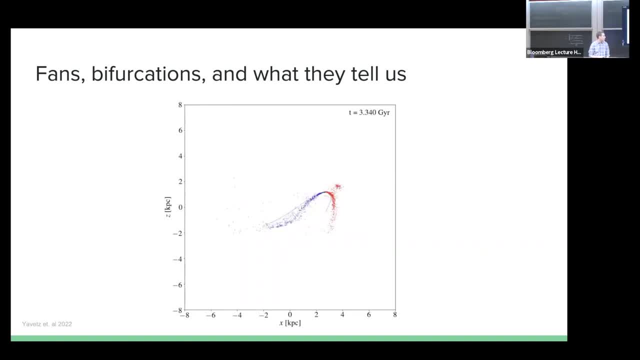 thought it was that should be is. If you keep looking at that red component, you'll see it actually looks. it started looking like a separate stream And if you pause this at the right time at an opportune moment, that might just look like a separate component. 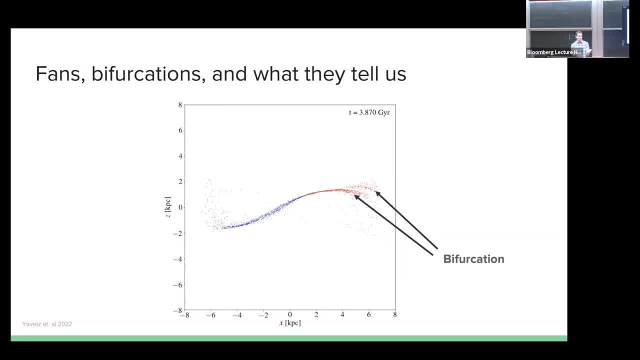 Or in this case, if you pause it, it looks like a bifurcation. You've got two streams, essentially, that you might not have associated to begin with, Or you might think that something got pulled off the stream, But here is a very elegant, dynamical way. 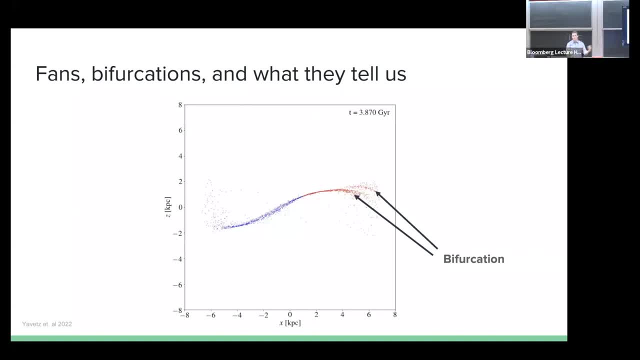 that doesn't invoke needing some perturb or something else, It just naturally in this potential you get these regions where the resonances will split up a stream into a resonant and a non-resonant component And you might get these separated components. 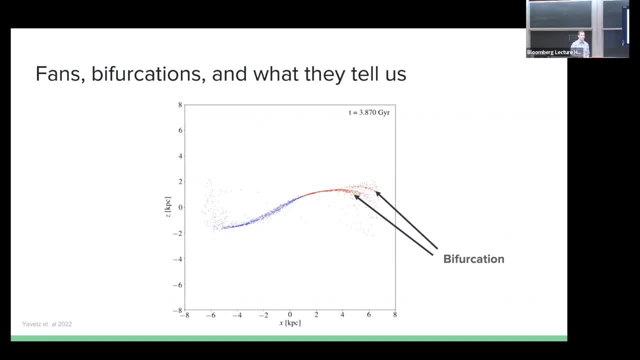 or these bifurcations, perhaps similar to some of the pictures I showed earlier in my newsflash of streams that misbehave? If you want to observe this, are you biased towards trying to catch it at this point, when there are one stream and another one which? 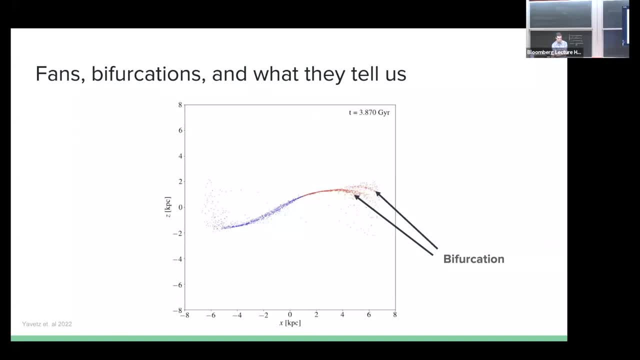 is close to it so you can go. oh, they might be similar. Let me look at their face, Because if you did the movie five, 10 seconds ago, they were on that side. we would never identify them. Well, the question is, if they are, if you get two kind 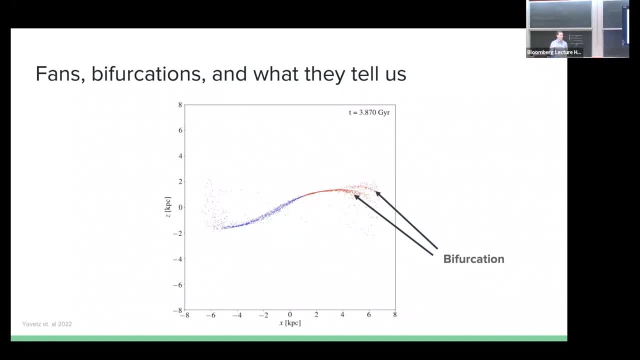 of distinct stream-like components. you're biased to think in two different ways, right? So in this case you might say: ah, I see the stream and there's a component next to it. Maybe this is like a bifurcation, like a GD1 has the spur. 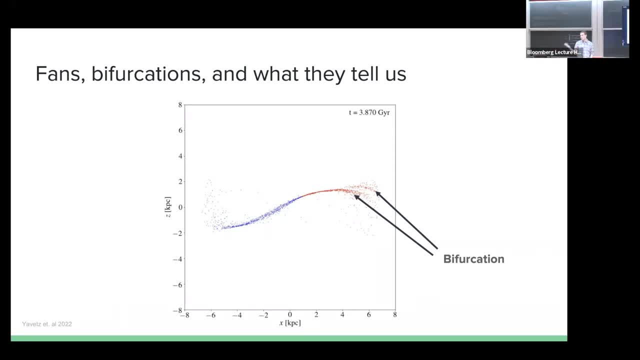 If you see them in two different sides and you still detect them. so first of all, you're maybe less about, you're biased to not detect it if it's far away, But maybe you'll see it and you just won't associate it. 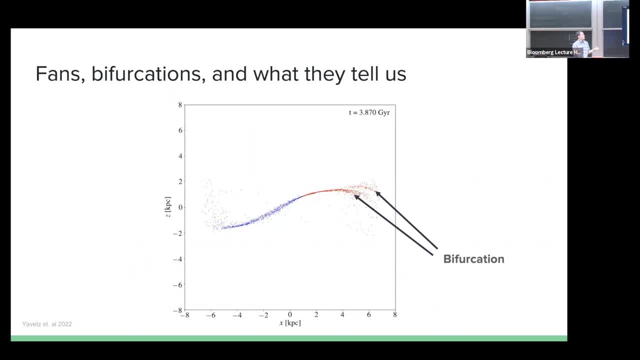 with the stream. Maybe you'll say there are two separate streams and you'd have no reason to associate between them, unless you happen to choose the right potential in your model here, which would require a lot of luck. Yeah, Or you've had some other indicator of, say, age or chemistry. 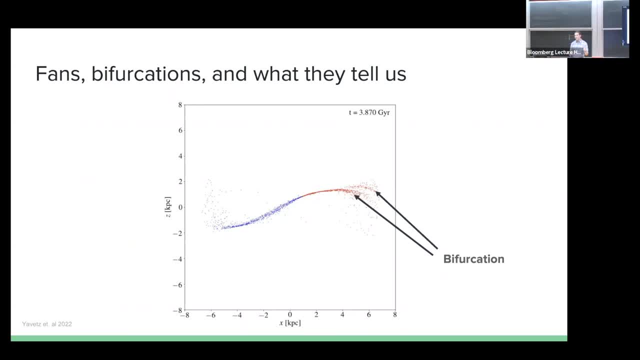 to say these two components are awkwardly similar kinematically. They're awkwardly similar in terms of their chemistry, and yet they're so far away from each other. in reality, What happened? Not that there are streams that have such characteristics. There are. 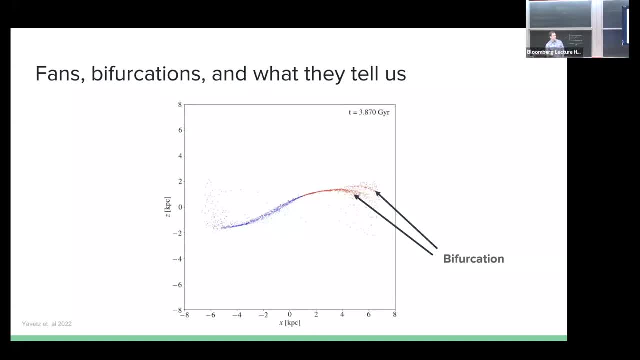 There are, So I could show that slide earlier. There are certainly streams that have similar ages. There are streams that have that look more like this, where there's a bifurcation. We haven't yet modeled any of them using this formalism. 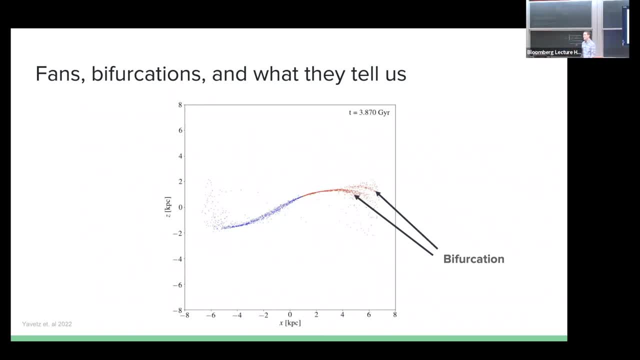 However, so far, I've only tried this on two unique cases. I haven't actually tried this across the entire catalog of data, And that is certainly one of the next steps, the main next step, I think, alongside what I will talk about at the end of this. 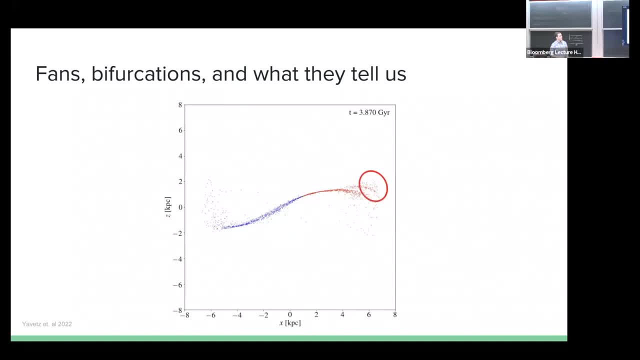 If you were to go back to that slide. if these are the different streams, do you have chemistry for all of them or in what fraction? Some of them you only have five or 10 stars for, so you don't really have great data on many of them. 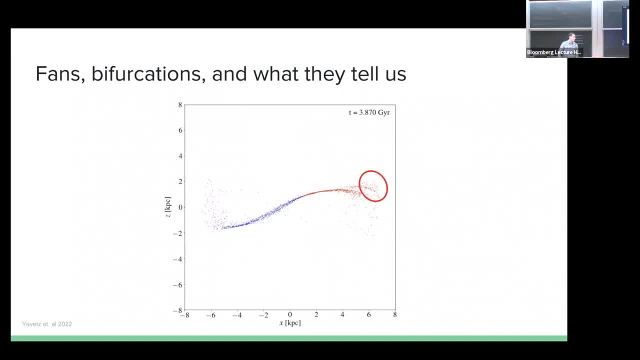 But it's getting better For some of them. you certainly do So. the case of JLM, which is the one that had two separate components, is a case that is both kinematic and chemical. The composition of the star is similar. 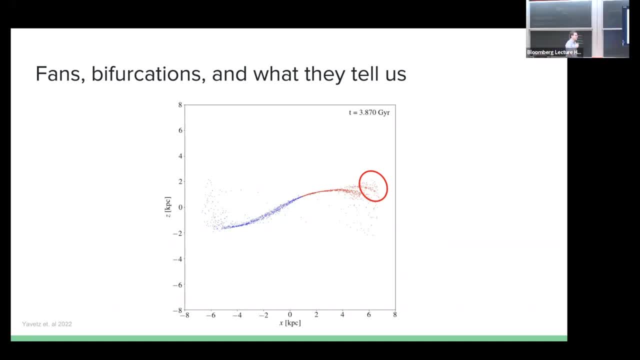 That's why they think it's the same stream. Not yet a good explanation. Unfortunately, for everything I've tried, that's the one I really threw everything at here. It does not fall near resonance in any of the potentials I looked at. 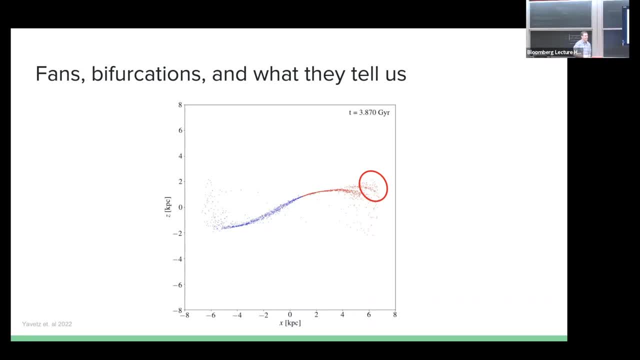 So shucks, But we'll keep trying. With something like that, would it be better to look for a companion to sanitary, Because that's a much bigger stream, So the chances that it straddles a separator it's a larger. 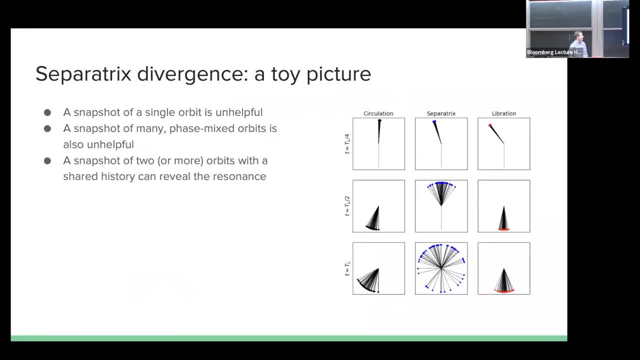 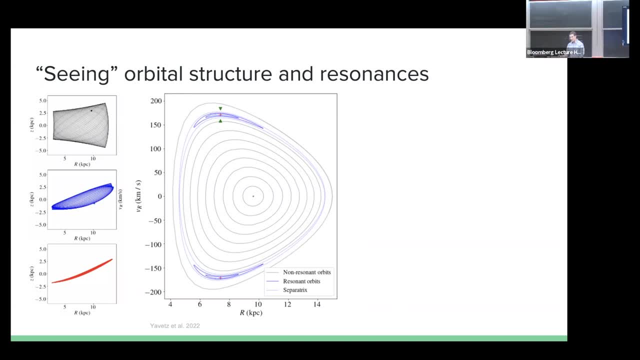 Yes, good question. You're asking all the questions that I typically get at the end, But we're in a no type here, So sanitary actually suffers from being too far in the extreme. I think in this case It's so big that it actually fills out a large portion of this. 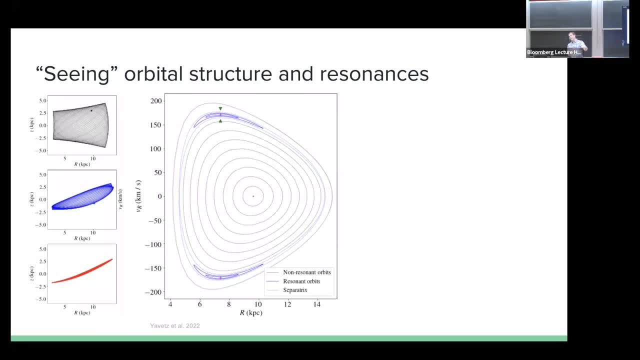 that you would have to pick out a very small component of it that stayed resonant And it really washes out through this diagram quite quickly that you wouldn't Everything I've tried. you have to either catch it exactly at the right moment before regular phase mixing overtakes. 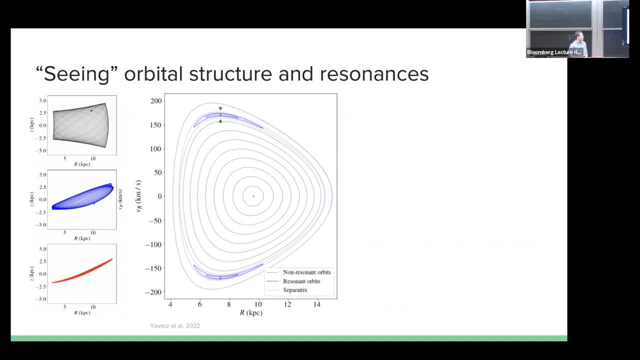 this accelerated phase mixing because you hit an unstable balance point Or you have to see a very thin component that is resonant, which is much thinner than the rest of the stream, which again would be hard to quantify and detect in the data. 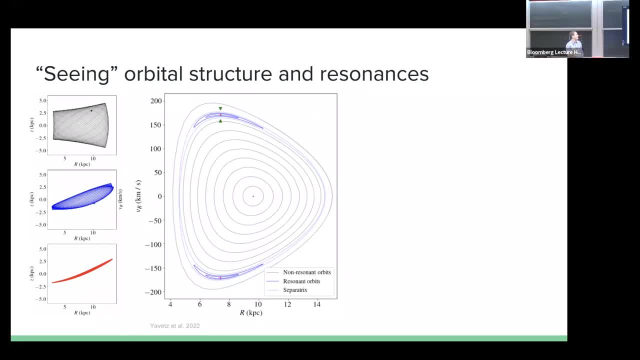 There is a very notable bifurcation in sanitarious. Don't think it's this. You'd have to have massive resonance which is way, way consistent with any of the reasonable prescriptions for the galaxy. The other problem sanitarious is it's way further out. 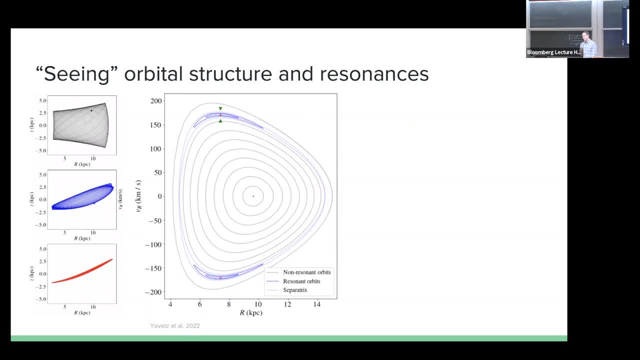 So it's orbited many fewer times. You actually need a good subset of orbits to actually pass by the unstable balance point for one component to go up and the other component to go down, So you would have to have gotten really lucky. The unstable balance point in this plot is here. 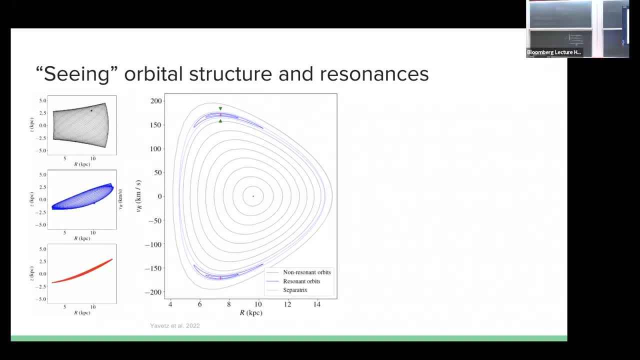 So sanitarious had to be born right around the unstable balance point. So in theory it could happen, But it is. It's a bunch of stretches you need to make to get there for sanitarious. So you mentioned that there are like 100 stellar streams now. 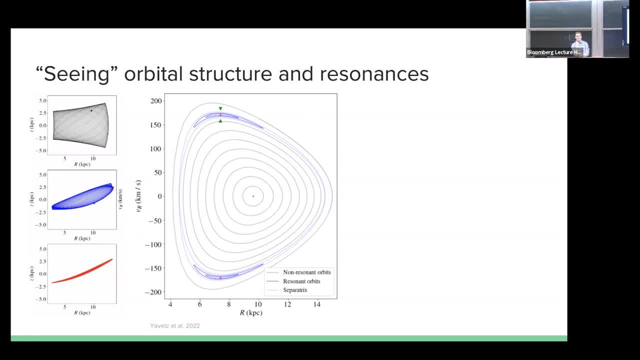 in the Milky Way. Do you have an estimated number, like how many of them have experience, or have just a metric? Remember the question. I have a slide on that exactly, which I will get to Before you get to that, so you may have just given enough. 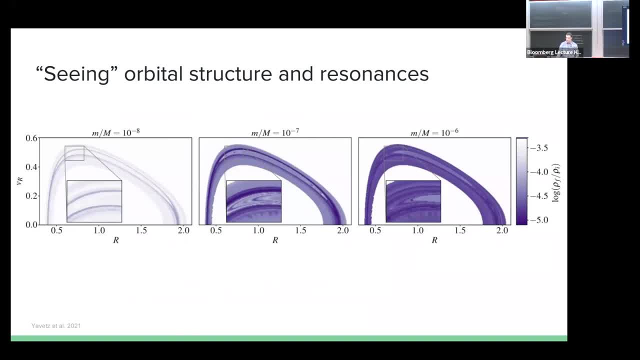 information to answer this, but I don't know yet. So when this happens, if you kind of share off into the second component to make sure it's dry, is there any prior on what the ratio of the number of stars in those two components are? 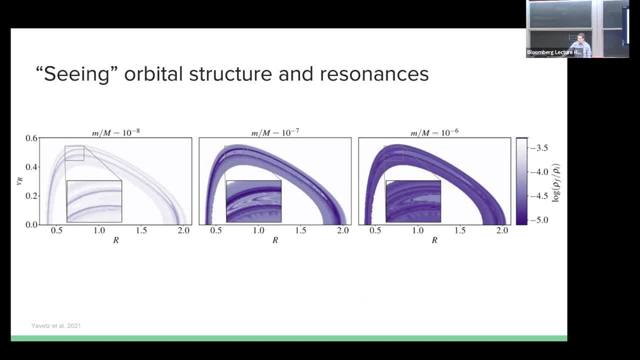 Or is it just? I will address that as well. But the general idea that I have- and having studied this a bit, but perhaps not enough- is that it's purely just the size of the resonance with respect to the size of your progenitor. 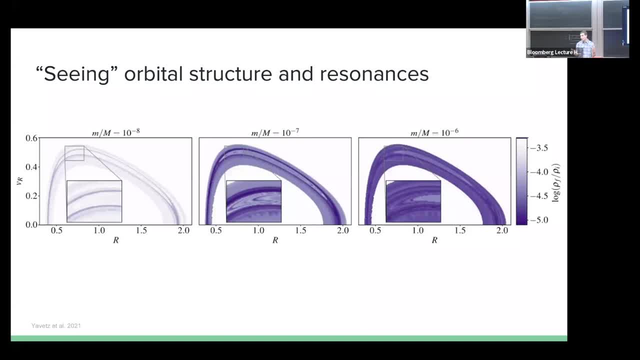 In most of the cases I look at, the progenitor is well, much bigger than the subgenitor. It's smaller than the separatrix, which is about the boundary, but it's usually smaller than the resonance itself. for the reason I just gave Chris, which is I don't want them to wash out. 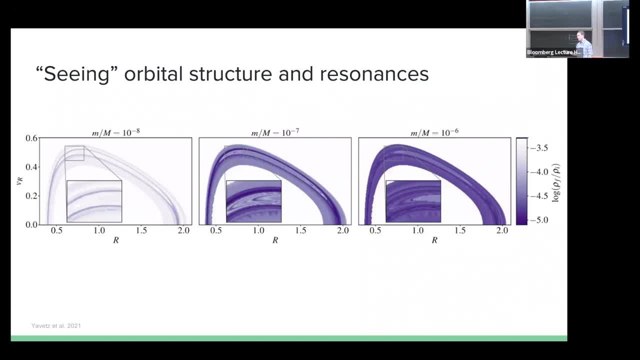 the entire structure, And so then it's just statistically: where does the separatrix slice through it? so it's more or less 50-50 that they would be trapped or untrapped. Of course you have to get the resonance first. 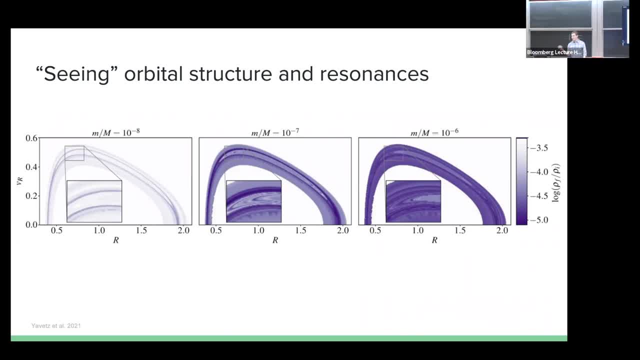 Most likely you are completely untrapped. But once you are at a separatrix, I don't think there's any reason to be biased towards trapped versus untrapped, assuming your progenitor is smaller than the original- Sorry- than the resonantly-trapped region. 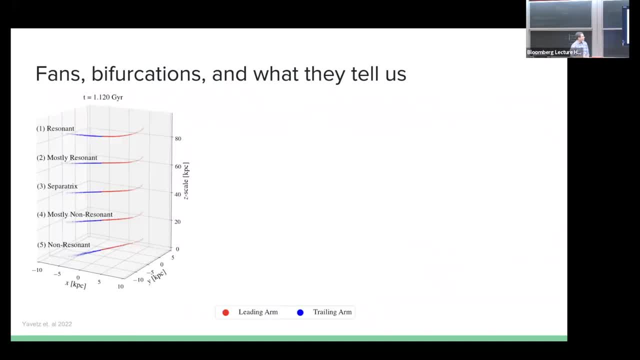 This Good, OK, so you saw a bifurcation. The more we study this, the more we see various different types of perturbations and well or morphologies you get, if you happen to evolve, an extra resonance. So here are five streams, all with relatively 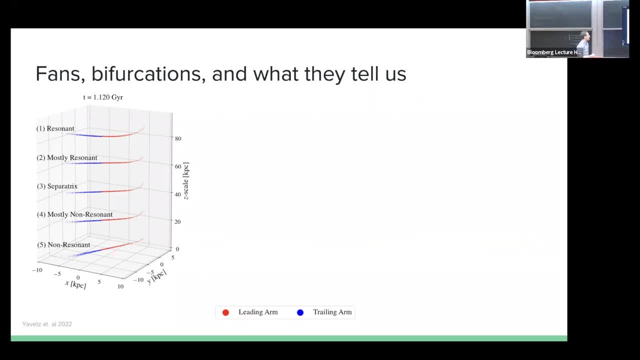 similar initial conditions. So, George, to your question, The difference between these streams is how many of the particles are trapped versus untrapped. So the top one is completely resonant, the bottom one is completely non-resonant, the middle one is half and half. 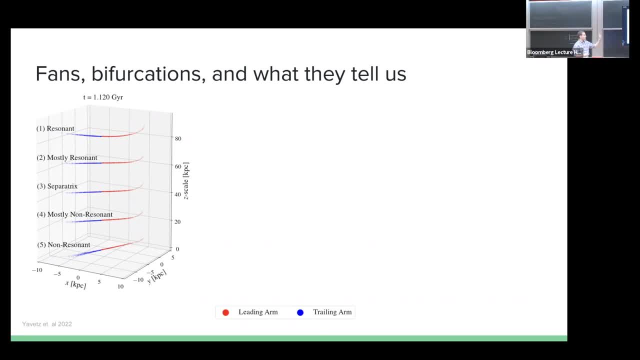 and then you got it. So far, they all look thin. This is again that first time. I paused in the other picture. Now, three of them, all three that have some component. that is a different component. one of their tidal tails has fanned out. 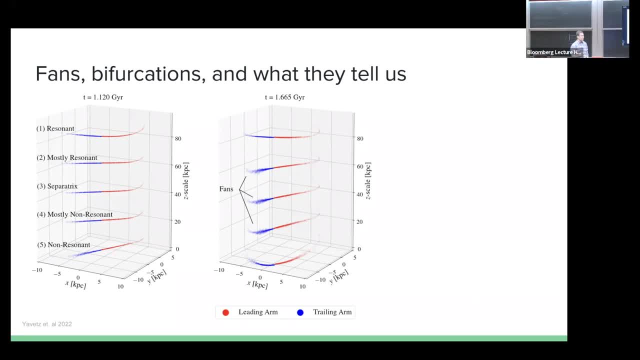 So the red tail still looks nice and thin. The blue tail seems to experience in all of them this kind of fanning out. So there's an asymmetry in terms of each of the tails, but there's a symmetry across the separatrix. so far. 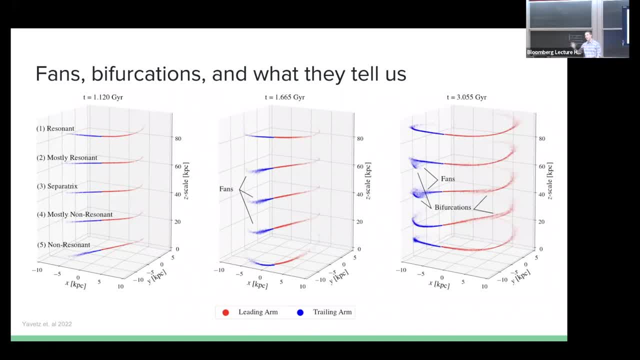 Take a snapshot ahead of this. so this is now three giga years in All sorts of asymmetry start popping up. So some of these now have bifurcations. So the component that fanned out coalesced into a thin component. 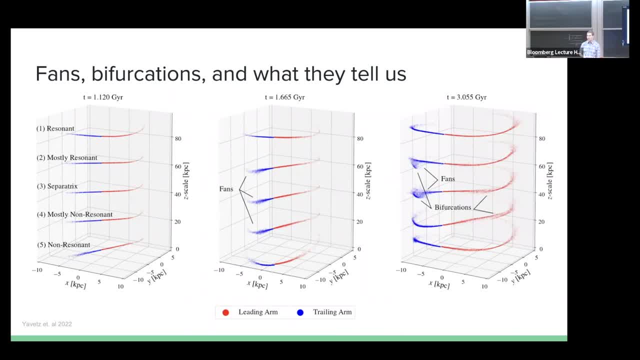 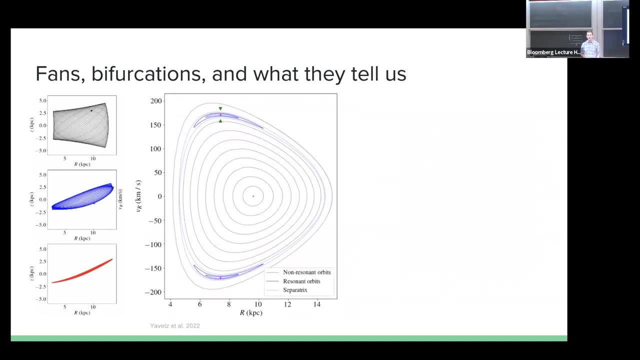 again. Some of them have features now in their leading arm, in the red arm. Some of them still maintain their fans. So OK, This is not clear as to why you get all these different kinds of morphologies in the streams. We think we've understood this relatively well just based. 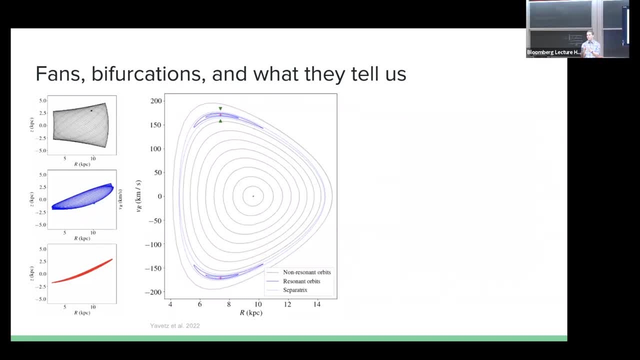 on the resonant dynamics. A lot of this has to do not just with straddling separatrix, but what is actually your evolution? essentially your slow frequency with which you evolve in this plot. What is your pendulum frequency? It is asymmetric. about the separatrix: 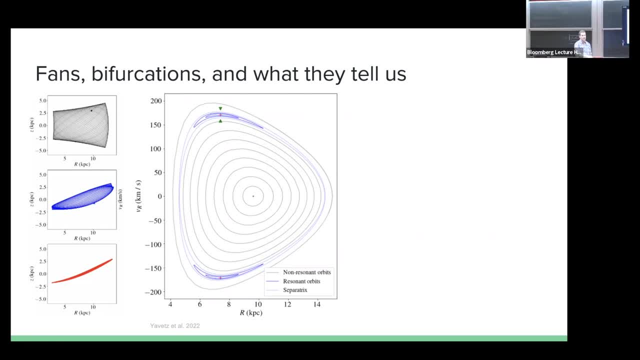 And it diverges as you get to the separatrix. So your pendulum that is exactly at the unstable balance point never reaches the top, So that has an infinite period or a zero frequency, And so around that you get this very sharp behavior. 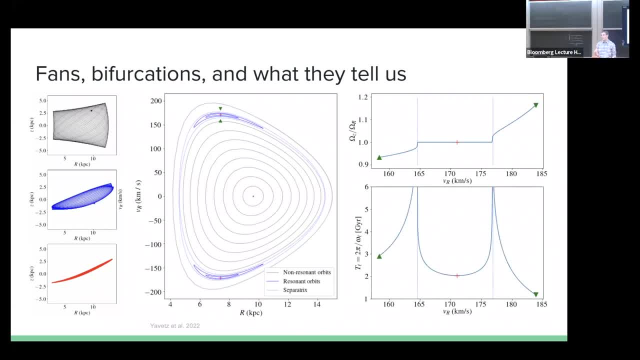 We plot this in the bottom plot is the liberation period. The middle region is the resonant trapped region. So you've got kind of some oscillation period in the middle which is your harmonic oscillator. Then you move out to where it's no longer harmonic oscillator. 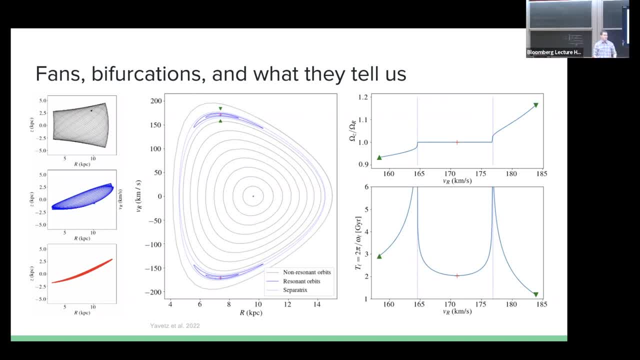 And you diverge, Your period diverges to a and you regularize back down. But if you are near this, one of these vertical lines which are the separatrices, if you're near that, then your particles are spread around and have a very large gradient frequency. 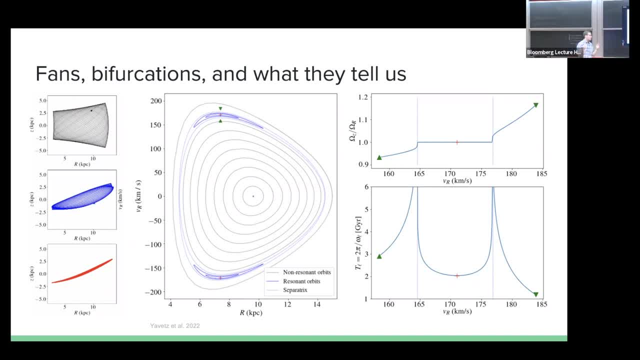 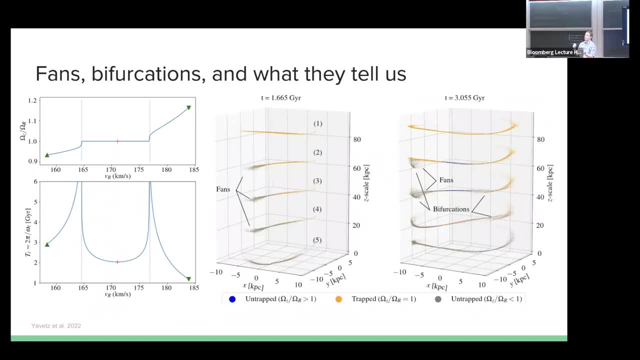 So that can induce additional changes in how you expect that phase mixing to happen. And so we've then gone and shown how these various components. you can understand them either, as in this case, I'm just showing what's trapped and what's untrapped. 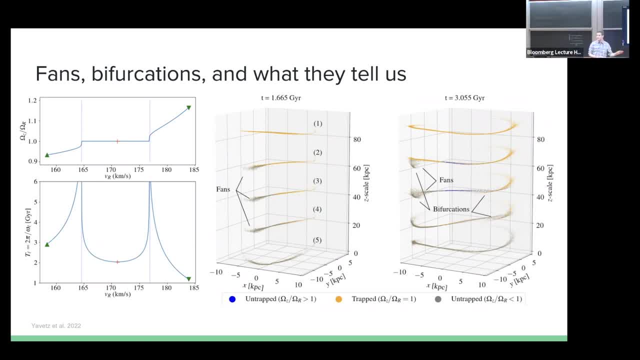 That's Short question earlier And you can explain the bifurcations very nicely. So we have a clean component and a clean component. That means one of them is resonant, one of them is not resonant. So one of them is trapped, one of them is untrapped. 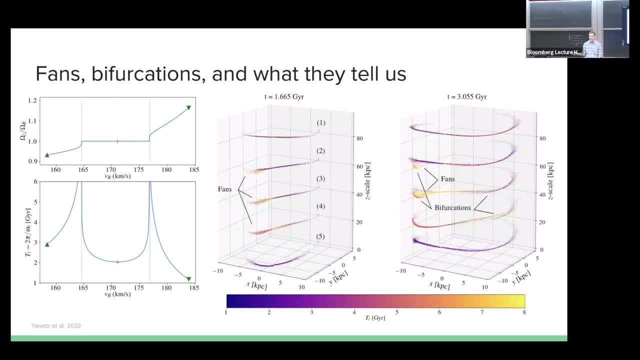 Whereas if you have fans, this is usually explainable based on this liberation period gradient. So you can understand the fanned out regions And, in fact, to get a fanned out region, you don't even need to be at all straddling the separatrix. 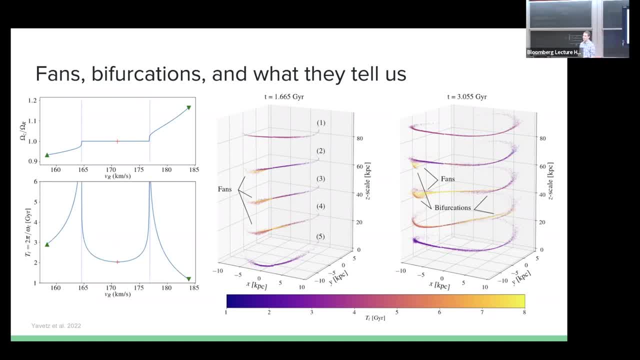 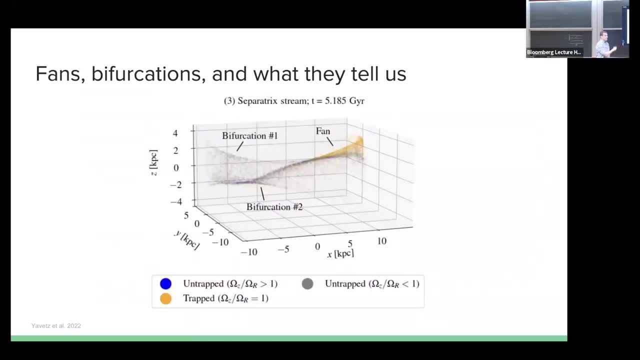 You just need to be close enough to experience this high gradient in your resonant frequency. Just another fun thing which happened because Chris mentioned this to me a year ago And I was like, well, we should try this If you happen to evolve a few times in this diagram. 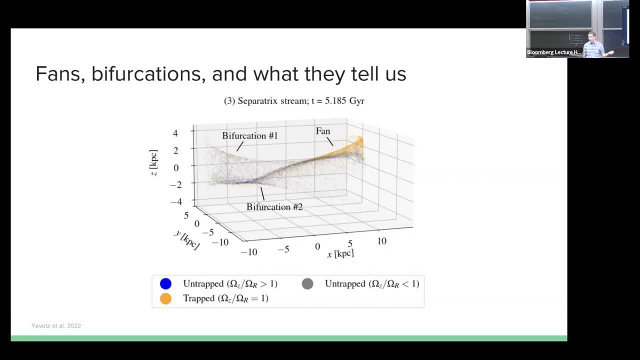 if you hit the unstable balance point more than once, you will pull off additional arms, So you can actually get strings with multiple bifurcations this way. More importantly, I would argue, this means that even if the thing is evolved for long enough, 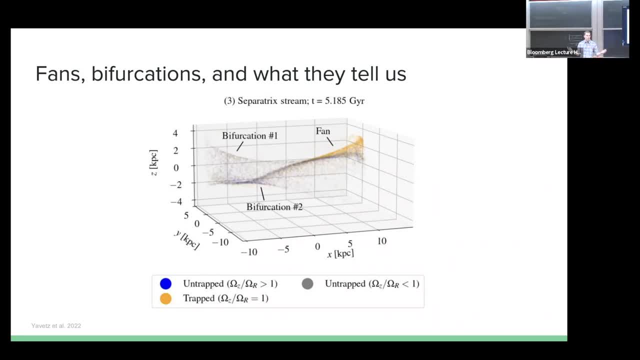 for one of these bifurcations to have blurred away into the background. it's too diffuse to actually see. as long as you evolved again past the unstable balance point, you'll pull off a new one. So if you happen to be near a separatrix, near resonance, 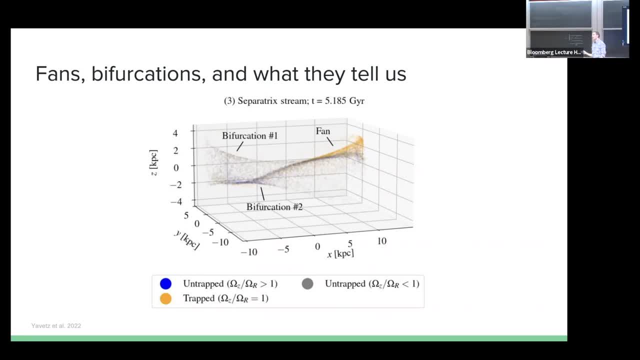 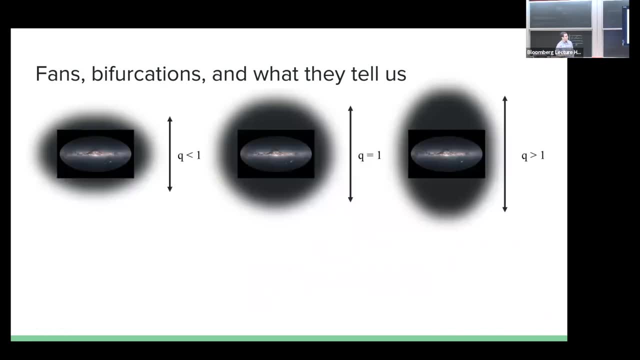 and you're evolving there, then as long as you have encountered an unstable balance point relatively recently in your history, there should be something observable in terms of your morphology. So to Shang-Chi's question. So have we tried this on the catalog of streams? 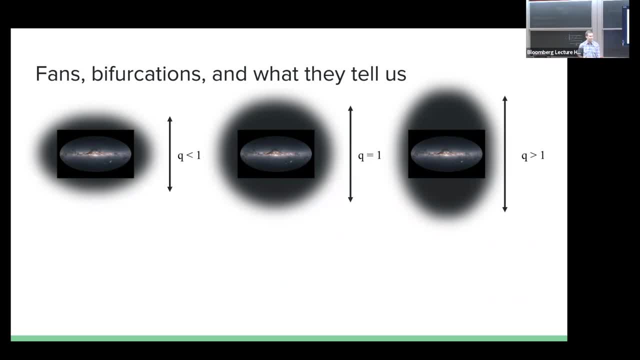 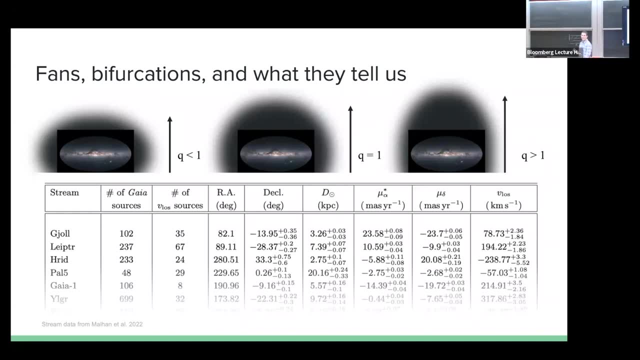 These 100 streams where do they fall in the spectrum? And so we've started this, And so we took a subset of streams. I filtered here for streams that I thought were particularly likely to be helpful. These are streams that are relatively close in. 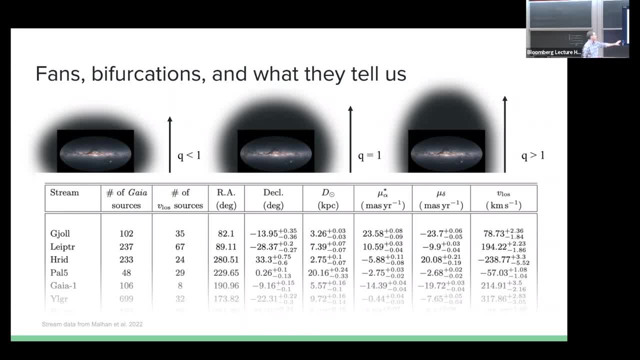 so they forwarded many times. This is from a larger catalog. I chose only 12 streams from this catalog. You'll notice that some of these streams have very few members, So 100 strings, This is 48, 233.. This is not like statistically large samples. 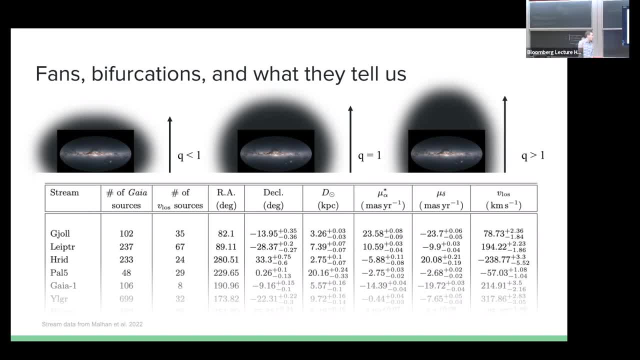 like we have for Sagittarius, for example, to actually say we see the full thing. If we have 100 particles and I say that 10% of the stream has been resonantly trapped, I'm not going to say I see 10 stars and make a claim based on that. 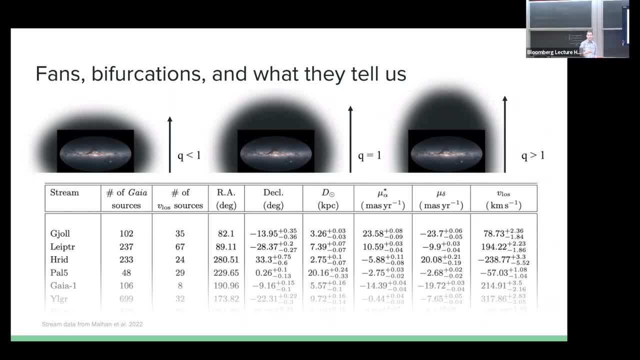 But to your question, the orbits of the streams. we more or less know what they are. What is the likelihood of one of these orbits being near a resonance in a reasonable configuration of the galaxy? So we take these 12 streams that we've filtered from this data. 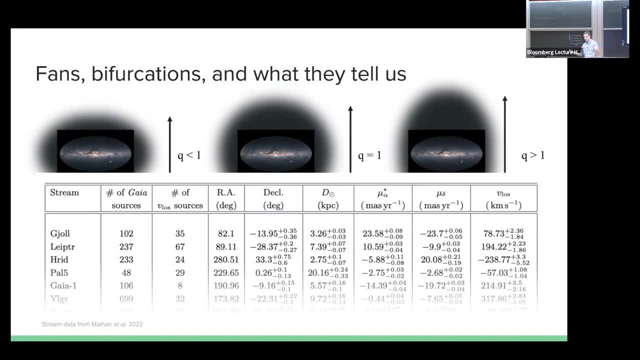 set And we look at and we know what their positions are in 60 phase space, So we can assume what their progenitor orbit is, more or less, And then we take those orbits. sorry, those 60 phase space information, not orbits. 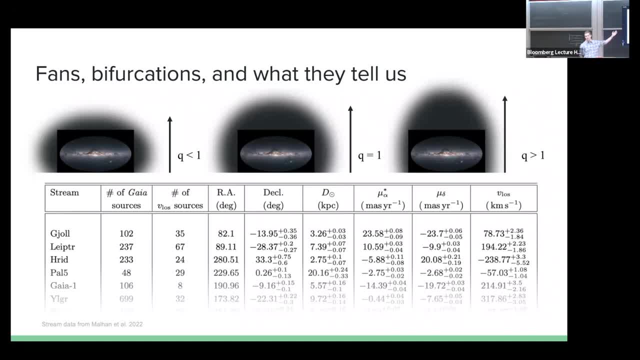 and we put them into a potential ranging from oblate on the left to oblate all the way on the right. We're just taking the halo and starting from a squashed halo and extending it And each one of those, this array of halos, we're looking. 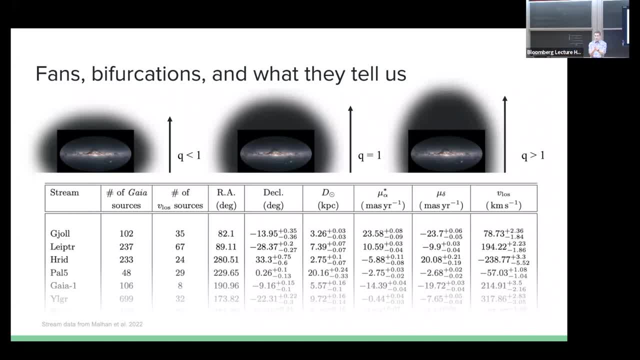 do any of these streams fall nearer, So the stream position- sorry, the location of the progenitor now- is not changing. What's changing is the potential And therefore the resonances are kind of sweeping through as we change the shape of our potential. 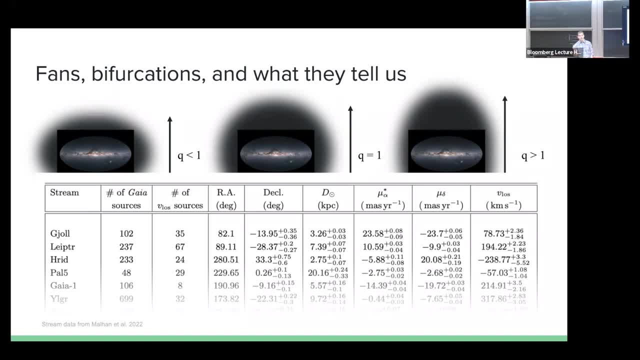 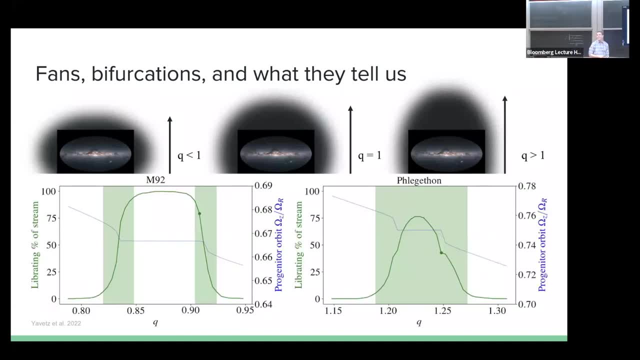 And we ask: do we see any of these streams fall near and kind of what I say prose this resonance structure? And we do, excitingly, Otherwise I maybe wouldn't be giving this talk. So for two of these, two out of 12,, 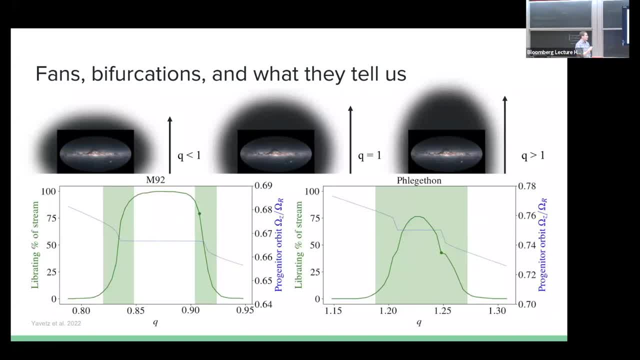 which is not insignificant subset. we see them fall near one of them. So I all I look for just three resonances here, just the one to one, the two to three and the three to four. so various low order frequency ratios. 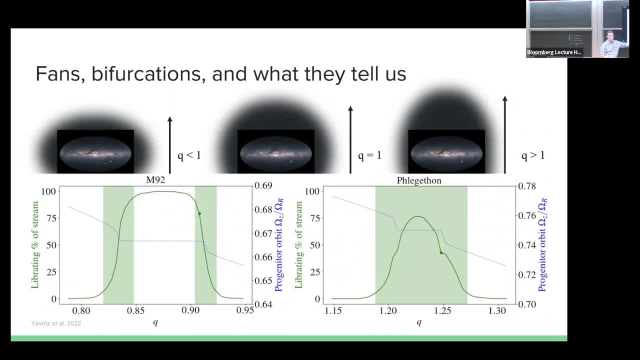 The important thing in these plots. the green line shows you the percentage of vibrating stars in the stream, assuming it's progenitor orbit. So, George, to your question, how many of these particles are in the resonant trap orbit family? So it goes from zero outside the resonant trap. 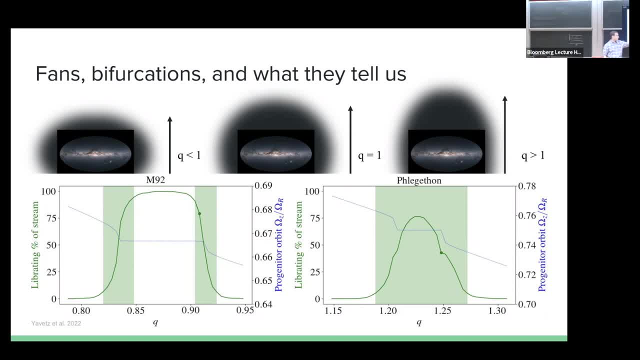 Resonance to 100, in this case, in the middle of the resonance to zero. on the other side, Here's actually one that is about the size of the resonance, So it never quite reaches 100%. Is either the size is actually no, it's not the size. 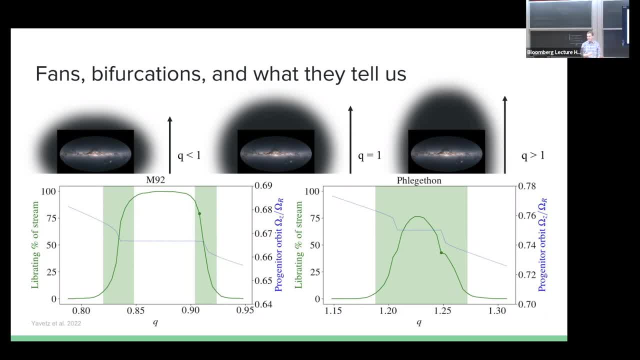 It's grazing the resonance, So it never actually is fully endorsed by the resonance, So that one reaches 75% at most of particles, And I highlight the regions where at least 5% of the particles belong to a second orbit family. So I would say 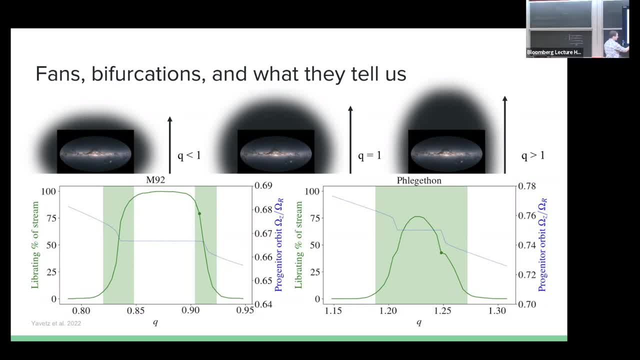 And If the potential is in any of these, squashing this parameter. so the q parameter is how? what is the ratio between the z-axis and the x or y-axis of these potentials, If the potential happens to be in any of the regions? 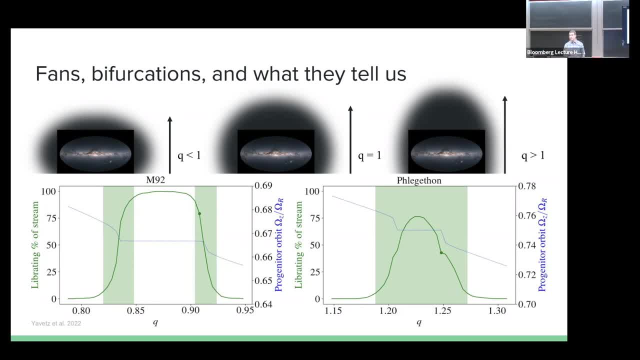 where the green area is highlighted. these streams would be sensitive to the existence of a resonance. Now, the two relatively small and not well studied streams- I'm not. their membership is certainly not enough to have found it. Nor have we looked to Chris's question. 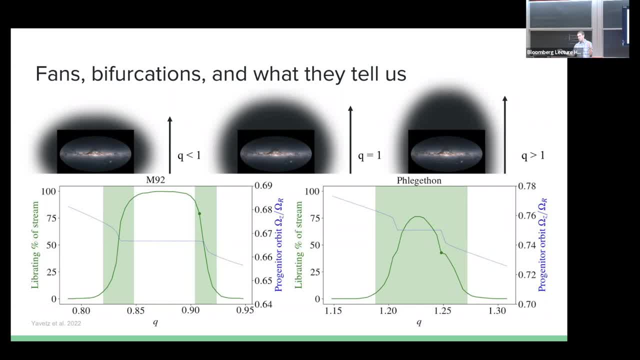 for companions that are further away. that would say, you know you really are on the other side. So this is one of the main things we want to do, which is say, OK, do this kind of search a little bit more robustly. 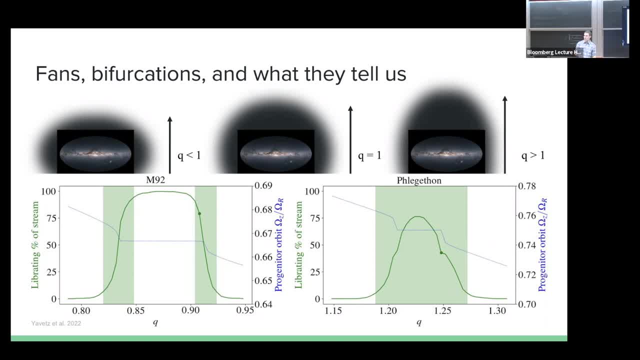 for a larger distribution of potential that you want to test. Find the candidate streams that are interesting, that might prove a reasonable subset of potential. So this one is actually particularly interesting because these ratios are what a lot of the other studies of streams have been pointing to in terms of the oblateness, the 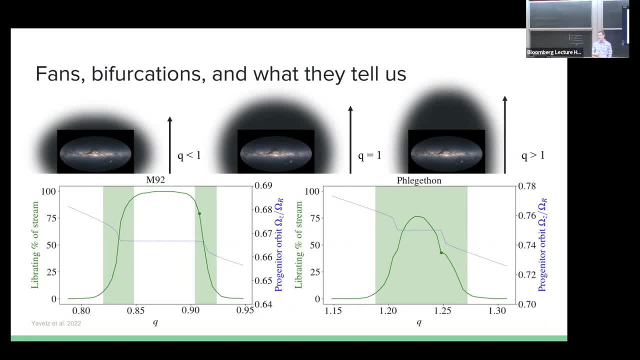 The usual range that's quoted now is between 0.7 and 0.9.. So in theory this one has a chance of actually catching something interesting. Perhaps less so for a phlegathon, which is at the pro-late end, which seems relatively ruled out. 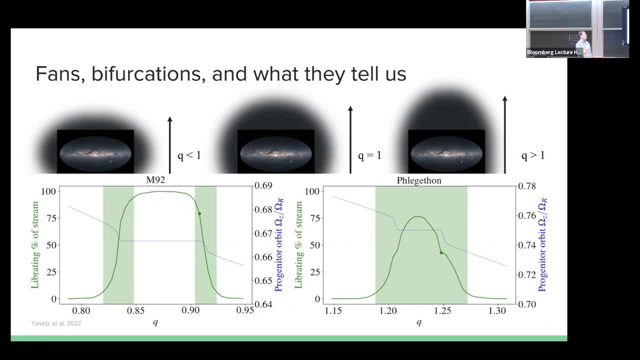 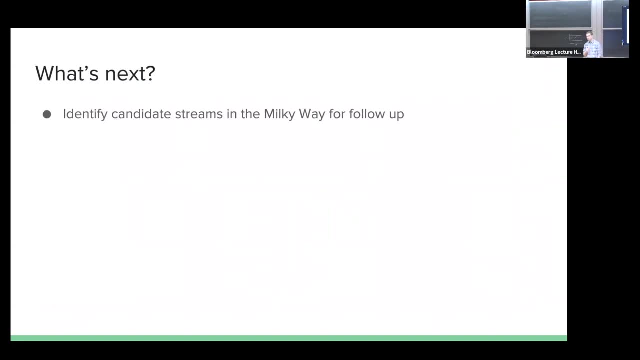 by some other studies. But either way, look for these streams or find the streams that would probe the right potentials and then do some observational follow up to look for components that are not following the expected stream track. So In this test, do you include those other misbehaved streams? 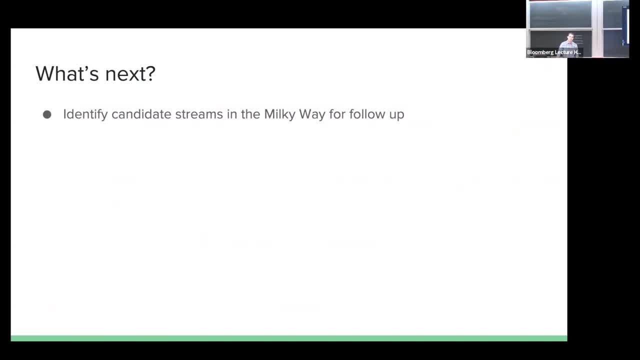 And so does that have. if so, does that mean that A few of them are there? So JLM is there, for example, which is one of the ones I really wanted to fit, does not fall in your resonance. Does that mean that it cannot be due to the resonance? 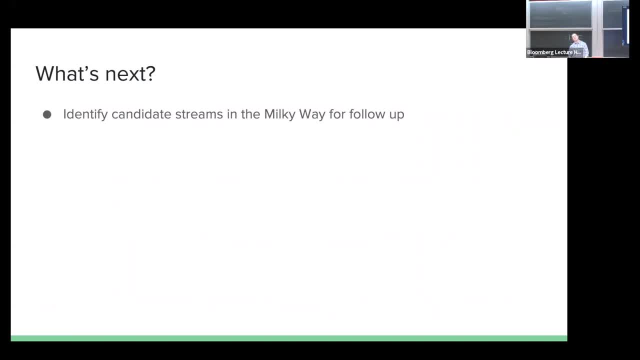 or is it because there's some other parameter space that If you're pessimistic, that's what you would say? If you're optimistic like me, maybe you'll say you haven't looked in the right potentials yet. I think likely. JLM is not. 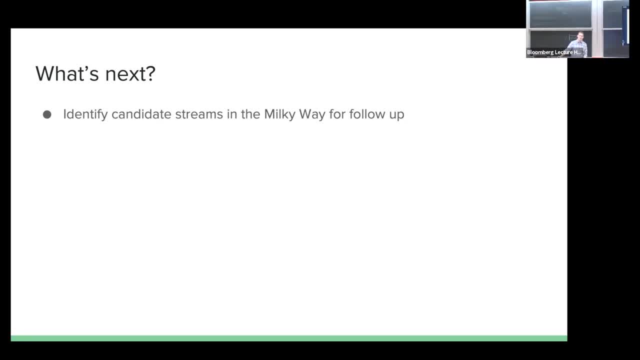 I'm certainly not going to keep looking at JLM, Because I've spent enough time trying to make it work And it's like shooting in the dark in this case. So I think better to decide based on the streams, which ones are the ones that are likely, rather than chase. 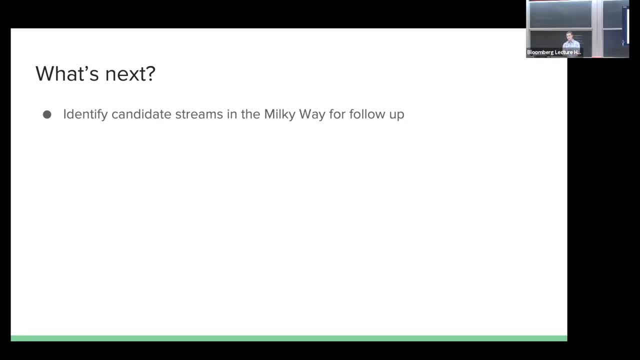 one in particular that has, Well, actually both approaches. I think you should chase the ones that do have known deviations from a stream like structure and see if it works, but to a certain extent. And besides that, I think this goes back to Chris's question. 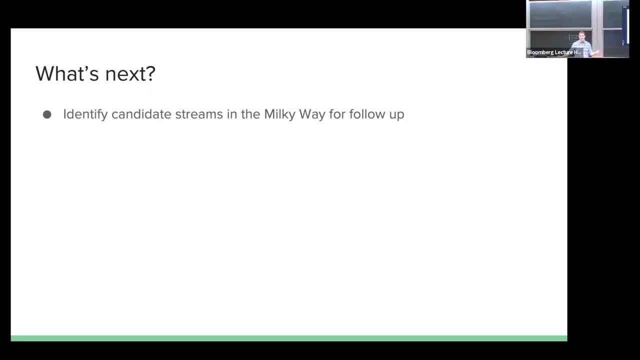 It's certainly likely that we haven't actually just we just haven't seen The component that is totally- I mean, we've only seen many of these misbehaving streams very recently because we have more and more data, because these are the streams that people have studied a lot. 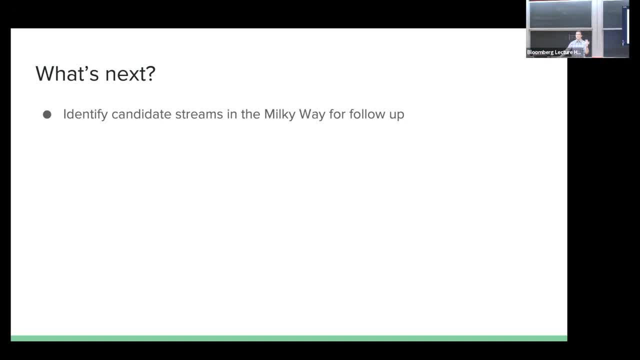 So GD1 is a very, very commonly studied stream, even before Gaia came out, because it's nice and thin and very easily observable and it's retrograde, So it brings out other interactions, And so WebGaia2 came out. I think Adrian plugged that in and had that plot. 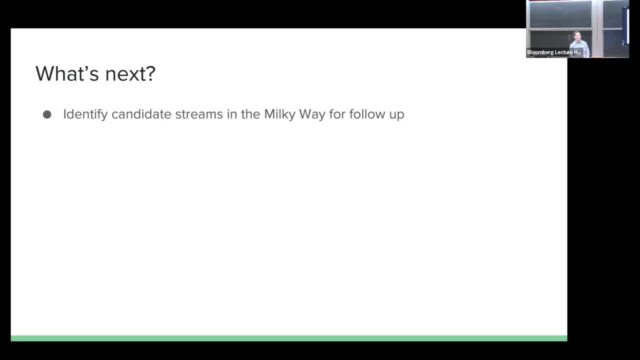 within a few hours because he knew that that's the stream he wanted to look at. A lot of these streams that I've picked out are very recently discovered streams Haven't had a lot of haven't seen a lot of love recently, So I haven't seen a lot of love at all because they're just new and small. 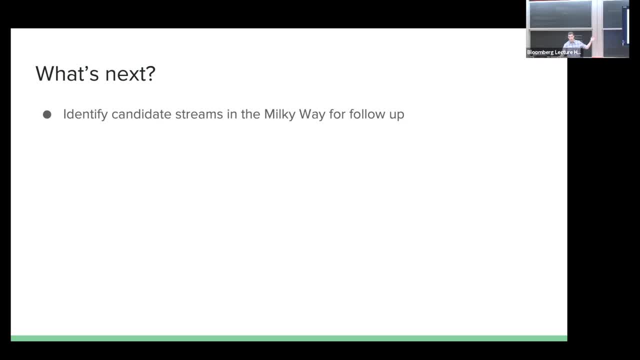 and nobody's thought to really pay much attention to them, where actually they might be very interesting because, again, the more streams we have, the more they probe the full picture of the surface of section that I showed earlier In about eight minutes Good. 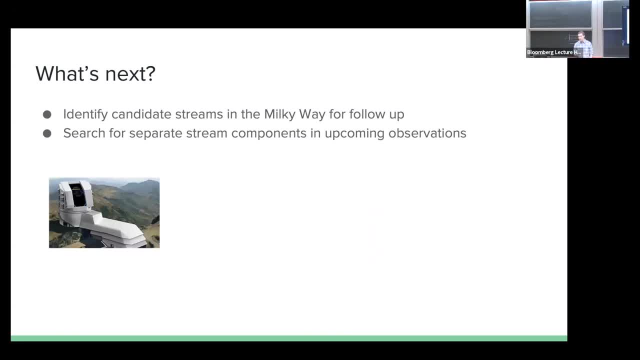 I don't need to say too much more, I'll just say so. two other things that are interesting here. There is more data to come which will help this, So LSST will complete a catalog of our Lyrae stars, in particular in the galaxy, which is a very good way. 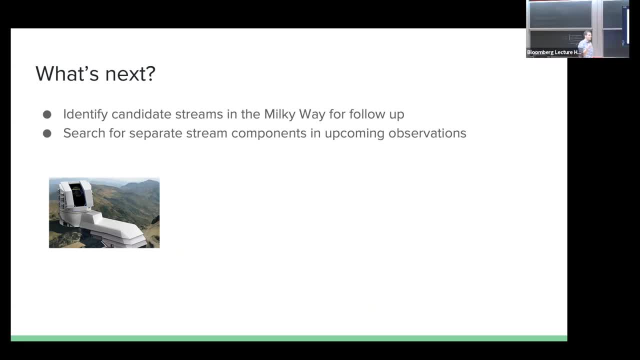 of finding streams. Our Lyrae stars are typically born in globular clusters, the ones in the halo, And so if you have a complete catalog of our Lyrae stars in our halo, you might easily say: OK, I see three Lyrae stars below the galactic plane that 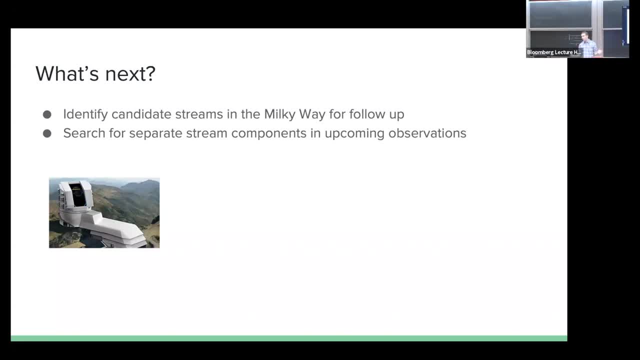 have very similar kinematics to a stream that is above the galactic plane. How could they get there? How would they be there if they weren't born in the same globular cluster? Very easy to ask. So a complete catalog of our Lyrae stars. 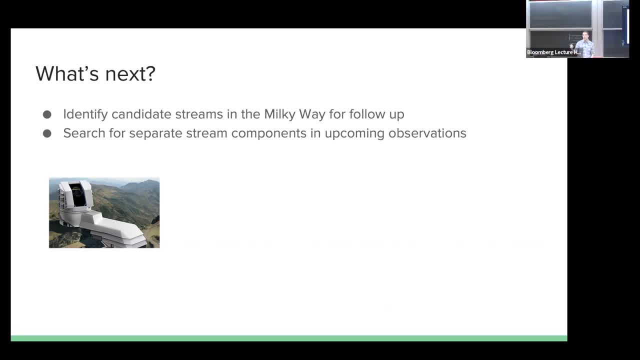 does help us complete this picture of are we seeing the other components of these streams, even if they've been pulled out or fanned out, but they still exist somewhere. In addition to LSST, we also have Roman. Both of these will start seeing streams in other galaxies. 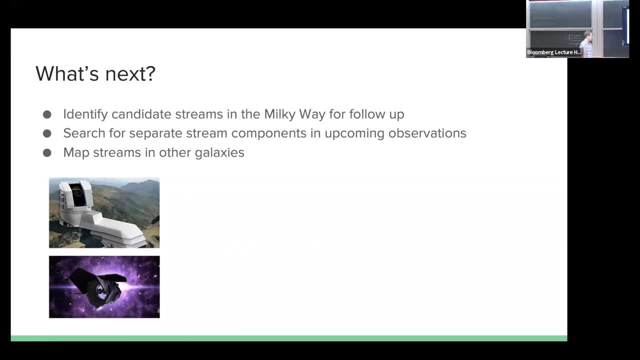 So LSST will see dwarf galaxy streams that are quite far away. OK, Roman will start seeing globular cluster streams, even in the global universe, The more streams we have. this effect is, among other things, a morphological effect, So you will see bifurcations pulled off. 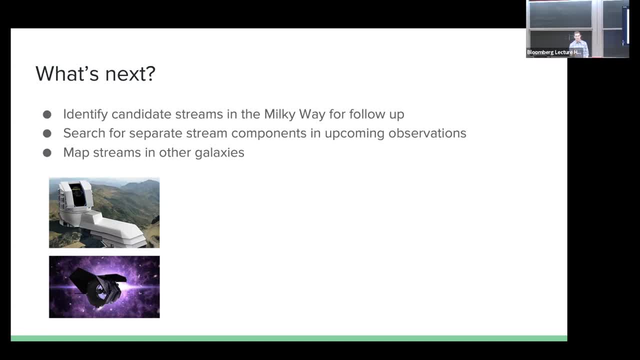 So if you have a huge catalog of streams, you might begin imagining that you can just start seeing these kinds of effects more frequently. You might even have some sort of a statistical measure. given potential shapes in general that we have from large scale simulations, How many streams do we expect to have encountered? 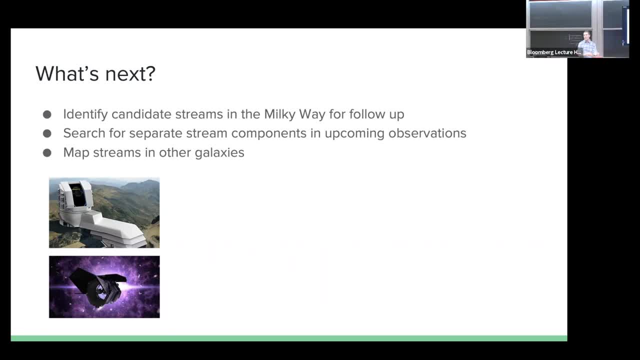 in resonance like this And you might say, well, we expect of 1,000 or 10,000 streams, we should see 10 or 20 that have experienced this. Why don't we see it in the data? or do we actually see it in the data? 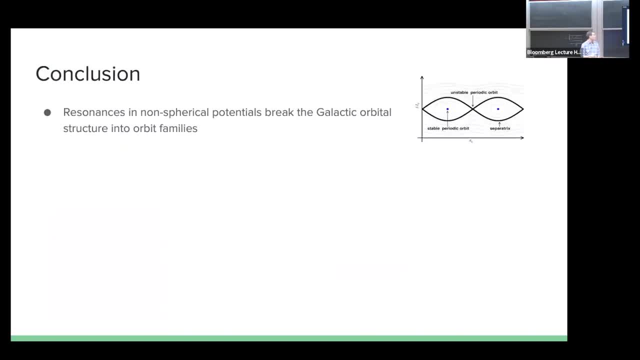 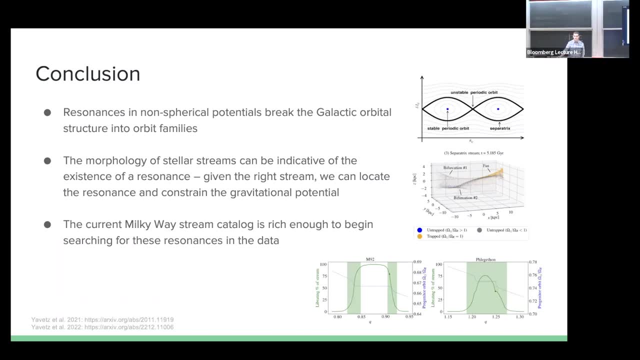 So yeah, just some thoughts of why this is going to work. So I'll talk about them and I'll just leave up my final slide. That's your question. Very nice question. Can I stop Time? dependence of the global potential is going to be unimportant if it's slow enough. 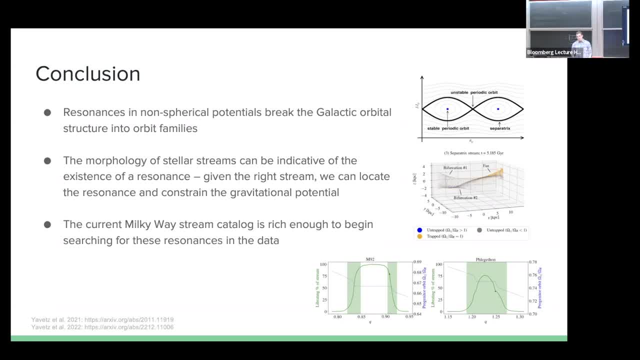 that your elaboration time is short compared to the global And given that the Milky Way hasn't undergone a major merger for eight giga years or something, is this pretty robust under changes in the Yes and no? I mean these resonances are relatively. 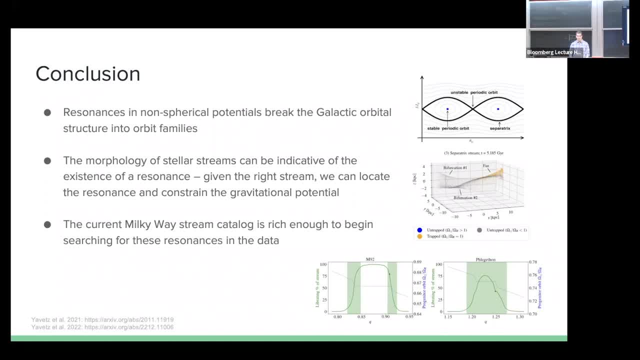 small and thin So it doesn't have to be a big perturbation to move the resonance around. So you have the LMC fall in and it's not necessarily what you think of as as close as we have to a major merger or even Sagittarius. 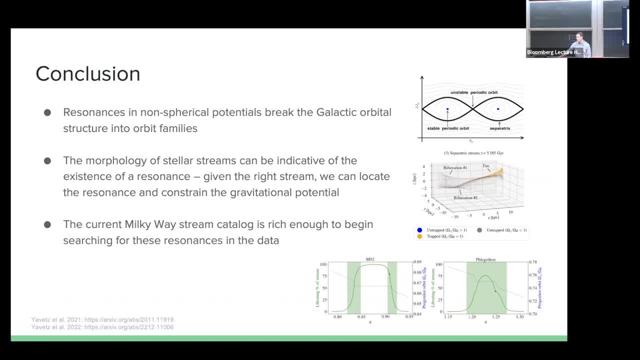 It's not really changing the global structure of the potential all the way in, but certainly it's certain radii. It is doing enough to move these resonances around and it is a very fast perturbation. So let the LMC fall in. 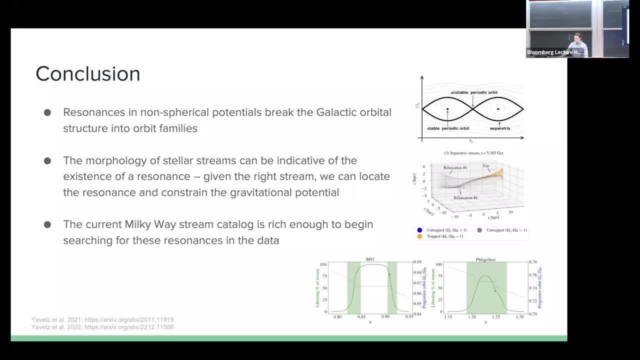 Does the red? Does your average resonance Shift by order of itself, as the location of that resonance shift by over the length of the resonance, much less or much larger? I don't know the answer exactly. Certainly not. It would be a question to figure out. 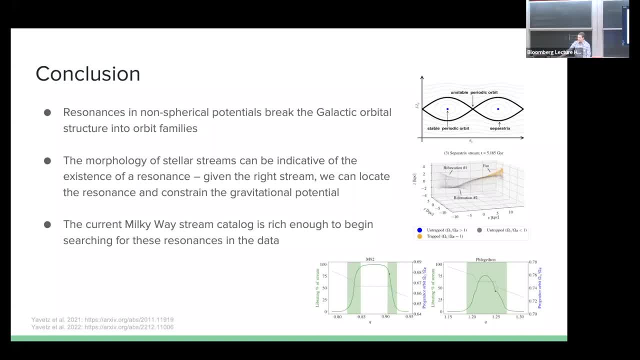 The main reason I have not looked at that question is because I mean it would be good to know. It doesn't actually change the effect as long as the resonance is still there. What changes? So let's say I see something and it experienced this effect. 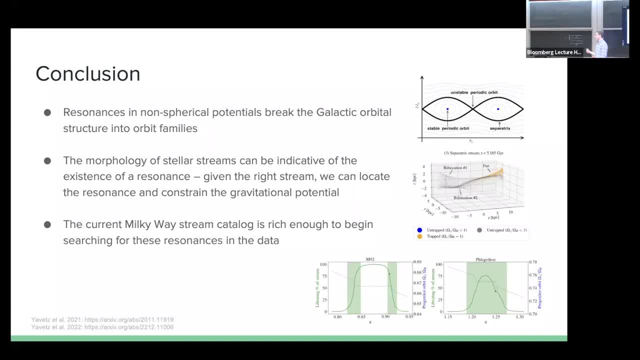 It hit the unstable balance point before Sagittarius moved the resonance away. What I'm constraining is the potential before Sagittarius did that. So it would be good to figure out what Sagittarius did, but at least figure out the location of a resonance. 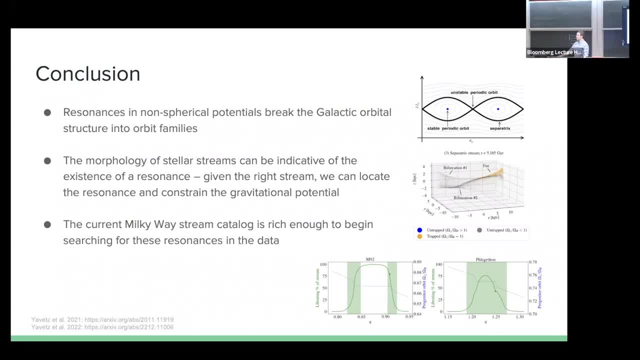 in a pre-Sagittarius encounter potential, which I think would also be interesting, I suppose if you think of an extreme case that something falls in and you just switch off the resonance because it actually goes So far away, And then everything will be blurred out by phase mixes. 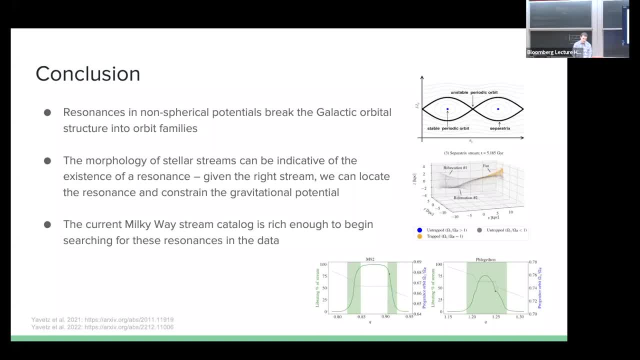 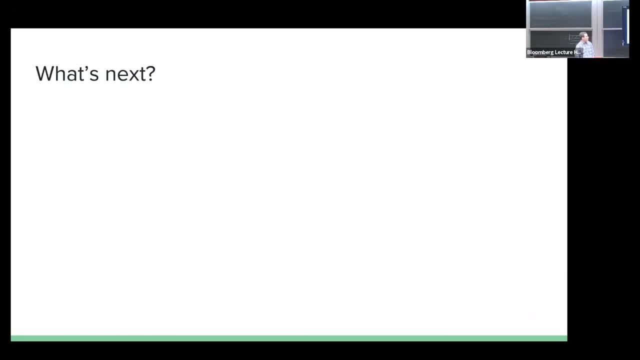 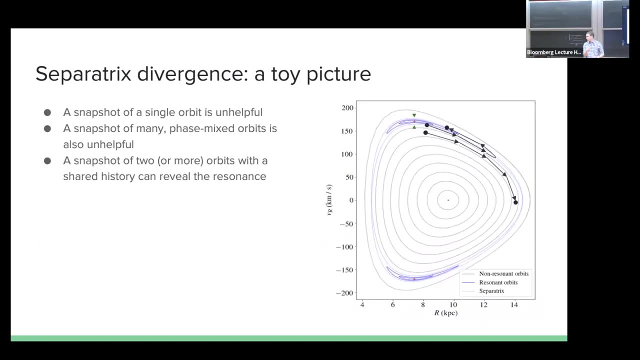 But I suppose the timescales are long for that, Eventually, But as long as you've done this. so if you have, where's my picture of the two orbits that go next to each other? As long as you've turned around, that's, I mean. 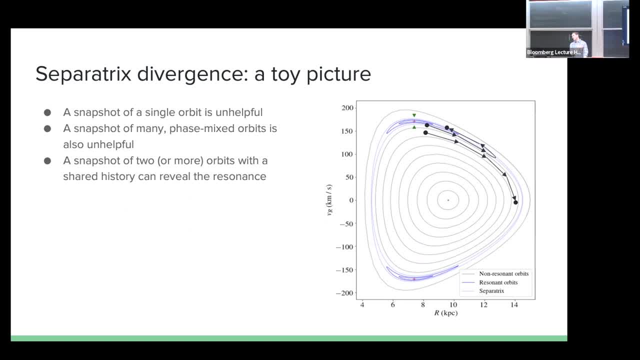 you only erase that once you phase mixed it up, which will happen even if the potential doesn't change. So if you do this And then you erase the resonance, what's done is done. This stream has been fanned out. You're going to have a component. that's always 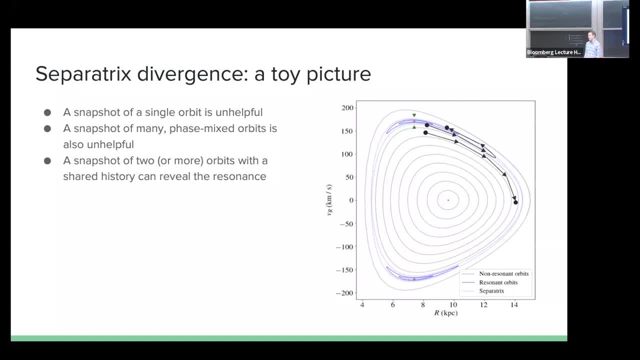 on a different or a different seeming orbit than the rest of the stream. It might look like it's on a very different phase. It might look like you've got two streams that have a very similar- or they have very similar- orbit of parameters. If this resonance is thin enough- the delta J in this case. 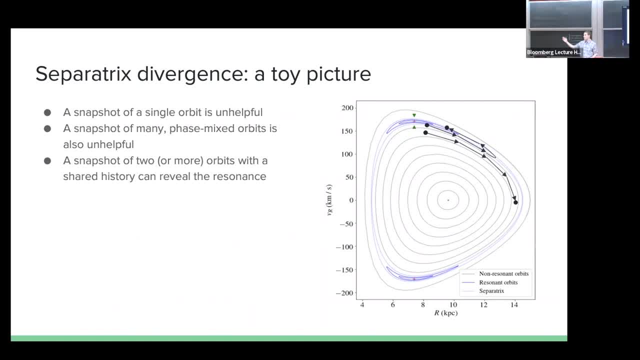 would be very small, but they'll be in a very, very different phase, So you might think they're just two streams that were born in three different phases on the same orbit, or if you were, however, you would model it this way: 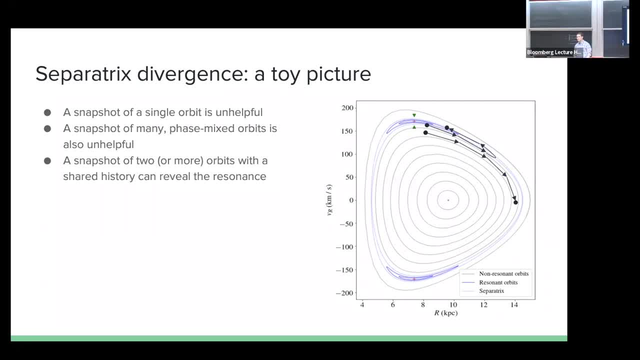 You'd figure out there was a resonance there. I have a naive question. So you've convinced me of the importance of considering resonances and so on. But if we were just to go back to the pre-Saturn rings picture, I can imagine modeling potential. as some kind of smooth component, maybe with some random field on top of it, and then just seeing what different statistical realizations of that. But I'm curious: what's the difference between the two in terms of the distribution of space? Is that just impossible to do because of the number? 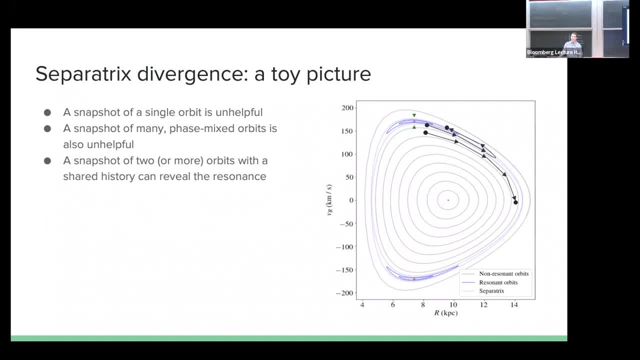 of degrees of freedom? Yes, and how much orbit integration you'd have to do to get there? Yeah, it is. I mean, in theory. all of this is garbage. All you want to do is look at a stream. You just have a bunch of stars. 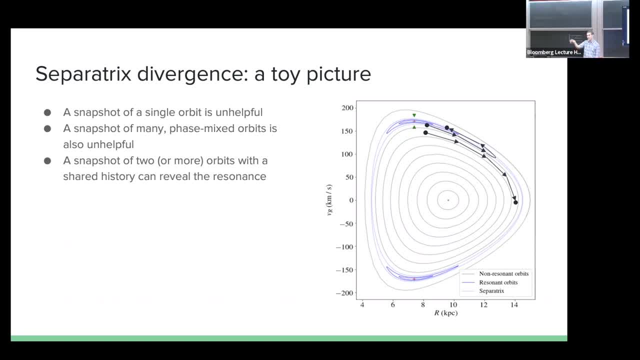 Just rewind their orbits and find the right potential, such that they all coalesce to the tidal radius and the escape velocity of the globular cluster that you think they were born in. And you can do that for more than eight or nine stars. It's just a computationally intractable problem. 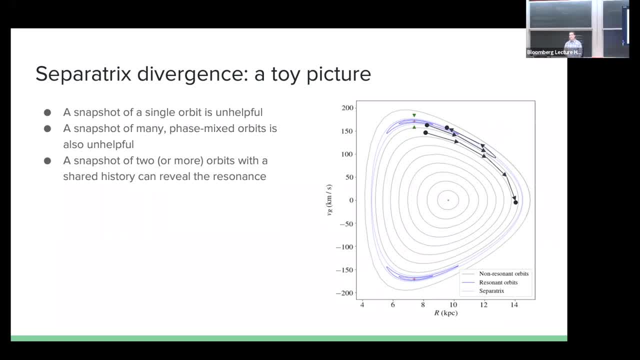 even for one stream, let alone doing it for multiple streams. The problem is here: you've got many degrees of freedom in terms of your observed data, the assumptions you make about what is the size of the progenitor, what is the time that things were leaked from the progenitor, 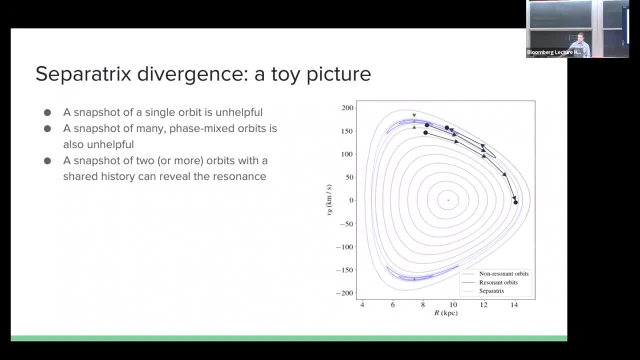 and then, of course, the potential space that you're investigating. But there aren't attractors. And again, you can imagine constructing a whole bunch of statistical realizations and so there aren't. Not that I'm aware of It would be. certainly people have worked on it. 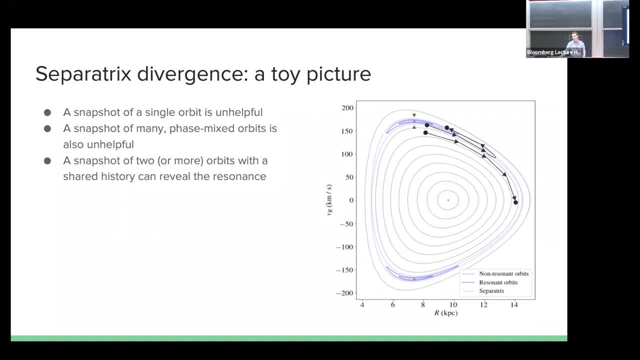 and are working on it, getting better, And there are various computational techniques that are improving this considerably. One of the main ways you do this is by computing gradients efficiently, because then you get kind of an orbit and an orbit integrator, And that has improved a lot in the last five, 10 years. 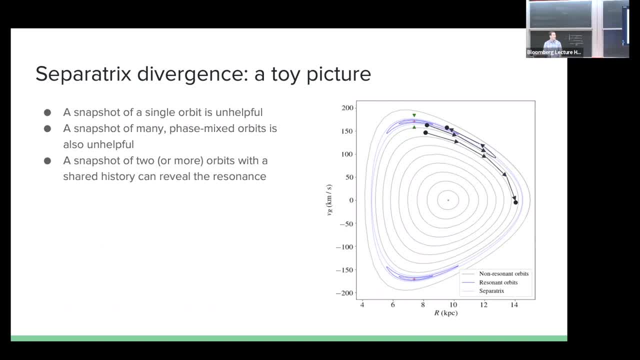 And so these things are happening, But certainly right now we need. we end up always using some dumbed-down projection- for lack of a better word- of the stream to try to fit it. So it's usually a generative model where you say: OK. 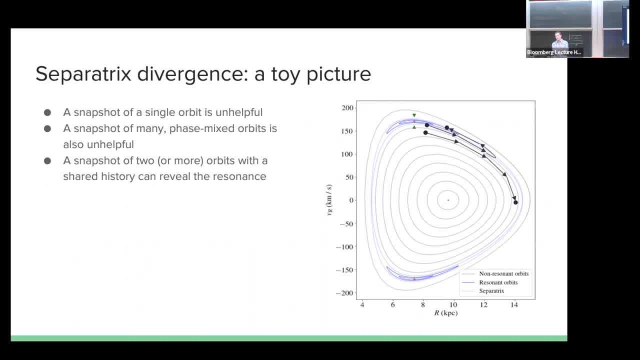 I'm going to figure out what the actions of my progenitor are. I'm going to use action angle formalism to project forward and draw from that distribution and see if I can fit. the stream is, for example, one way that that's done. 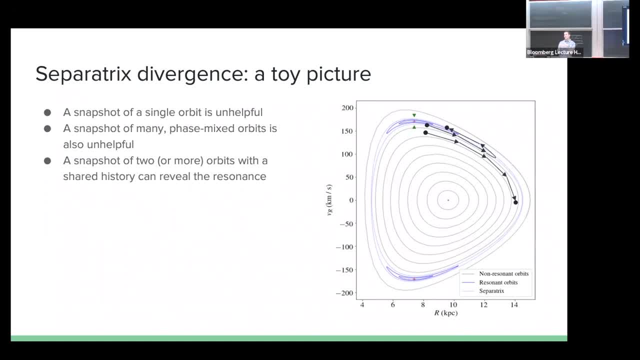 You do this in action space, where you try to get the actions to focus that are going to make the assumptions about actions and what the original configuration in action space was. So all these usually involve some projection of the data, choosing it in a wise way. 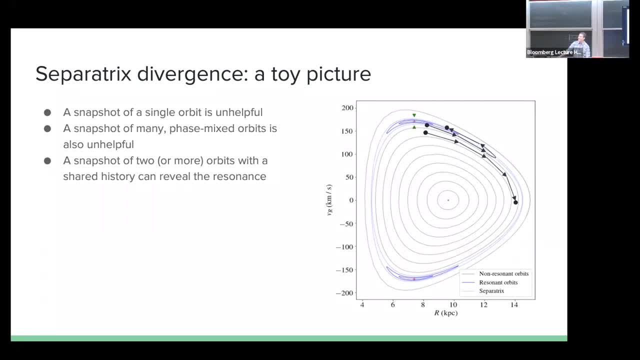 Chris and I are talking about another one that has been done writing off. But there are various ways to do this, that kind of circumvent the computational problem, but they always involve lowering the information. You didn't say much about clumpy dark matter. 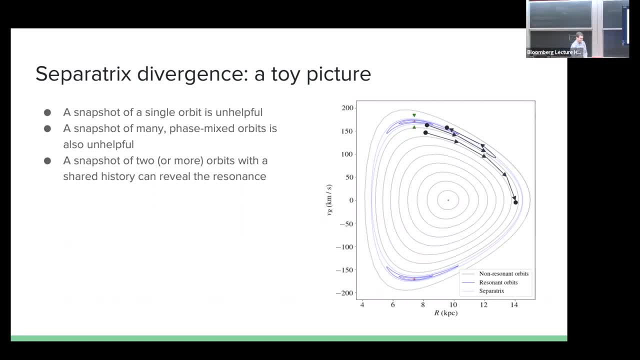 So does that mean that residences seem to explain the structures we see, or do we still think that clumpy dark matter, if it's a small sub-halo type that you would expect that a stream would have? I think that's a good question. 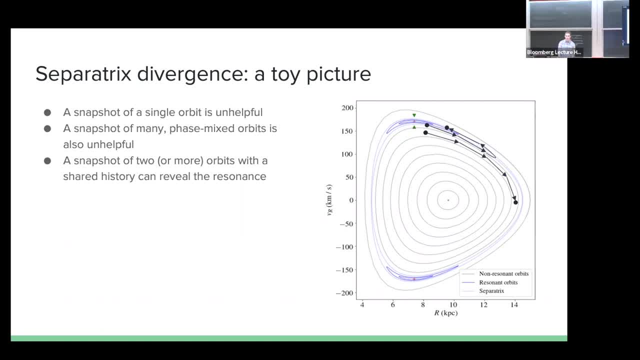 No, I think it's very different. It's a good question And I think it's so when Adrian was working on this paper on G1,. the right theory may be a sub-halo punch, a dark matter with a sub-halo punch. 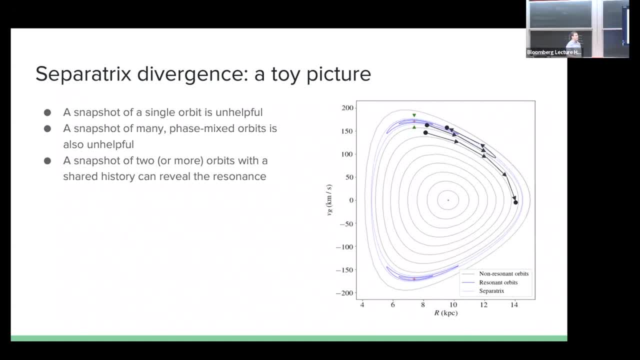 through the stream, which would be very exciting if it were. He asked me: can you do the same thing with this? The answer is no. It's very challenging to do that kind of local, So clumpy, dark matter, in particular if it's. 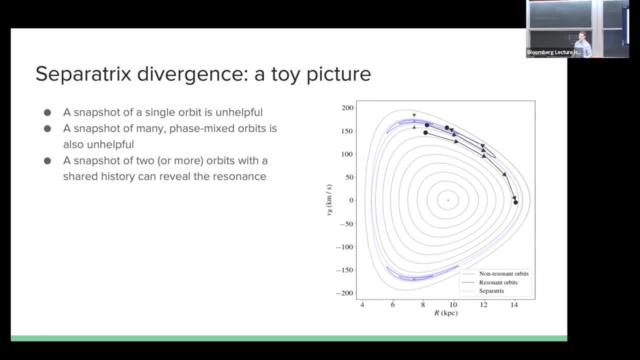 going to counter, not like a dwarf galaxy-sized sub-halo which has a very different effect. It's a very local effect. It kind of disturbs a very specific portion of the stream. It pulls off a spur, as you maybe saw in that picture. 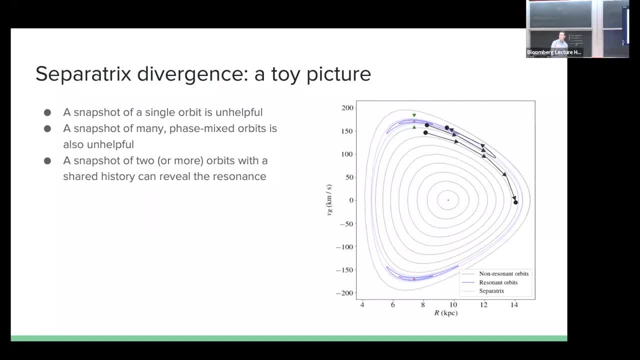 That spur is not in orbit. That spur is a time That spur will phase, mix away very quickly. It's just a local, it's a chance alignment of the stars as they're being pulled away from the rest of the stream. The bifurcations that I show here, 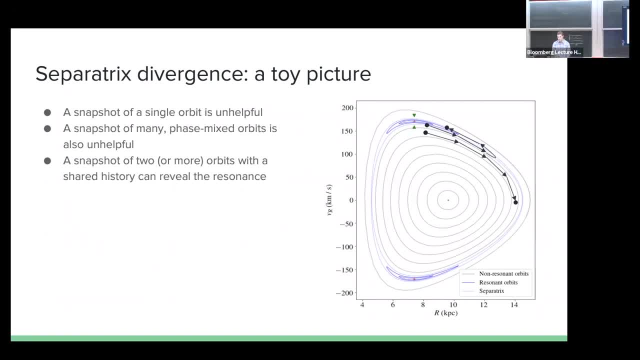 are actually all well-modeled, The orbits in any potential you choose. you might not model them as a resonant orbit. They are all kind of these multi-phase mix away. They will stay coherent streams. in the simulation I showed you, You actually saw two red streams evolving next to each other. 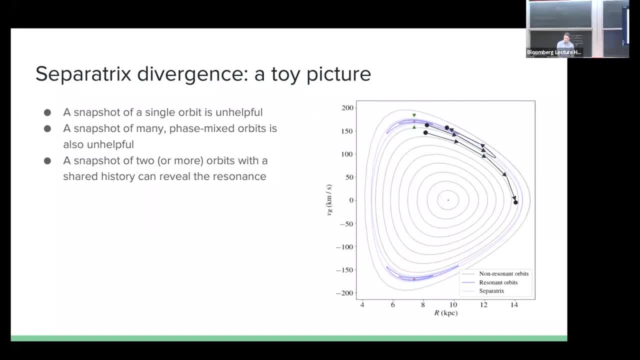 So they're actually very nice to differentiate between substructure in this case and this global potential. It's harder to do when you're talking about big sub-halo that kind of plows through and splits the stream off, because then you can actually get a perturbation that.